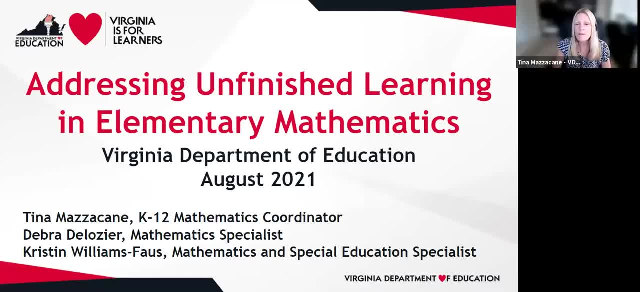 Today. my name is Tina Mazzucane. I'm the K-12 Mathematics Coordinator at the Virginia Department of Education. We are happy to have you here for our Addressing Unfinished Learning in Elementary Mathematics webinar. It is part of a series- a fall series- of webinars that the Virginia Department of Education will be sponsoring. 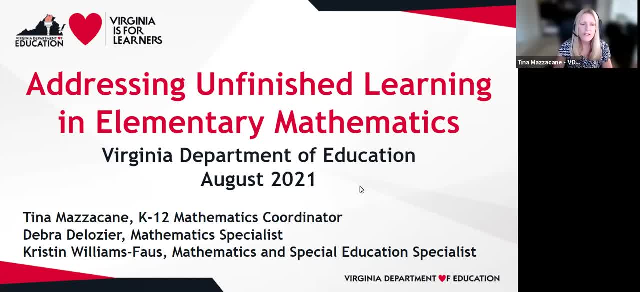 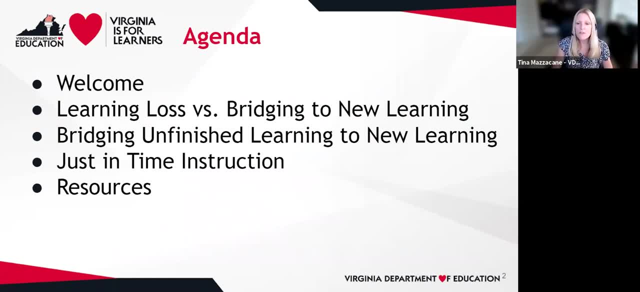 So this is the first in that series and we're happy to have you here today. So, as we get started, we would love to have your cameras on, but we want you to be comfortable, so please do what makes you most comfortable as you join us today. 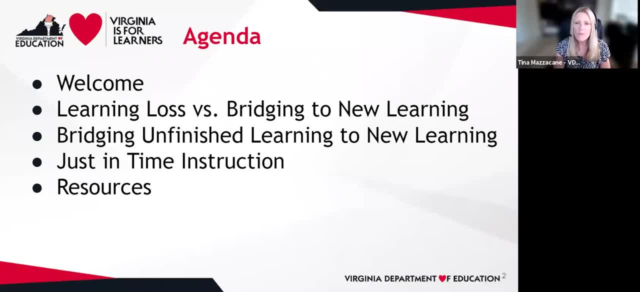 We will be utilizing the chat feature in the Zoom platform, so please check the chat. We'll be sharing different links and such as we go through the presentation At any point. if you have any questions, please post them in the chat. We will stop and certainly answer questions as we go. 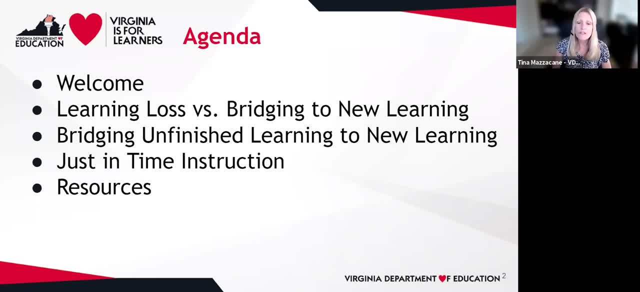 And we'll have some time at the end to answer your questions as well. So today we're going to do a little bit about learning loss versus bridging to new learning. So what does it mean to actually bridge to new learning? And then we'll talk a little bit about how we bridge from unfinished learning to new learning and some of those ideas. 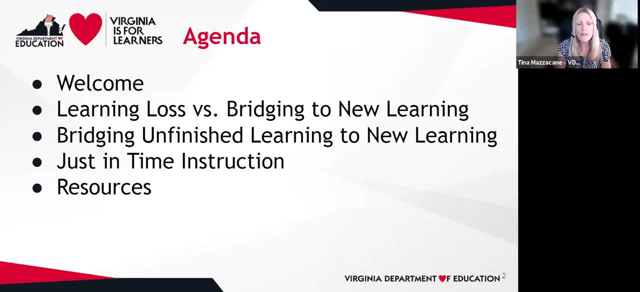 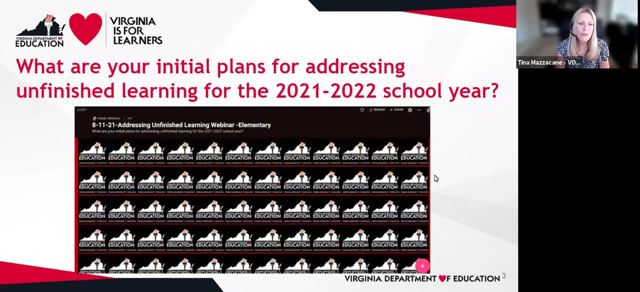 We'll talk a little bit about just-in-time instruction and what we mean by that, And then we'll follow up with some resources that we'll be sharing with you today, And we'll be doing that probably all the way throughout. but there'll be quite a few different resources that we'll be presenting to you today and hopefully they'll be of help to you as you plan for the upcoming school year. 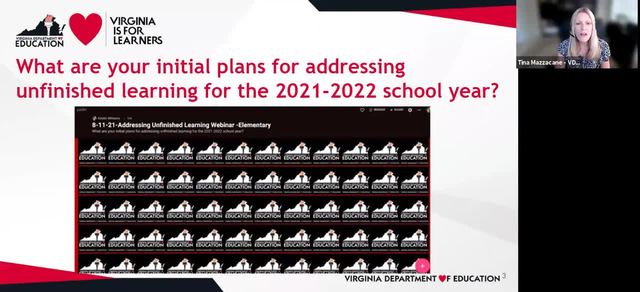 So we know that this is on your mind, as it has been certainly on ours- is: how are we going to address some of the unfinished learning that we know students are going to be coming to us this coming school year having either not experienced to the full extent some of the learning that we hoped they would have experienced? 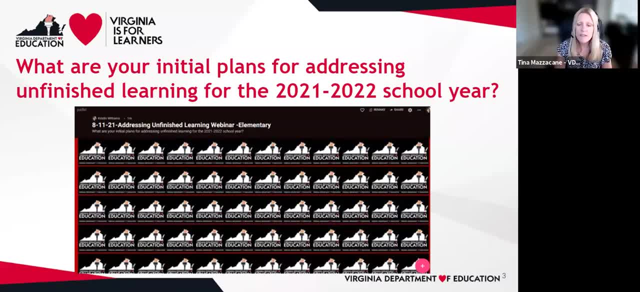 that previous school year that we know they're going to need for math in this upcoming year, or even just content that the teacher last year just did not get to, just because of the pandemic and the situation some of our school divisions have been in in terms of virtual learning or hybrid learning. So, Kristen, as I'm going to share in the chat a link to a Padlet, and this is a platform that you can use to easily- 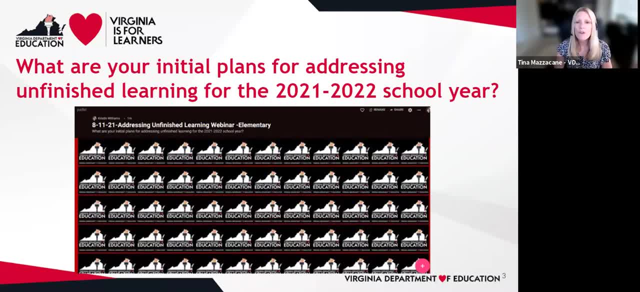 click in there and just share some of your thoughts about what are you doing to address unfinished learning for the 2021-2022 school year. So we'll give you a couple minutes to click on the link and try and get into that and see if you can. you can share some of your thoughts. 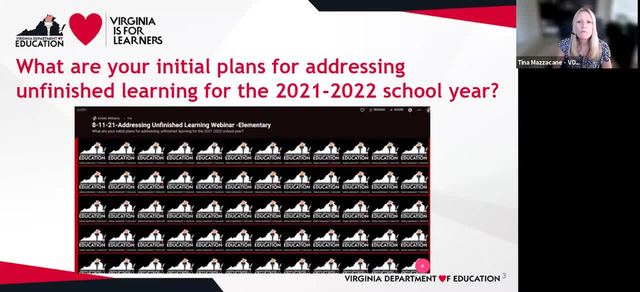 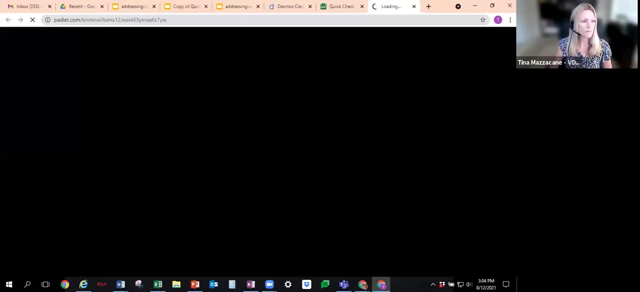 So, Kristen, did you want to share, or did you need me to share, or how did you? what did you want to do about kind of sharing? I think, Deb, you have it up on your screen, don't you? Yeah, Okay. 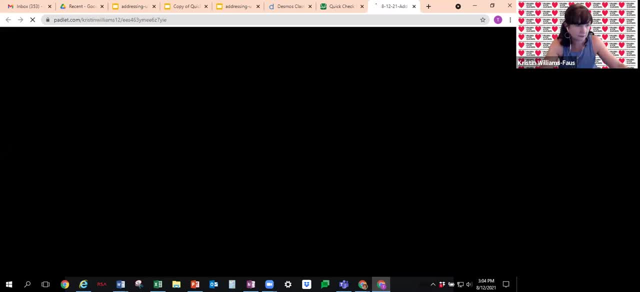 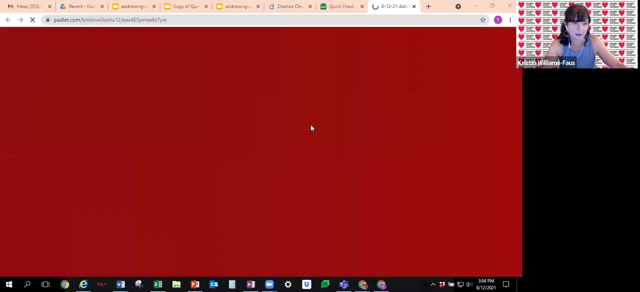 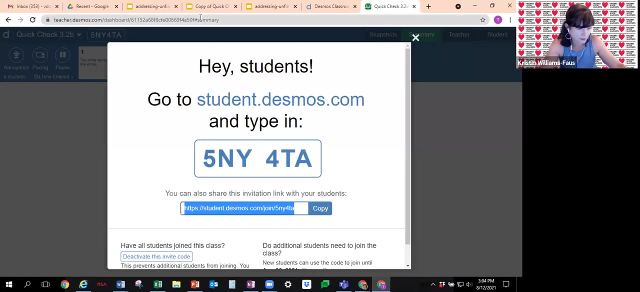 Thank you Awesome. I'm going to try to see if I can put this in your chat box. Actually, I think I might have accidentally put the yesterday's link into the chat. It doesn't look like anybody has clicked in there. Let me try. let me give you guys another link. I apologize, I think I accidentally gave you guys yesterday. 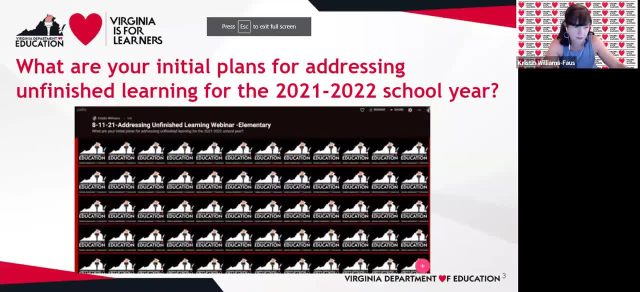 let's try this next one. I'm not sure why it's not working. We might need to ask people to put to put their thoughts in the chat, OK. so yeah, Plan B. there's always has to be a Plan B when you're a teacher, right? 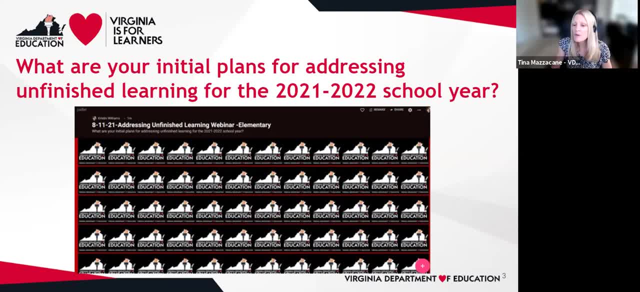 So, since the padlet isn't working, if you could just put into the chat what you you're planning for addressing unfinished learning for next year. So somebody said the written taught and assessed curriculum, focusing on what they lost using quick check. somebody said pre-assessment, small group instruction stations, standards based grading. 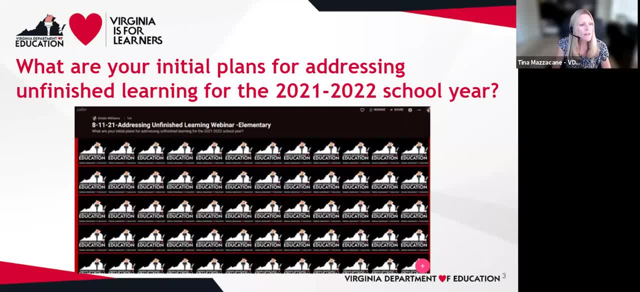 more pre-assessments and stations, formative assessment, intense intervention curriculum. Gosh, it's going so fast I can't read it. Reviewing vocabulary: that's one that the vertical planning and looking for student strengths. I like that. Using data from pre-assessments to drive instruction. 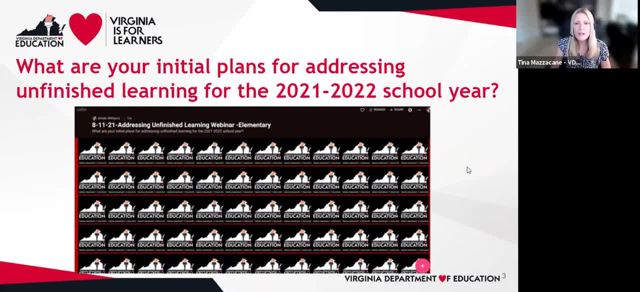 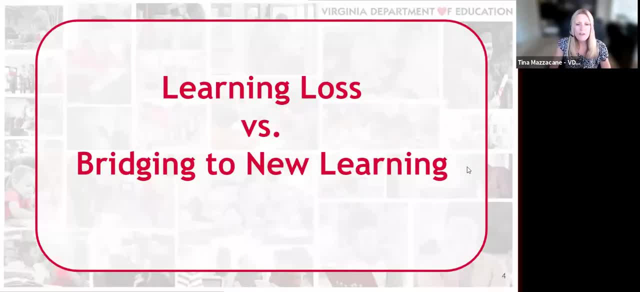 Great. So it sounds like you all have been thinking a lot about this, as we have been as well. Maximizing learning through quick checks, guided math groups- So lots of great ideas. We're going to probably expound on a few of those today and hopefully give you some additional resources. 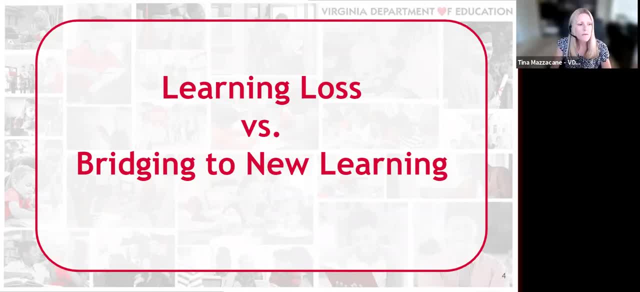 that will help you to think a little more about some of the the instruction that you might be able to plan for next year. So first we're going to talk a little bit about the idea of bridging to new learning, And you all have probably been reading things and see things posted on the Internet about how fall 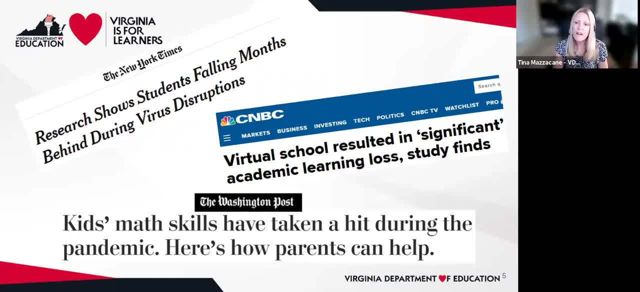 how far our students are falling behind in math and how they're going to have significant learning loss and how math skills have taken a big hit during the pandemic And we do recognize that students are going to have some unfinished learning And there's definitely things that 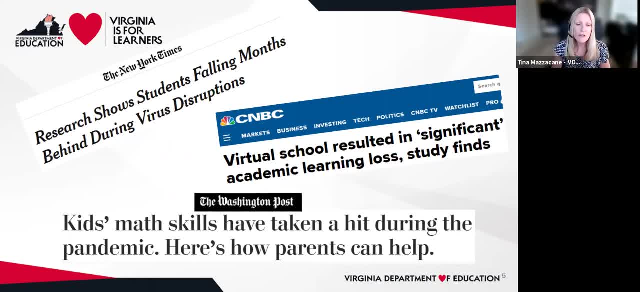 we're going to have to consider as we go into our planning for next year. But we really encourage you to avoid this kind of deficit sort of focus on learning for students and to try and pull together a more asset-based sort of approach. So, instead of saying we're going to be looking at, 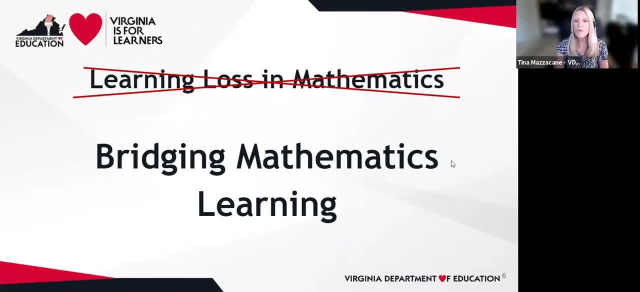 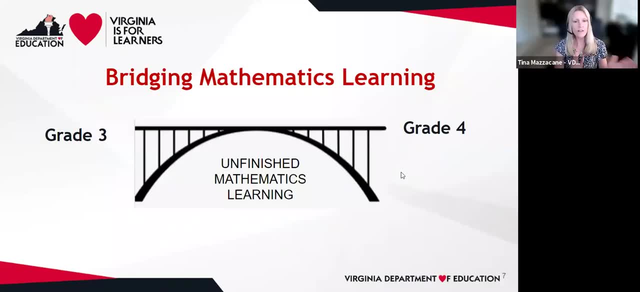 student learning loss. let's think about how can we bridge students to the grade level mathematics that we want them to learn this year, Recognizing that, yes, there are going to be some places where we're going to have to fill in, Kind of compensate for that unfinished learning. But if I'm a fourth grade teacher this year, 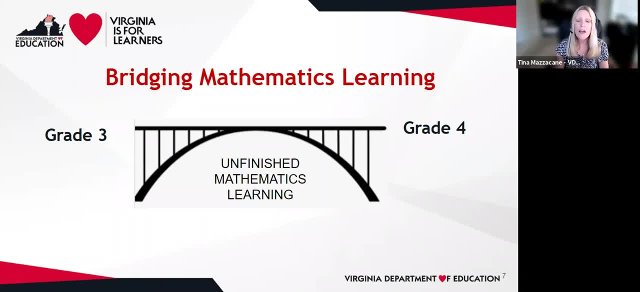 teaching mathematics. I'm going to make sure that I take every opportunity to bridge to that grade three content to ensure that my kids are ready for what I'm going to be teaching in fourth grade. So that's kind of what we're going to talk about tonight is: what does it mean to bridge to? 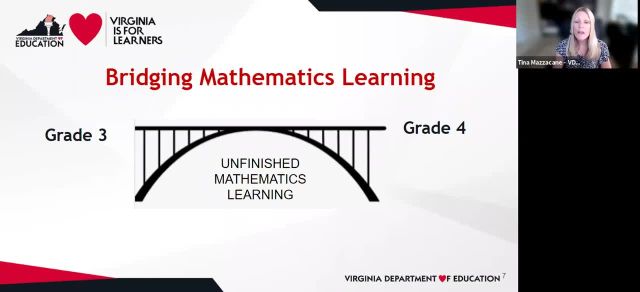 that new learning And how can we, number one, determine what that unfinished learning is for our students? And then, number two, how can we bridge to that new learning And how can we think about how we can fold that into our instruction? So on the next slide, I think it talks a little. 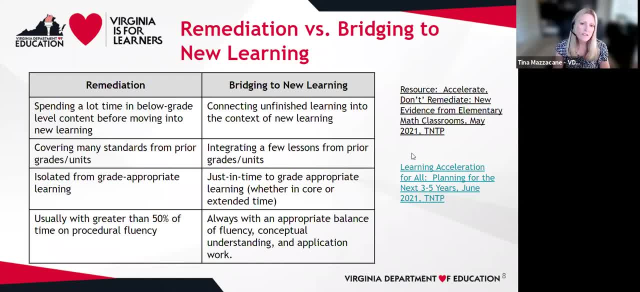 bit about the idea of remediation versus bridging to new learning. And when we bridge to new learning, we really do want to connect unfinished learning into the context of new learning. So, remediation- we typically spend a lot of time below grade level content before we even move into new learning. 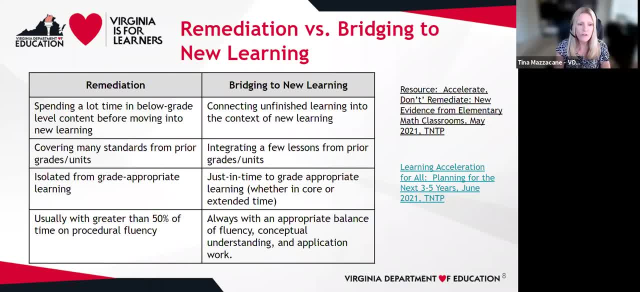 And that's not really what we want to do when we bridge to new learning. So we want to connect that content into the context of new learning, And that's not really what we want to do when we bridge to new learning. When we bridge to new learning, we cover a lot of standards from prior grades or 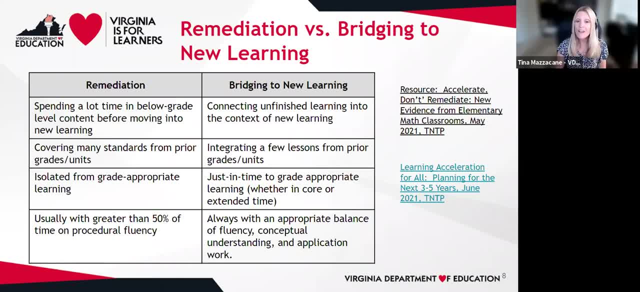 units And in bridging to new learning we want to integrate a few lessons from prior grades and units that we know maybe kids just didn't get that content at all last year, Or we know that there's quite a few students that are going to need some additional instruction In remediation. we 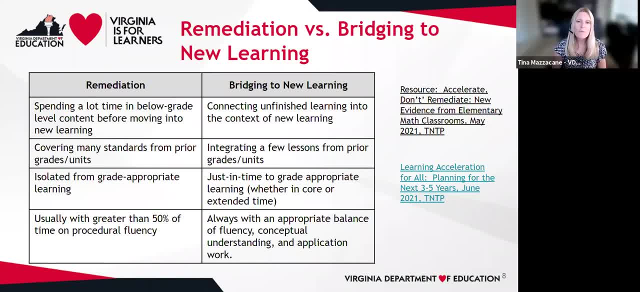 oftentimes isolate from our grade appropriate learning. But for bridging to new learning, it's that idea of bridging to new learning And that's what we want to do. So when we bridge to new learning, we want to have that just-in-time sort of approach to the learning. So, whether we're 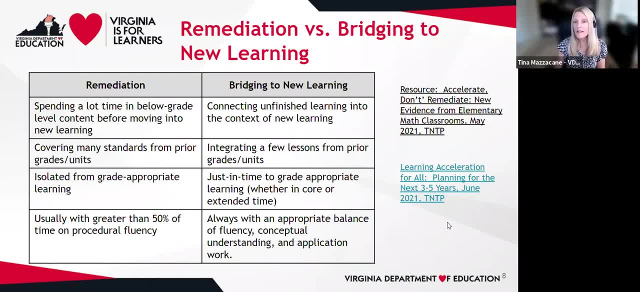 in a core academic situation or we're adding extended time for students, we still want that instruction to fill in the unfinished learning that students need to access that new learning And then oftentimes, with remediation, we're focusing a lot on procedural fluency. 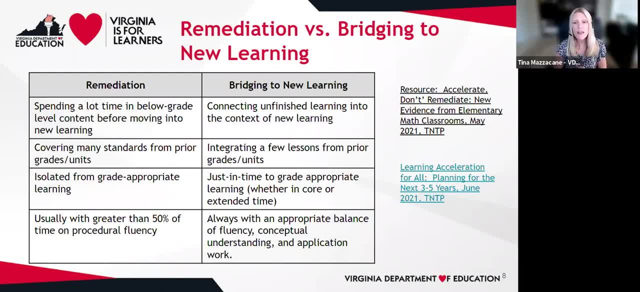 And while that is important- and we do want to focus on that in bridging to new learning, we really also want to make sure, is that conceptual basis there? How can we build that conceptual basis as we're approaching the new learning for the grade level that we're teaching? 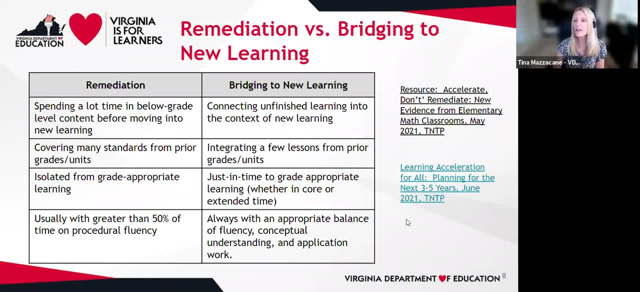 this year And how can we ensure that students are seeing how that content applies to what they're learning? So those are some differences. you'll see And you'll get a link to this presentation towards the end of the presentation where you can go to this resource that we have linked to. 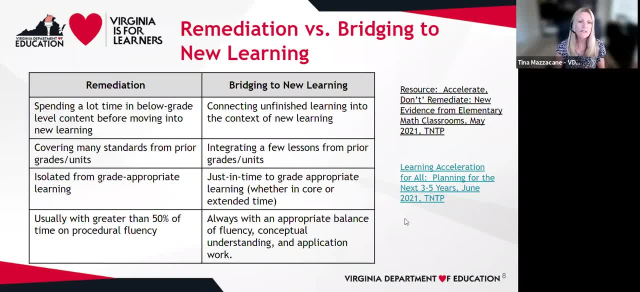 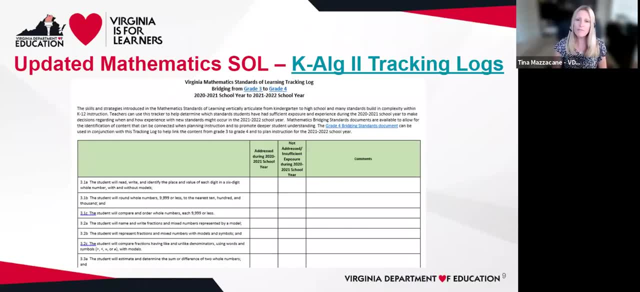 help you learn a little bit more about some of the ideas that this is going to be talking about. So if you haven't looked at these, these came out in March- not this past March, but the previous March. when the pandemic first came out and many of the schools began to close, We created what we called 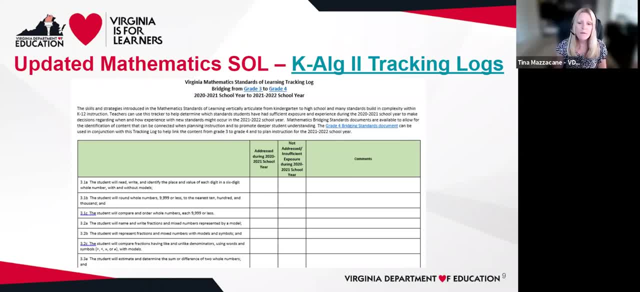 tracking logs for mathematics, And then the other disciplines also developed these, But they're very simple documents. So as a fourth grade teacher I might want to go to my third grade teacher and say, hey, what standards did you address during last school year, And which ones? 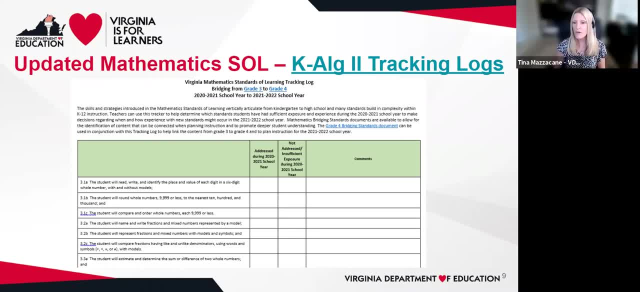 do you feel like the kids maybe didn't get enough exposure, or you know that you just didn't feel like you got a deep dive into last year? Because that's going to help me, as a teacher, to think about as I plan my scope and sequence and I think about my pacing, if I know that the teacher 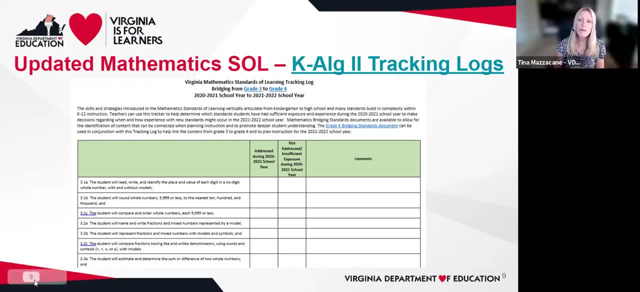 last year didn't get to this particular topic, then I'm going to have to really build in that addition. I'm going to have to really build in that additional instruction for my students, And how am I going to fold that in? And I really need to be thinking about that And that's something we 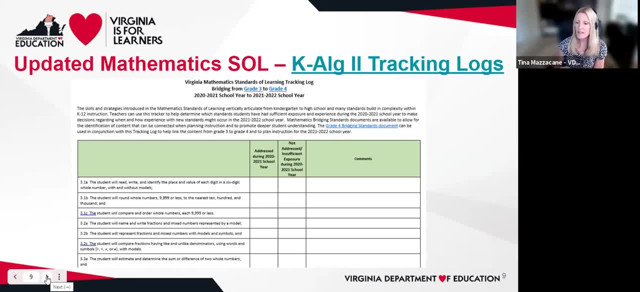 need to be thinking about ahead of time and not wait until we get to the moment. But if we can plan ahead of time and work with the teachers from last year, that's going to really help inform our instruction, Knowing that some kids are going to move from different places or different schools. 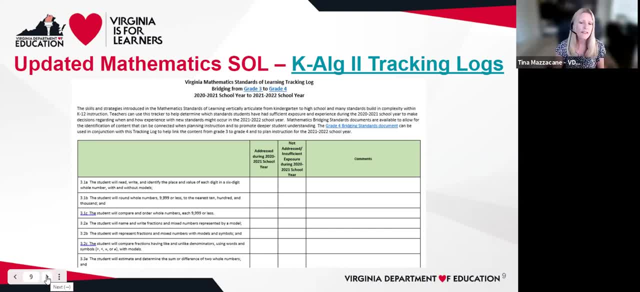 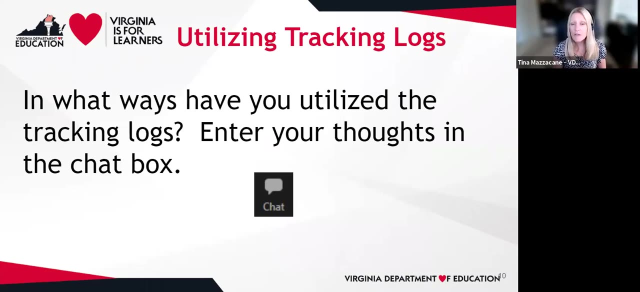 but as a whole, if we can start to get a handle on that, that's going to be super helpful. So those tracking logs are available from K all the way. So we want to see if you've been able to utilize the tracking logs at all. Have you had a chance to utilize those? 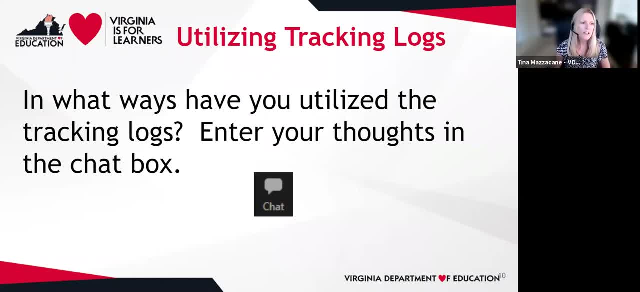 And if you have, what have you done with those? So in the chat, if you could just kind of share, have you used the tracking logs at all And if so, how did you use them? I think Kristen put a link to those as well in the chat. 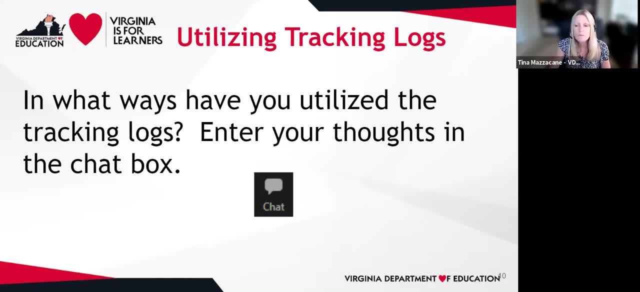 So Dawn said they used them for summer school for kindergartners to see what they may have needed to touch on, Filled them out as a grade level at the end of last year, Heather said. Amanda said to use them for students attending summer school to see which skills were covered and which were only. 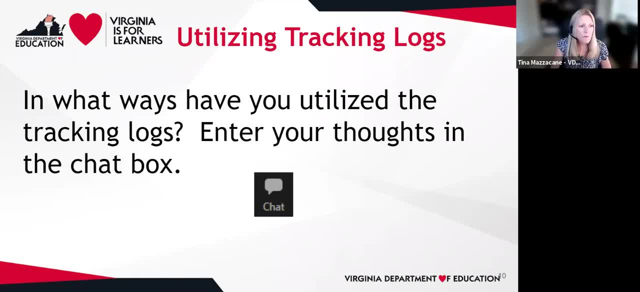 touched on. Sarah said they used them to prepare for this year's pacing- Great, Sarah. Hillary said they used them to see what skills are missing. Carrie said she hasn't used them but she's eager to to implement them. So it looks like a lot of you are taking a look at them and trying to utilize those, so that's great. 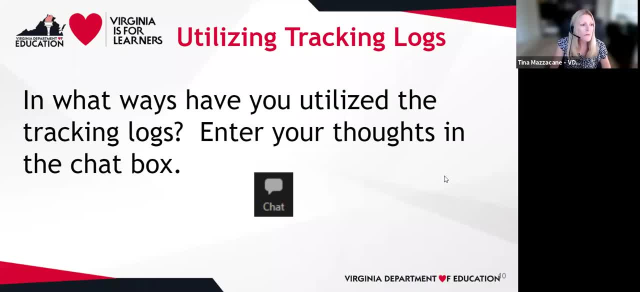 Use them in collaborative weekly planning meetings, And that's great, Brooks, that's a great idea Thinking about how we modify our pacing and thinking about sharing them with focus groups for planning for next year. So lots of great things looking vertically at the curriculum. 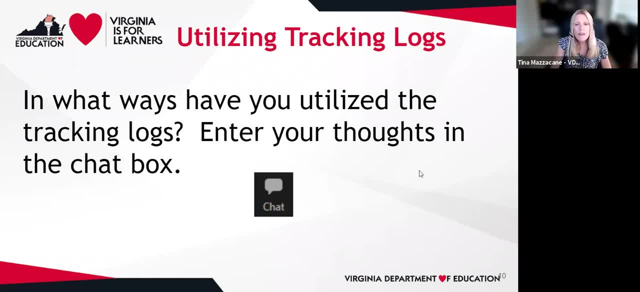 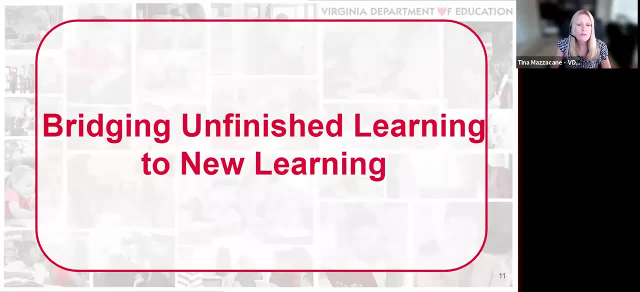 That's a good idea too. So we're happy that we can introduce you to this particular resource and glad that some of you have already found it and are utilizing it. So I'm going to turn this over to Kristen. Kristen Williams is our math instructor. 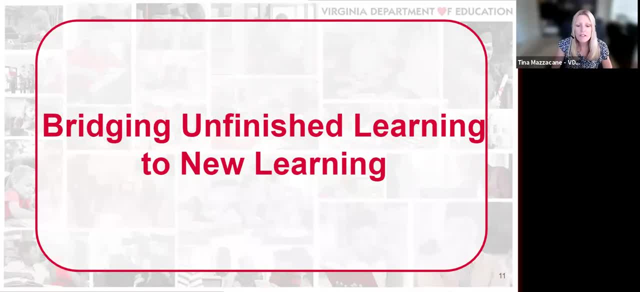 Thank you, And she's the professor of math and special education specialist here at the Department of Education, And I believe it might be Deb that's going next. Who's going next? I always forget. You got it right. this time, I did. 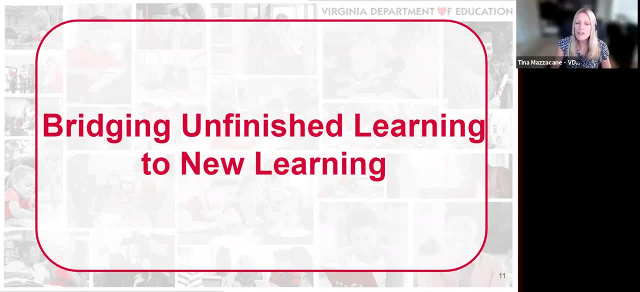 Good, And when you, when you turn it over to Deb, will you make sure that you introduce her, Because I failed to do that at the beginning. I apologize, Thank you, I will definitely do that. So, welcome everybody. So I'm going to go. I'm going to talk a little bit more about this whole idea of bridging unfinished learning to new learning. 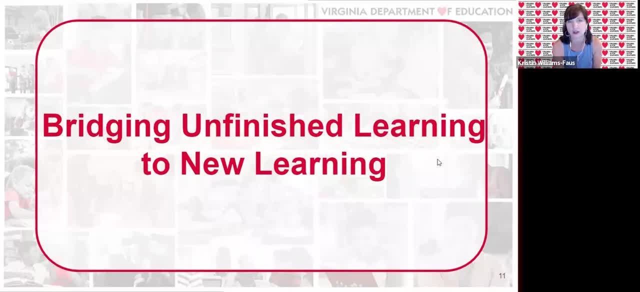 Because that's really important. So stay tuned. really, how we want to think about this year, How can we bridge the learning that our students have already had and what they do know the strength? you know the strengths that they have. how can 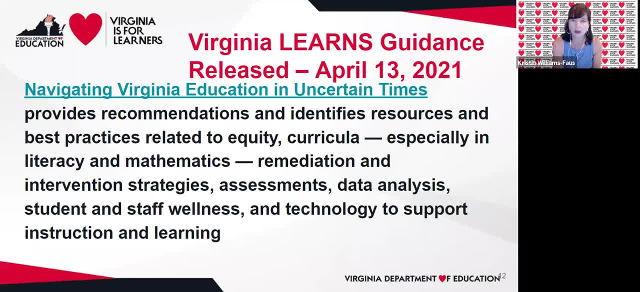 we bridge that to where we're taking them this year. So I put a link in the chat box to our Virginia Learns page and that will have a lot of links that we're going to be kind of referring to throughout the section. Back in April we released this guidance. It was called Navigating. 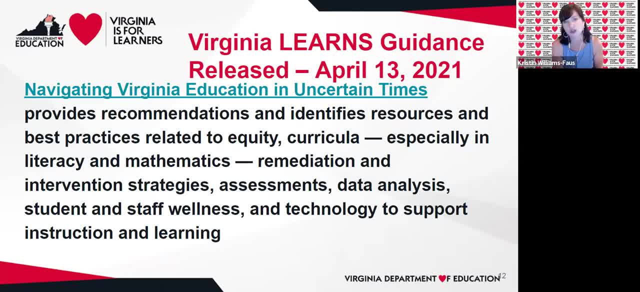 Virginia Education in Uncertain Times and there were educators that came together all across the state to put together this guidance, for how do we go back to school, you know, after being in a virtual world, and what are some things that we need to think about. So this guidance, 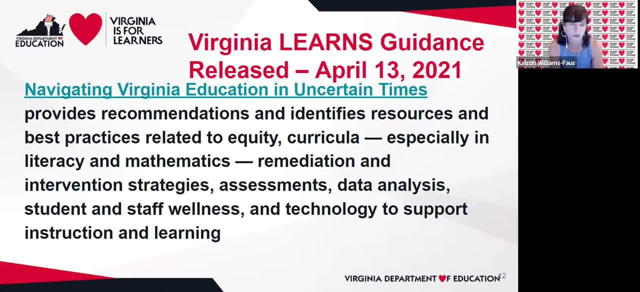 provides recommendations and really identifies resources and best practices when we're thinking about equity and curriculum, and it really has a big focus on literacy and mathematics, Including intervention strategies, what we need to think about for assessment, how we should analyze our data and our social-emotional health, which is also really 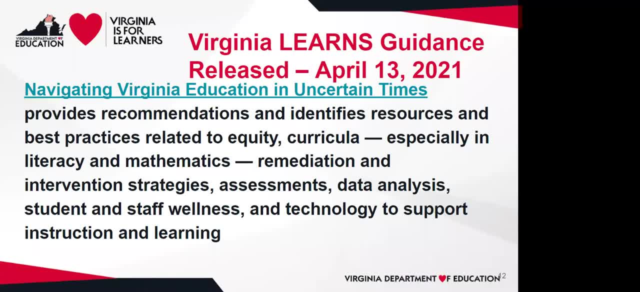 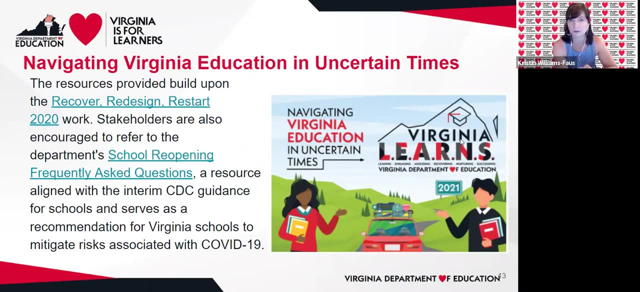 a big consideration. So that page, that or that website link I put in the chat box will take you to this document. So this is the front cover of it, and it was actually kind of an offshoot from our what we call the Virginia Learns website, which is a website that we've been working on. 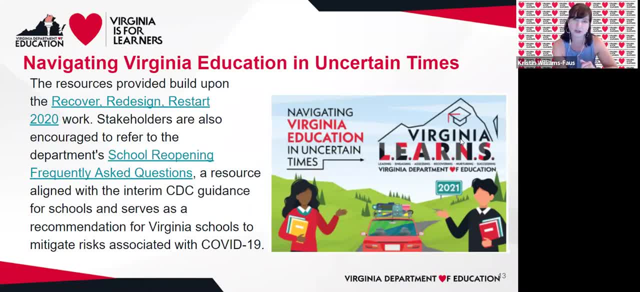 for a long time, and it's called our R-Cube document, the Recover, Redesign and Restart, which was created right after the initial closures in March of 2020, and it also includes, if you'll notice, on that same page it has a link to the frequently asked questions because, as you know, things are changing every day in terms of what is going on with the pandemic, so that page is continuously being updated in terms of what you know. what are our frequently asked questions? 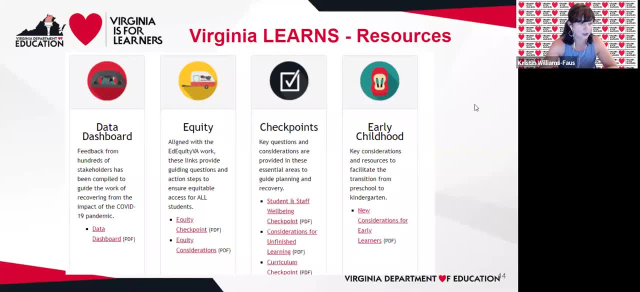 You'll also notice as you go through the page that we have. these are actually called bootstrap boxes of different information in the document. So the document is divided into these eight sections so you can get to different parts of the document quicker. but there's a section that 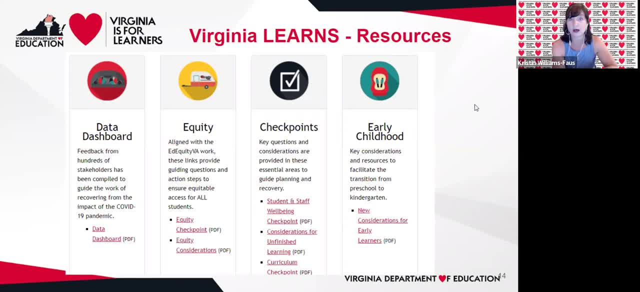 includes data. They used a lot of stakeholder feedback throughout the state to come up with these recommendations, something that was really kind of the whole. what was kind of in the forefront of everybody's minds as they were thinking about this guidance was equity, and it refers to some equity checkpoints and so forth. and then the black. 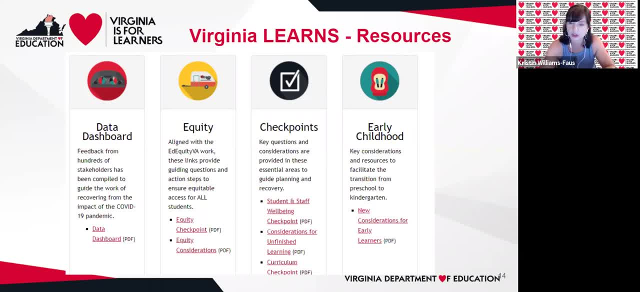 checkmark is checkpoints in consideration for, you know, social-emotional learning. This is a section that has a lot of good recommendations in terms of our students with disabilities and what we need to think about with their needs. There's a section on early childhood. There is a section on if you've noticed, if you go to. 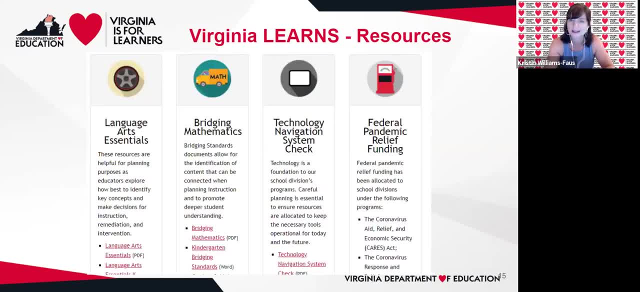 this next slide, Deb. there's a section on language arts essentials, and then of course, we're going to be talking mostly about the bridging mathematics section, and then there's some really good pieces that give us some good guidance in terms of technology, because obviously we've a lot has. 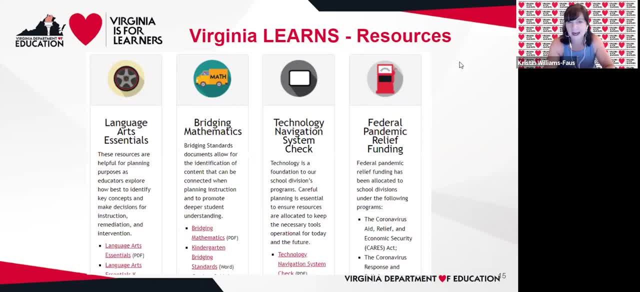 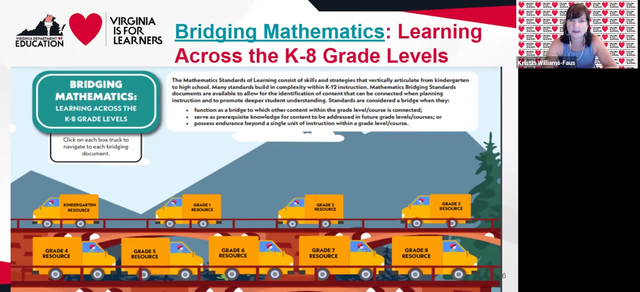 changed and improved in terms of our technology. and then there's a section on language arts essentials and then there's also information about all the federal pandemic relief funding that's available. So if you go to the bridging mathematics section, if you, if you go to the actual PDF of the entire document, this page comes up where you have, where you see these trucks. 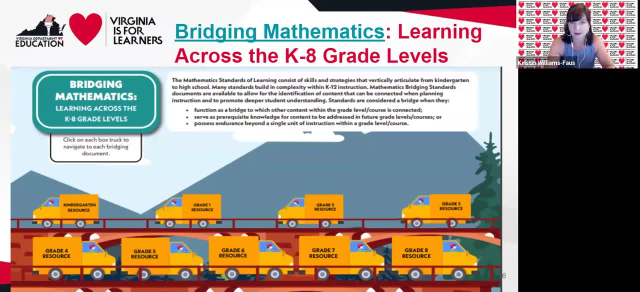 So you can either access the bridging documents through this PDF or that link that I provided in the chat. just that actually probably gets them, gets you to the bridging documents. The bridging documents quicker, but you can click on. I would go ahead and click on whatever grade you're most interested in in terms of what you're teaching or where you're giving, if you're coaching or your administrator or so forth. 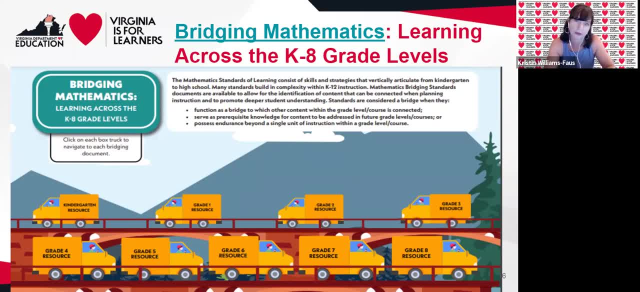 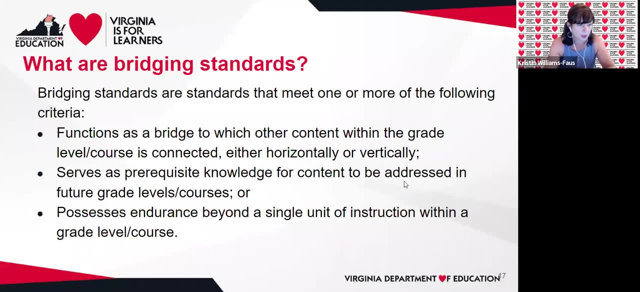 So go ahead and click on one of the bridging documents for the grade that you're interested in, and we're going to talk a little bit about what the bridging documents include. So, as you're opening up your particular grade level, we're going to talk about. 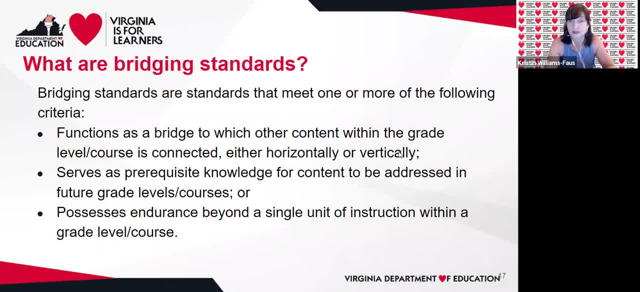 notice that, as you open it up, there are standards that are bold, that are in bold, and not not all of them are in bold. the standards that are in bold are considered bridging standards. so when we were, when we were looking at all the standards and designating which standards would be considered, 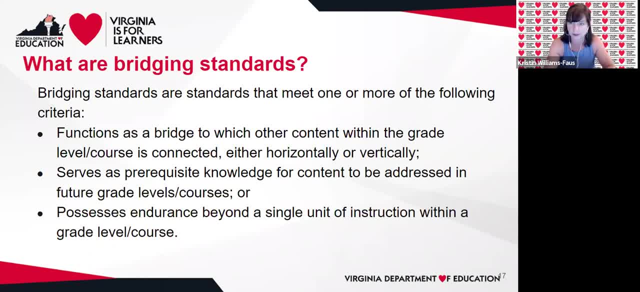 bridging standards. we really looked at these three, three criteria and you'll notice that these three criteria are described at the top of the document. so bridging standards really function as a bridge to which other content within the grade level, so there's horizontal connections or content. 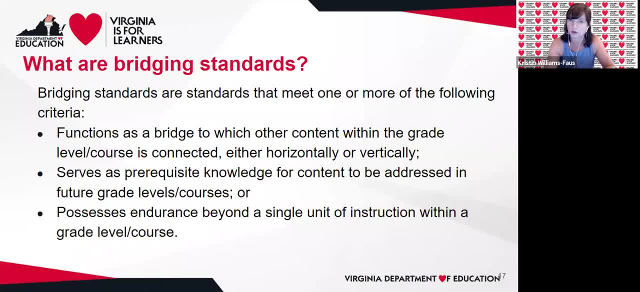 before the grade level or after the grade alert. so you have those rural connections that the standard really serves as prerequisite knowledge for content that's going to be really hit upon in future grade levels, and then that content really possesses endurance beyond a single unit of instruction. so those were kind of the three. 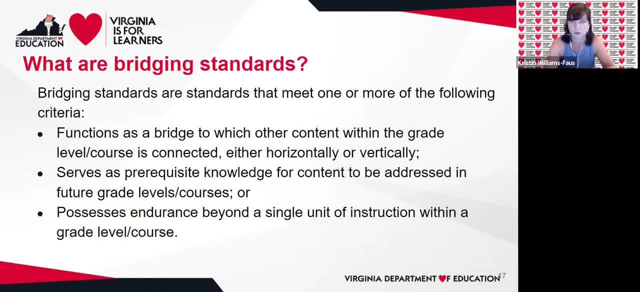 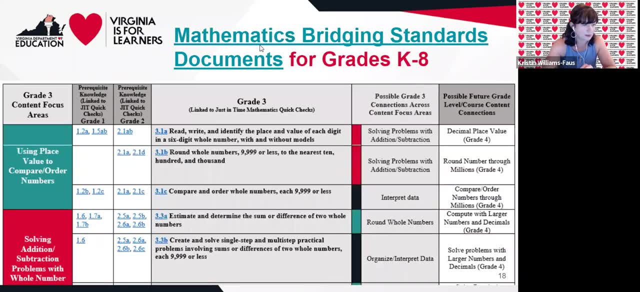 criteria that we really looked at and determining what standards were bridging standards. so hopefully you've all had a chance to open up one of the bridging documents, um, and this example on the screen is actually from grade three, um, and you all are looking at different grade levels. uh, according to what your, what your focus is, but the format of all the 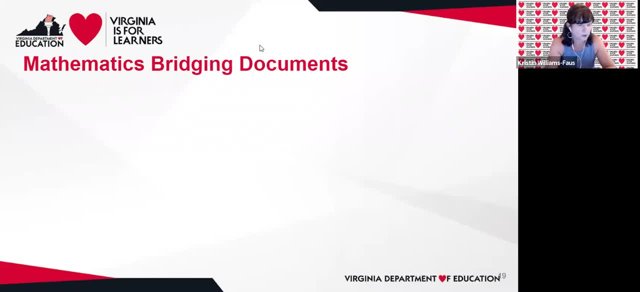 bridging documents are the same. so that's why we're going to look at the different grade levels and then we're going to look at what the standard values are for the different grade levels. so the first thing we want you to kind of think about is: what do you notice about the bridging? 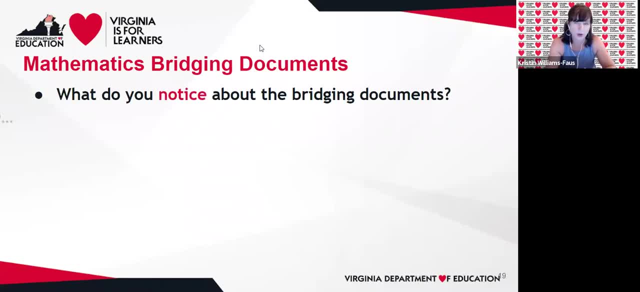 documents. so, as you're taking a look, go ahead and type in the chat box what are some things you notice about the bridging documents, and i will kind of monitor the chat to see what you're noticing. we notice the color coded connections. we notice the content focus areas, the 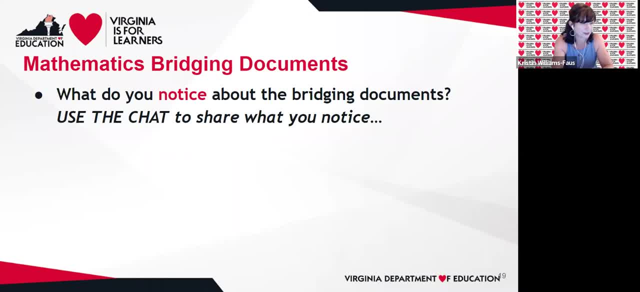 prerequisite knowledge that are linked to the Quick Checks, Well organized with links. the vertical alignment hyperlinks to Quick Checks. Looking at the future connections, Let's see here- SOL numbers are similar for easier comparison: The vertical alignment with the Quick Checks. 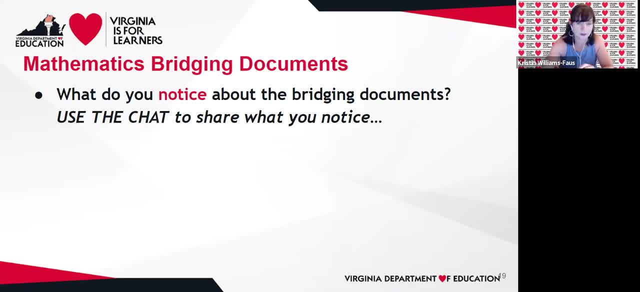 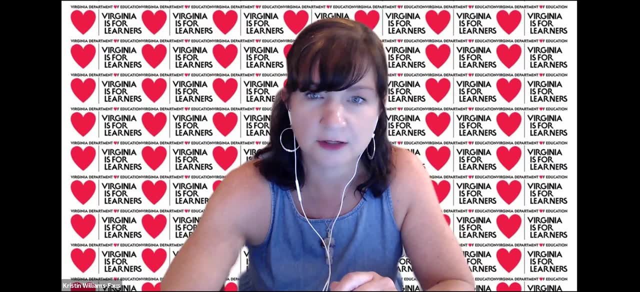 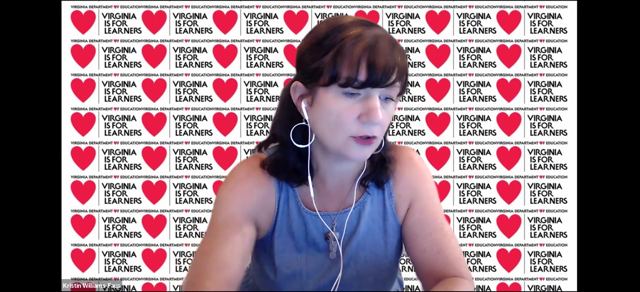 So, yeah, you're all noticing some similar characteristics. It looks like we might've lost Deb. See if she ends up being able to come back to us, or I'll have to share my screen Links to previous learning and future learning. All right, awesome. 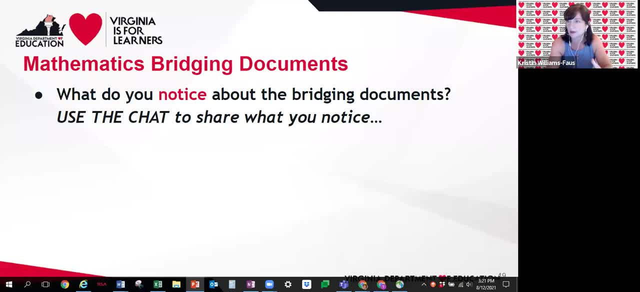 So now we want you to think about. so you, you kind of have entered your noticings. So what are you wondering about these? So probably a lot of you are familiar with this routine. What do you notice and what do you wonder? 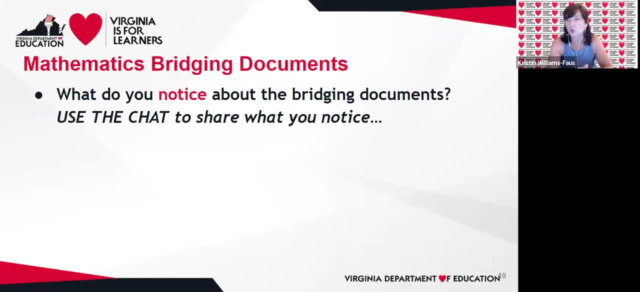 So, as you look at these documents, what do you wonder about them? So go ahead and enter your thoughts in the chat in terms of what are you wondering. Is anybody wondering anything about these documents, Wondering about the links to resources for supporting them? 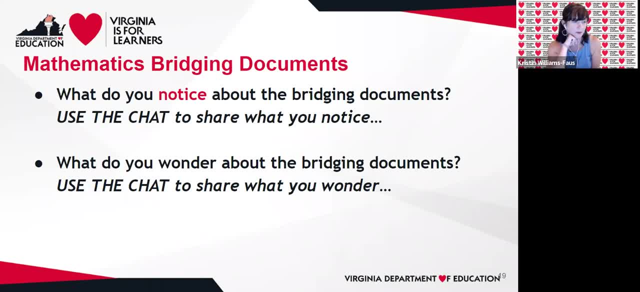 Okay, so actual instructional resources: Is it a suggestive progression of learning? Is it a progressive progression of learning? How will students be affected if we don't emphasize the non-bolded ones? And I think that's a really good wondering, And I think we want to make the point. 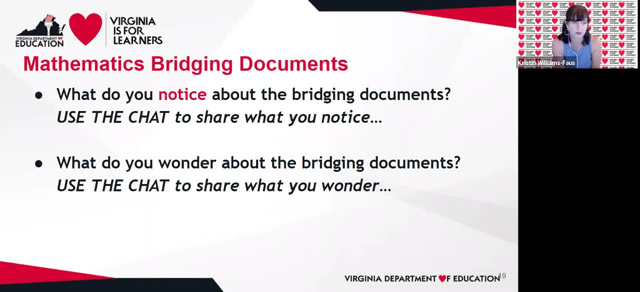 and Tina and Deb, you can elaborate on this if you would like to. We're not saying to not teach the other standards. So we don't want you to think that you, you know, you're just emphasizing the bridging standards and not worrying about the other ones. 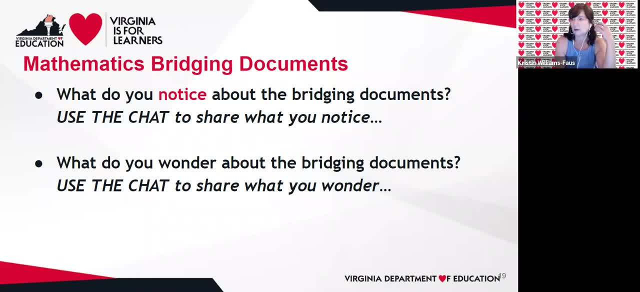 You are still teaching the other ones, but you're thinking about, when you're talking about bridging standards, how can you connect, make those connections to all of the content and really make sure that those bridging standards are connected to other content in your units? 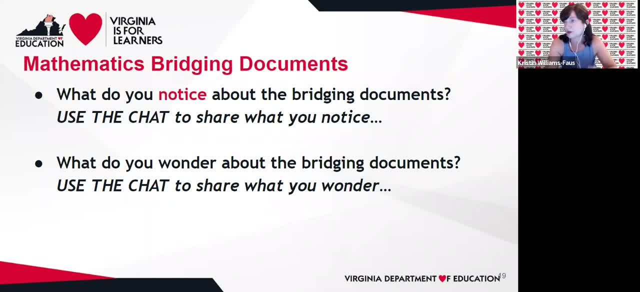 and that you're thinking about how they're going to affect where the students are coming from and where they're going to in their future learning, How to integrate them into planning. That's a great wondering. Are the bridging standards aligned with the testing blueprint is a question. 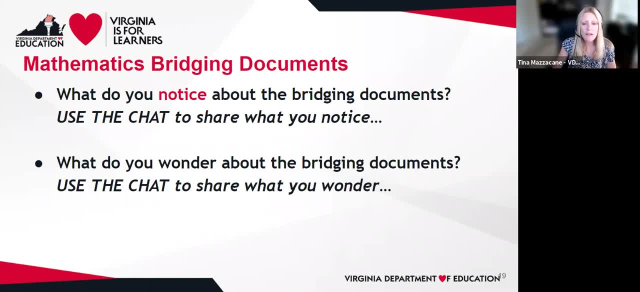 And I would say that the answer to that would be kind of what Kristin already mentioned- is that the bridging standards aren't meant to exclude any content from being addressed. It's just to really think more about which content do we want to be sure that we emphasize and connect with other content. 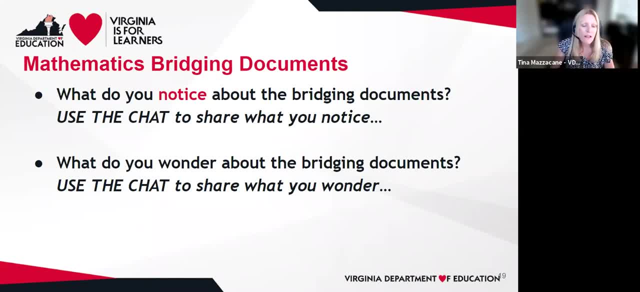 So I don't think that it has any impact on the content. I think that's a great question. I don't think that it has any impact on assessment, So your blueprints would be still valid. Clara had a good question in terms of how. 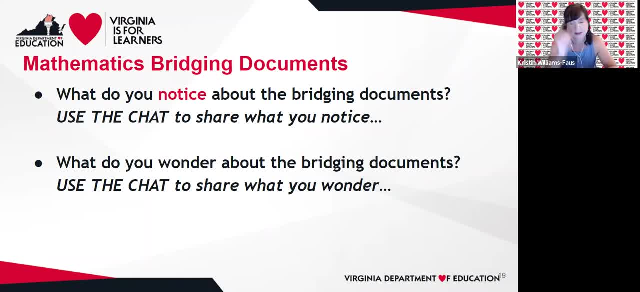 to tie the standards and write appropriate goals for IEPs. And I think that's a really good question, Tara, because when you're thinking about, when you're writing your math goals for your students, who need math goals that have IEPs- 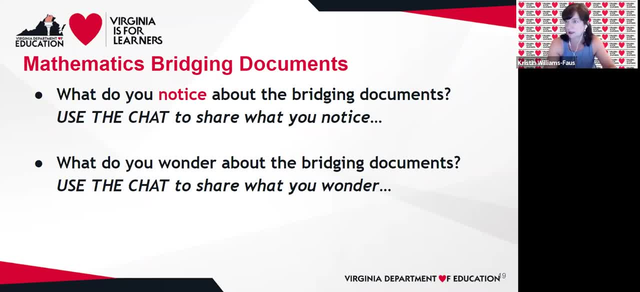 of course you're basing them on what their needs are and what their strengths and their weaknesses are. But again, if you're looking at these bridging standards and you need to kind of prioritize what you are working on with your students, that will kind of help you think. 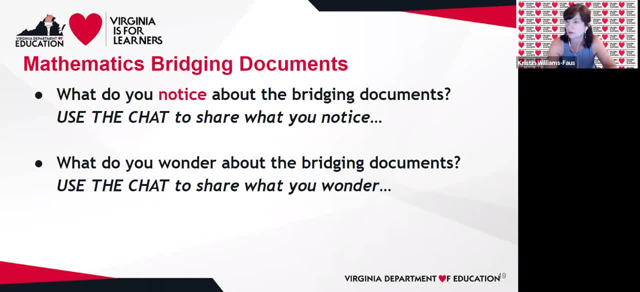 about which areas you might want to focus on for the IEP, Kristin. I saw two questions that really stuck out for me that I think we'll be able to address during our session today, which is really great. There'll be a time a little later on Sharon, where we can talk about the best ways. 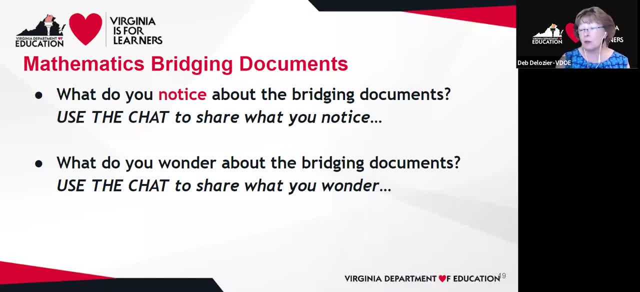 to utilize some of these resources either as classroom teachers or as leaders with as math coaches or math specialists later in our session. So that'll be a great time as we're exploring some of the resources that aren't as familiar to you. You'll be able to talk with others about that. 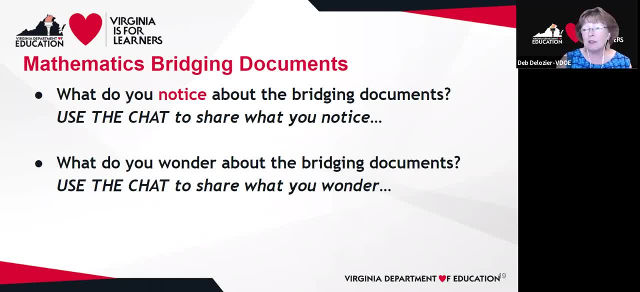 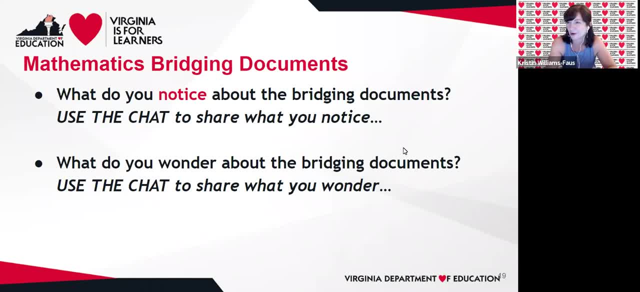 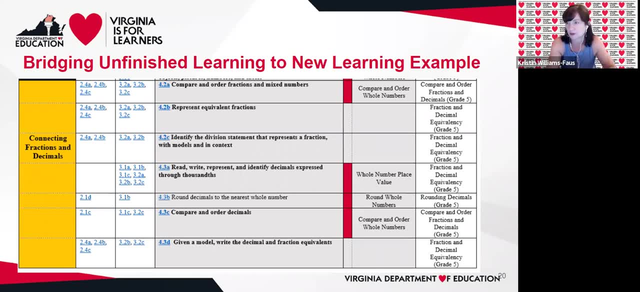 Yes. So, speaking of which, that's kind of our whole goal is to kind of help everybody think about how can we use these documents, how can we use these resources to really be strategic in our planning for the school year, Because we know that, just like last year, it's an unprecedented school year again. 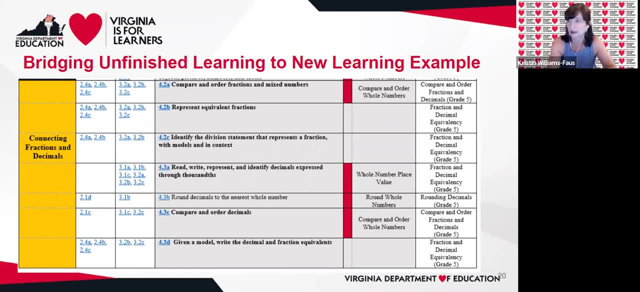 So how can we kind of get the most bang for our buck in terms of being strategic with our planning? So we thought maybe the best way to kind of give everybody some ideas is to actually kind of put ourselves in the place of a teacher and what we would think about as a teacher. 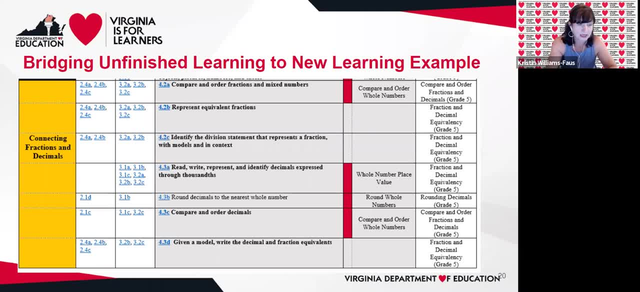 as we're planning. So I'm going to pretend that I'm a fourth grade teacher and I'm going, and I'm actually getting ready, to teach equivalent fractions. I'm getting ready to do a unit on equivalent fractions. So when I look at this bridging document, I look at the prerequisite skills. 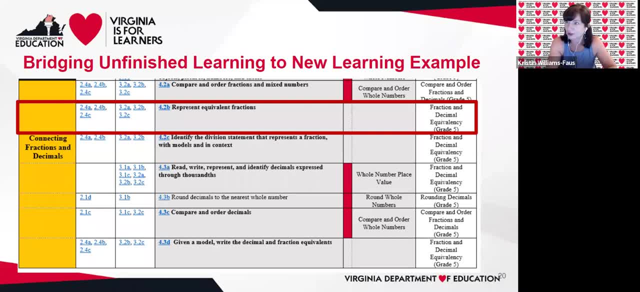 We can see that the prerequisite skills in third grade are all the 0.2s, so 3.2a, b and c. And when I look at 3.2b, 3.2b has to do with representing fractions as quantity and modeling. 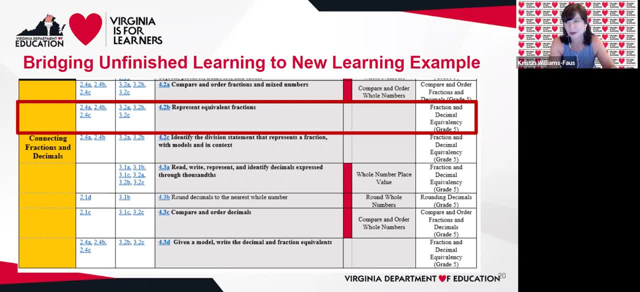 fractions and mixed numbers. Well, obviously, a student has to really have a good grasp of modeling fractions and mixed numbers before determining whether they're equivalent. So it's really important for me to know, before I start my unit On 4.2b, where my students are in terms of modeling fractions as quantities. so I need 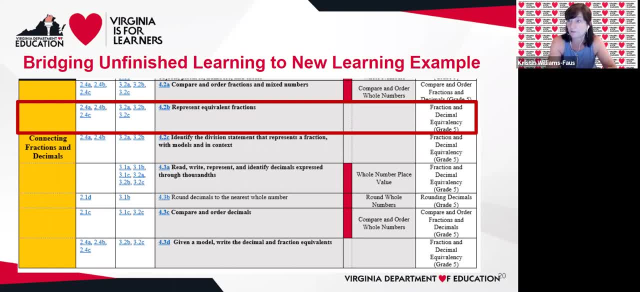 to have. I really need to take a pulse check and formatively- not formatively so- actually pre-assess where what do my, what are my students coming with in terms of the third grade skills? So when I click, when I click on 3.2b in the bridging document, that actually takes me. 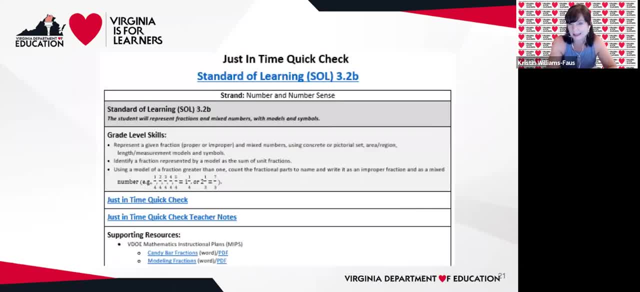 to the quick check for 3.2b And I can see 3.2b. It's representing fractions and mixed numbers with models and symbols. So I really want to see what my students are coming to me with in terms of their representing. 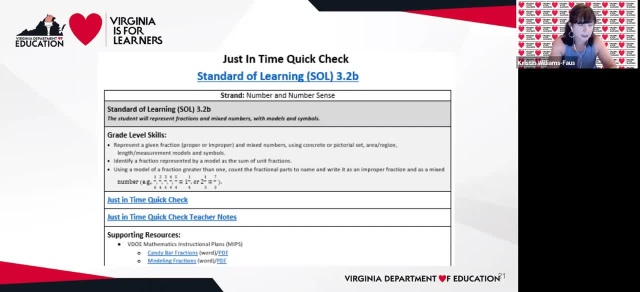 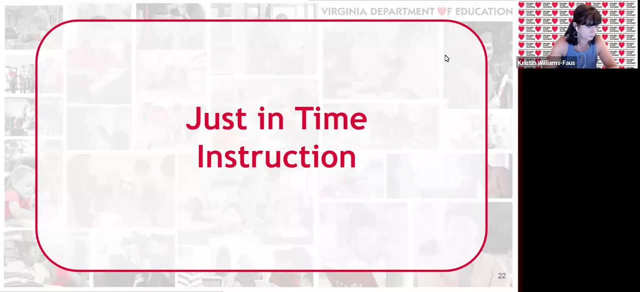 fractions and mixed numbers with models and symbols. So Deb is going to kind of take us through the process of what you might do as a fourth grade teacher, thinking about this instruction. Deb, I think you're muted And actually I was supposed to introduce you. I was supposed to introduce you. 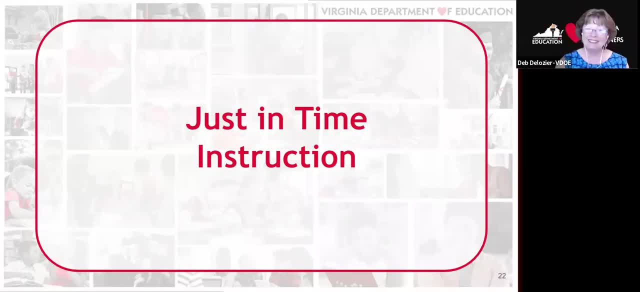 Deb Delozier is our mathematics specialist, So we have three people in the math office of the BDOE. Tina is our math coordinator for all the grades. I'm the math and special ed specialist and my main focus is the middle school grades. 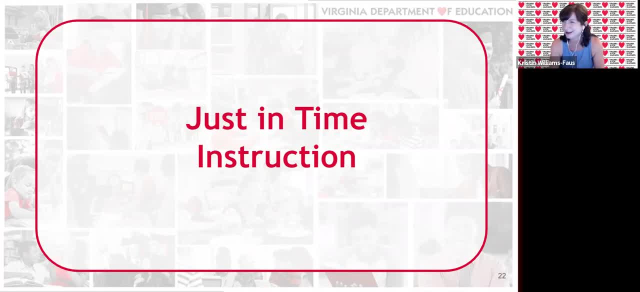 And then Deb is our elementary expert, So that's why she's going to kind of go through the elementary process with you. So it's great to be here with you today and we thank you for taking the time to join us. We're going to take a little time to dig deeper into utilizing the quick check and give some 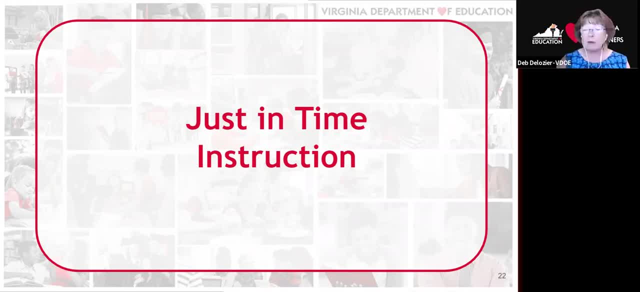 examples of ways that we've seen teachers utilizing them, And we know we've kind of. for some people, we've been beating this drum about quick checks, but we think that they will definitely serve as one way that will help you to bridge prior. 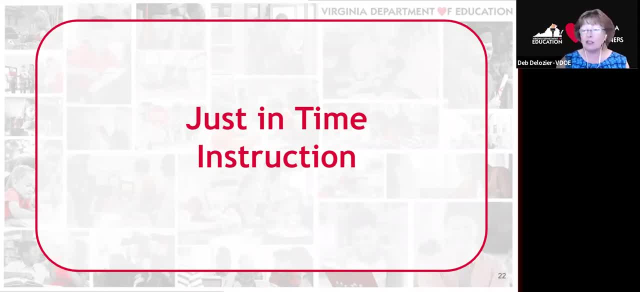 grade level content to the current grade level content, And we've made some progress. We've made sure to include some new ideas and new strategies that we think will be helpful to you. So let's go ahead and move forward. Many of you utilize oops, before I start that many of you utilize math routines in 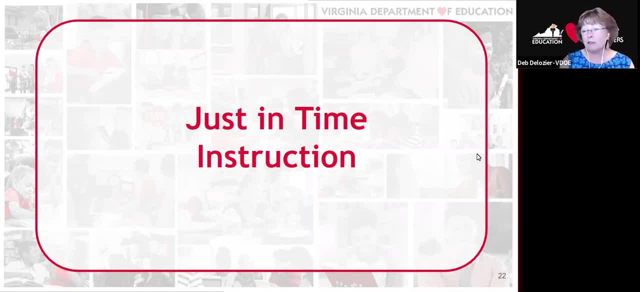 your classrooms as a launch right, And you use those often to formatively assess where your students are in terms of their current understanding and also sometimes to link to prior knowledge. So one of those routines that many of you are familiar with is the quick check and give. 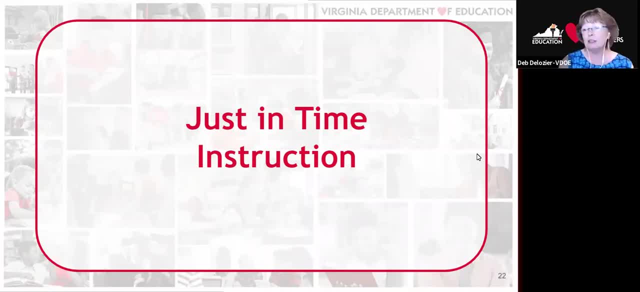 some examples of ways that we've seen teachers utilizing the quick check and give some examples of where your students are in terms of their current understanding, and also sometimes to link to prior knowledge. So one of those routines that many of you are familiar with is the which one doesn't. 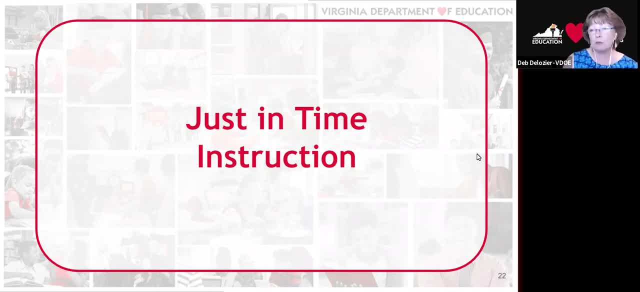 belong And to prepare you to utilize or to participate with the which one doesn't belong exercise that we're going to do in just a moment. we want you to be able to utilize the annotate tool. So if you look at the top of your screen, you should see a little green strip that says: 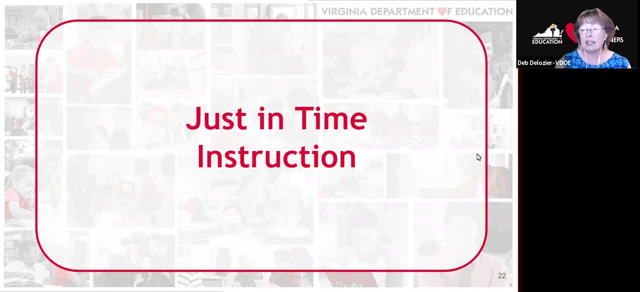 Deb DeLozier is sharing her screen And just to the right of that you will see view options. So if you click on that little arrow there- view options- and go down and click on view options And you'll see a little green strip that says Deb DeLozier is sharing her screen. 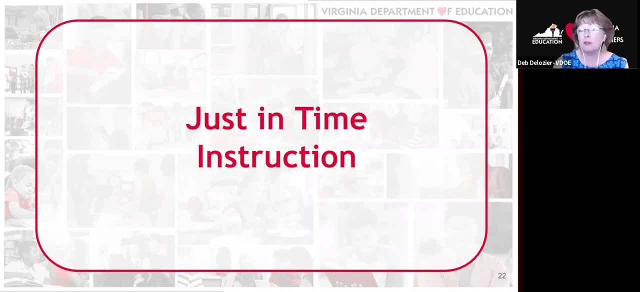 And just to the right of that, you will see view options. So if you click on that little arrow there- view options- and go down and click on annotate, you're going to see a strip that will allow you to. it will allow you to see some little. 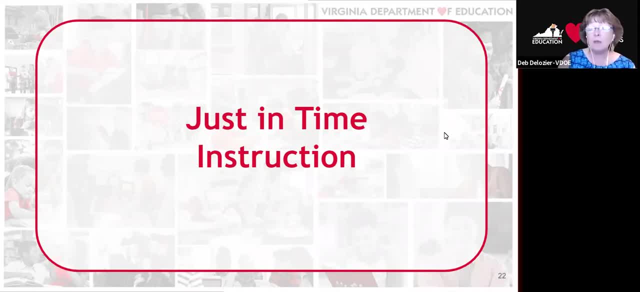 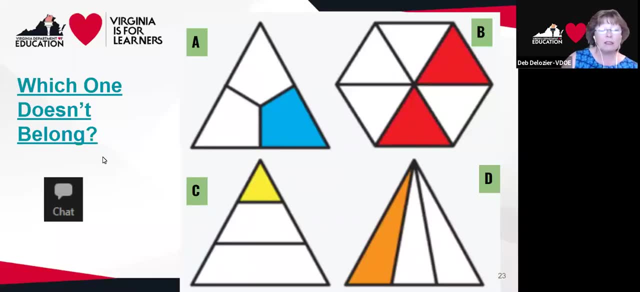 stamps and things like that. So, Karen, I can see that you found it already, And so what we're going to ask you to do is- we're going to click on the annotate and we're going to come to this screen- is utilize the annotate feature to decide which of the following does not belong and put a little. 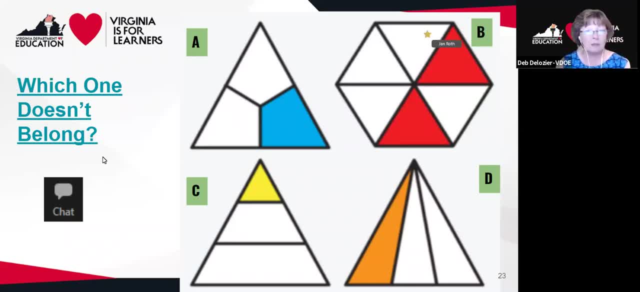 stamp on whichever picture you feel doesn't belong. So Jan just put her star, Denise put hers. I can see others adding theirs, so go ahead and add a symbol or something that lets us know which one you feel doesn't belong. Poor Dee doesn't have any takers. Won't anybody take Dee? 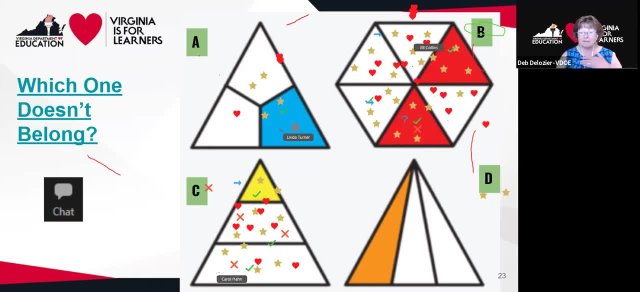 Oh, there we go- a couple of folks- And if you aren't able to use the annotate feature for some reason, please feel free to use the chat and just put in whichever letter you feel you'd like to choose. The annotate feature is is fairly new to Zoom and we have heard from others that use Chromebooks that you 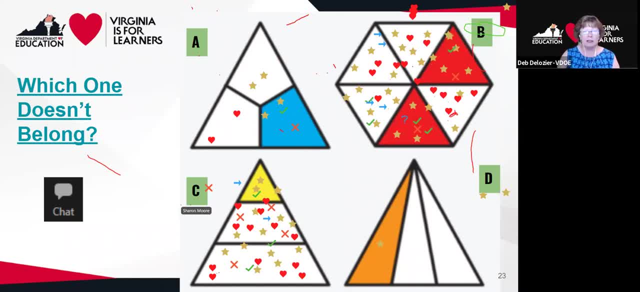 don't have that feature on some Chromebooks, So just go ahead and put your thoughts in the chat. that way, you can still participate in the discussion. Okay, so hopefully everyone had the chance, and if you want to get rid of your stamp so that you're not continuing to put marks? 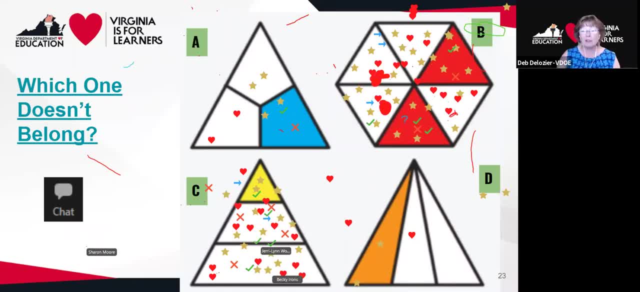 on the screen. you would go over and just click on mouse on that strip. that gives you a stamp. So that's the one that gives you options. So let's hear from some folks in terms of why they selected a particular shape and decided that that one is the one that doesn't fit. So if you selected 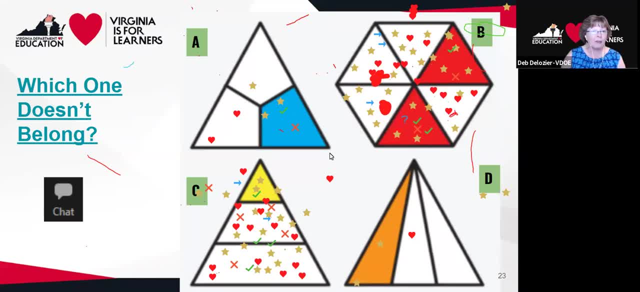 A as the shape or the picture that does not belong with the others. would you put in the chat box, please, why you feel like A doesn't belong? Yes, we would definitely decide that one only because it has an A, but it gets. 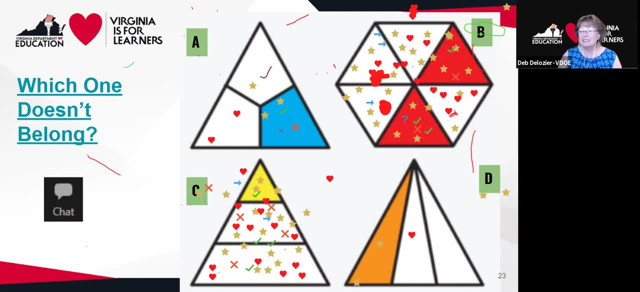 a little bit more complicated. if you want to use A, It does give you a level of confidence that this is the one that goes the Löwe way. So what the answer is is, I would say, the shape of it. It does give you a little bit more confidence. 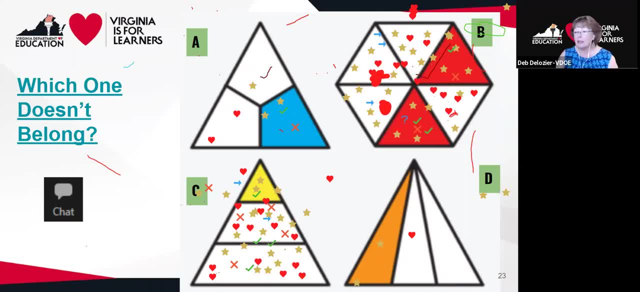 If you put a number of things in the chat box, itHHES also gives you a more personal vision of what it would like to be. Okay, Some people have changed their mind. The shaded section is a quadrilateral and not a triangle as in the other shapes. 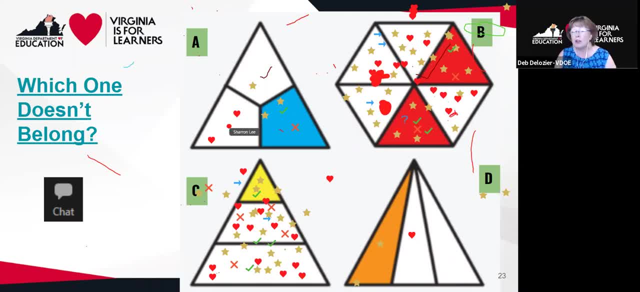 I selected this because it's the only one that does not. It's not taste in the shape of the triangle. Okay, so we're talking about A right now, So let me go down to the A folks. It's the only one that has a third shaded. 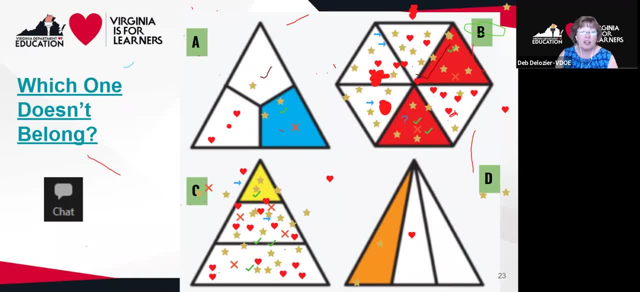 So, Audrey and others, are there other shapes represented that have a third shaded? Someone says the shaded part is not in the shape of a triangle. My bad, Sandra. that's what we want kids to notice, right When they notice something or they make a statement. 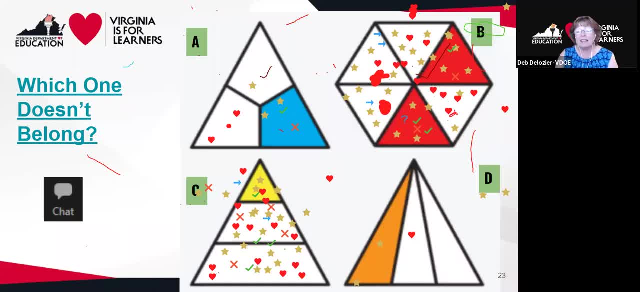 and then they realize, oh, that's not right, I needed to change my mind. I love that when that happens in class, because kids learn that math is about thinking and that sometimes we don't have to revise our thinking, right, So that's wonderful. Thank you for being willing to put. 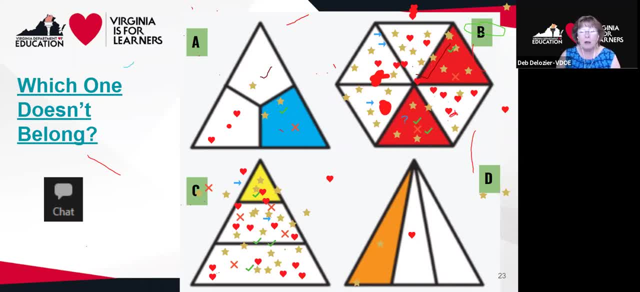 yourself out there. Oh, and so Susan is saying: well, B and D are both thirds. D can be simplified or B can be simplified to a third. I'm having a hard time reading all these. They're going so fast, So let's go ahead and transition to B, If you selected B as the one that doesn't belong. 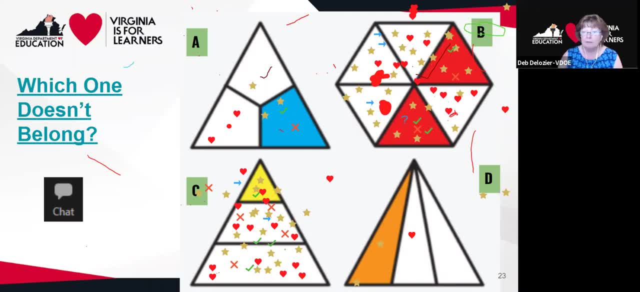 would you say why B does not belong, So only the people who selected B would be responding right now. B has more parts shaded. Jamie Correct, B has more parts shaded. It's not a triangle. There are two parts shaded, where all the other shapes only have one right. 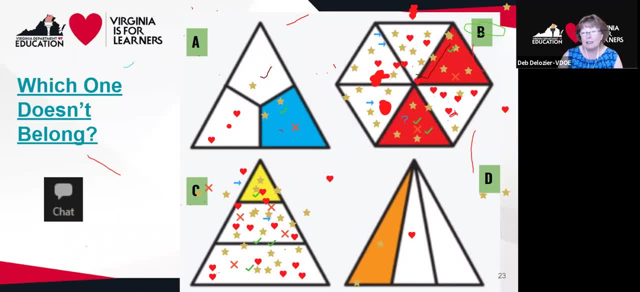 It has six sides. It's the only shape with six sides, But someone noticed it does have internal triangles, right? So nice observation. So we would go through this In my classroom. I use this quite a bit, But what I often did was take. and cut the shapes out and put them on different poster boards, sticky notes. you know everything with different shapes, But what I often did was take and cut the shapes out and put them on different poster boards, sticky notes. So we're going to go through this and we're going to go through that. So we're going to go through this, And then we're going to go through this, and then we're going to go over the shape hosts, which three weights, The components of thisoidеый edge. This is a really unique one as well. 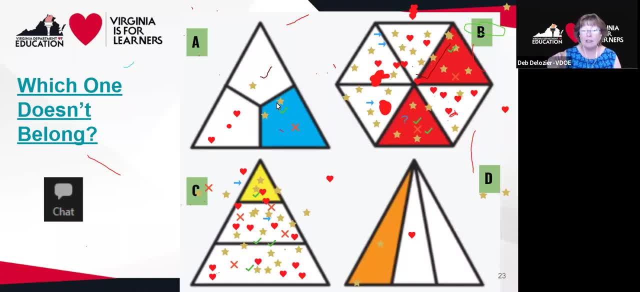 How does it basically come from a Herausforder, Theort, mangled, overweight website by young American sticky notes or whatever. And I have the kids write on a sticky note which one they felt didn't belong and their reasoning, And then they would take it and place it beside of the shape. So you 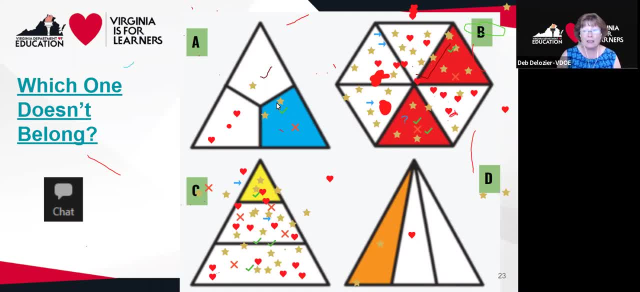 could see how you can do this electronically, in this case how we've done it here, but also how you could do it in a classroom. Routines like this are really great as a way to activate or to bridge to prior knowledge to the current grade level content, And you can do this all in five to 10. 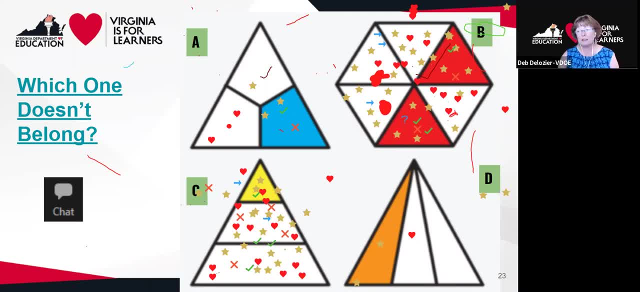 minutes, But there are lots of benefits, of course, for using routines like this. One, of course, is that all students have an entry point right. Is there not a reason for each of these to not belong, as long as the reasoning is correct, right? The one thing I like, though, about this particular 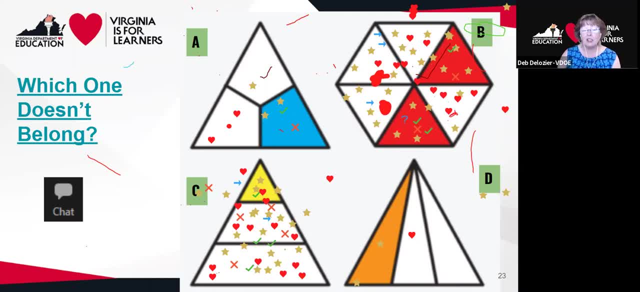 which one doesn't belong activity is the discussion that we can have around C about why, Why it doesn't belong. And C, as Carol pointed out, does not have equal parts within the whole. And, Carol, I know you're a classroom teacher And I know that you probably have kids particularly. 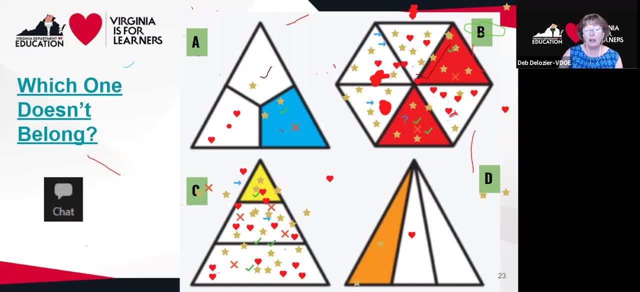 at the beginning of the school year. who might struggle with this? I know I did. I was a third grade teacher at one point in my career And some students would have said, well, that's a third. So it's correct too right, They're all thirds And that this was a third. But 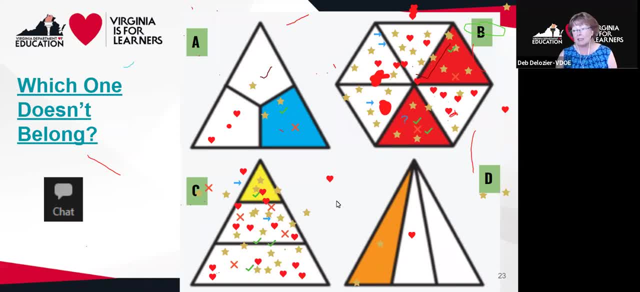 they're all thirds, And that this was a third, And that this was a third, And that this was a third, And they're having to think about, well, how can I prove it? Or the teacher might be asking things like: how can you prove it? So it's a great way to address misconceptions. Oftentimes a number talk. 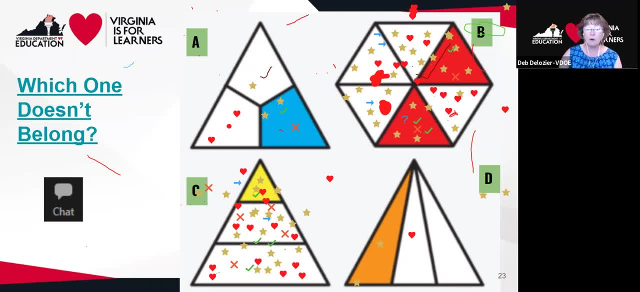 or a routine such as this will allow for great discussions around vocabulary and a chance for the teacher to address any misconceptions that students typically have, in this case around fractions. So when you get the link to this to the entire PowerPoint that we're sharing today, 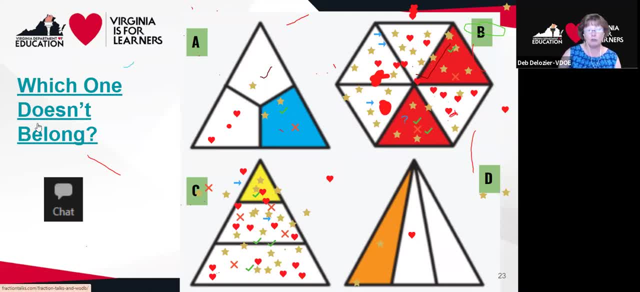 the link that I've included, for which one doesn't belong, actually takes you to the fraction which one doesn't belong, where there are lots of fraction examples that you can utilize in your classroom. So we wanted to get us thinking mathematically a little before we moved on. 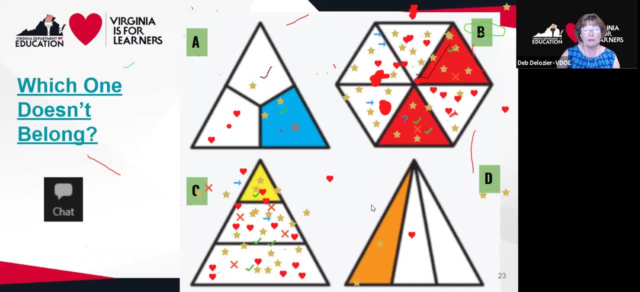 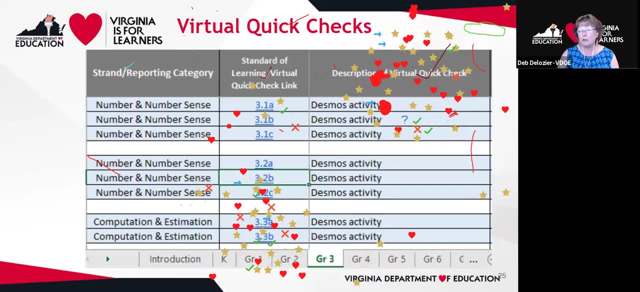 So let me go ahead. Well, kind of go way too fast, Let's try that again, All right? So now we'll take some time to step back into the use of quick checks as a tool for determining student understanding, And many of you know that in the spring of this year we had a team of Virginia teacher leaders. 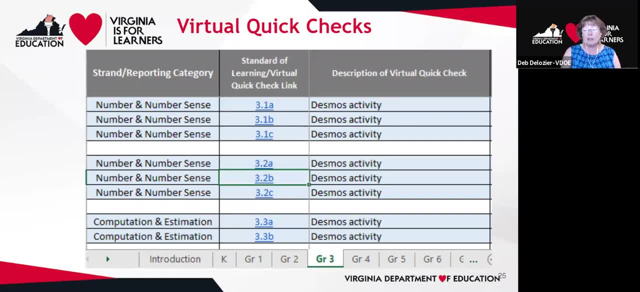 assist us in vetting the virtual quick checks that had been developed by many folks around the state. And those vetted virtual quick checks are now available And Kristin is going to put that link in the chat, But on the screen you can see that I have a picture of the spreadsheet. This is what 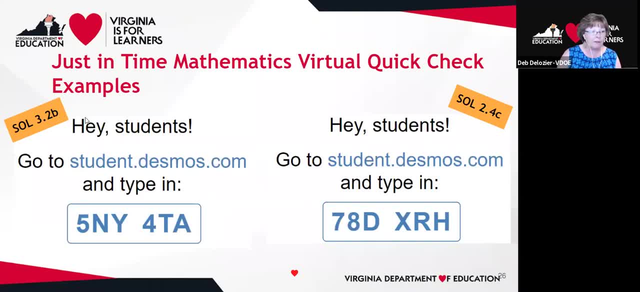 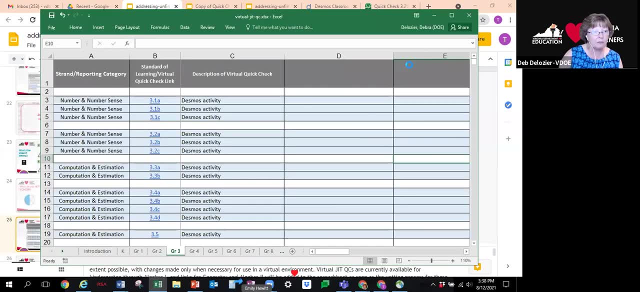 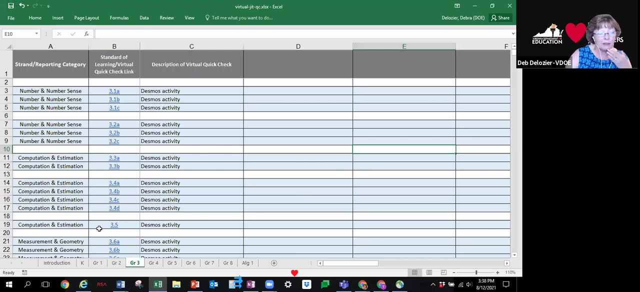 the spreadsheet looks like- And actually I'm going to just get out of here for just a moment- I can stay on the right page and take you to the actual spreadsheet. So I have the spreadsheet on my screen And you can see- for those of you who aren't as familiar with Excel- at the bottom of the page. 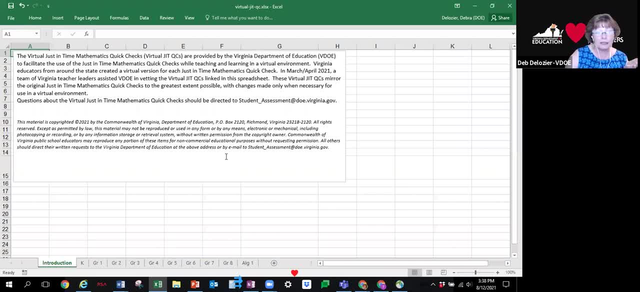 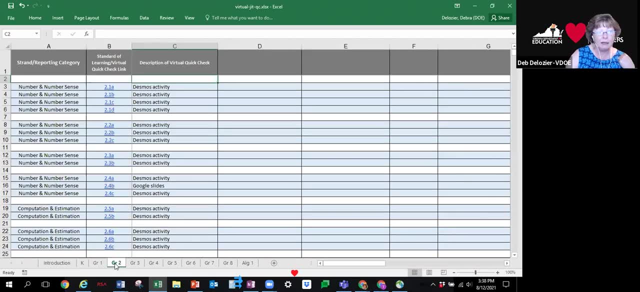 I can go to the introduction which talks about how these were created. But then I can click on my grade level. So, say I'm a second grade teacher. I can go to the grade two tab and then you're going to notice that all the quick checks, the virtual 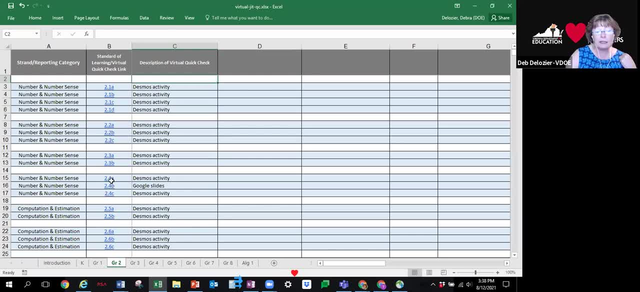 This is the list of the virtual quick checks are listed here. Then I can click on any one of these. that will show the content that I'm looking for for that particular lesson, or if I'm planning for next week's math lessons, et cetera. 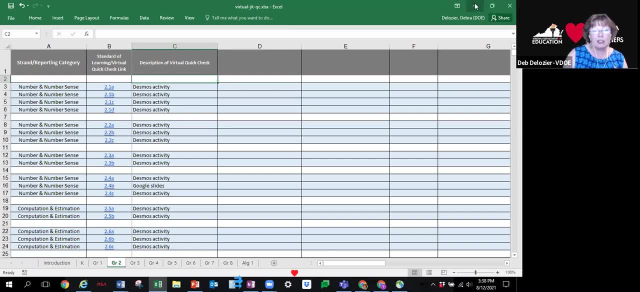 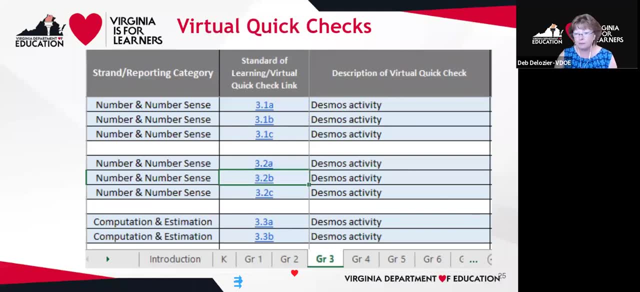 And we're going to take a look at some of these, But we did want to kind of share that with you. But for the moment, we're going to actually dive deep into one of them in just a moment or two, So let's take a few minutes to actually experience one. 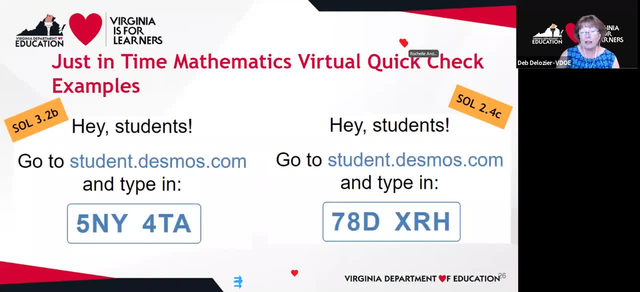 OK, And I'm actually going to show you a little bit of what that looks like. OK, And I'm actually going to ask that you do one of the two that I've shown on my screen. We're going to actually go to Desmos, to the Desmos website. 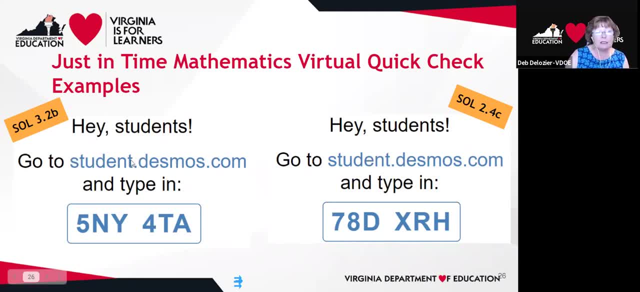 So on your computer, if you'd go ahead and type studentdesmoscom And then when you get there, we're going to look at either SOL 3.2B, the activity associated with that, and the way that you get there is then to type in the code here, or if you're a primary teacher and you would like to 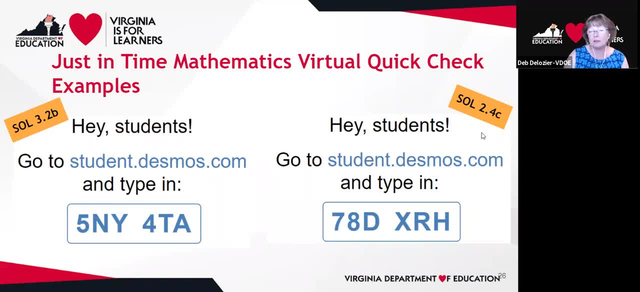 look at a primary skill, but an associated skill to the to the representing equivalent fractions we were talking about earlier. for grade four, you could look at the 2.4C activity And here is the code for that one. So we're all going to studentdesmoscom and then typing in one of the two codes. 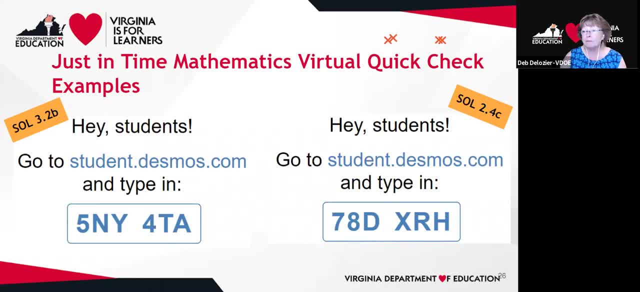 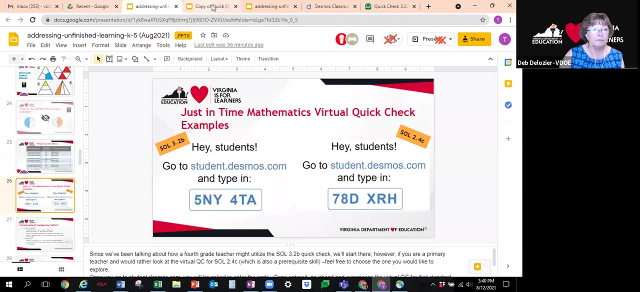 And you're going to try out that activity, And I'm going to give you a moment to do that, and then I'm going to go to the web page where you're going to be able to. Well, I'm going to take you through the teacher aspect of looking at this. 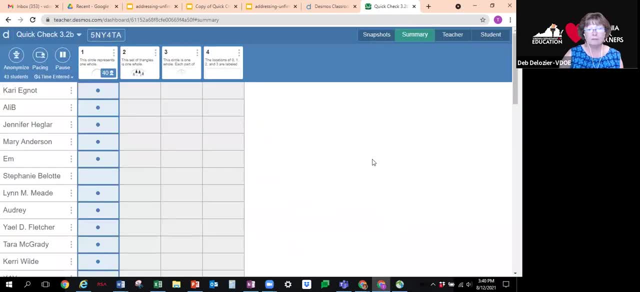 I'm going to be quiet for just a moment or so so that you can work your way through this particular virtual quick check. But when you're ready, or if you've not been able to get into either one, go ahead and take a look at my screen so that you can see what the teacher sees. 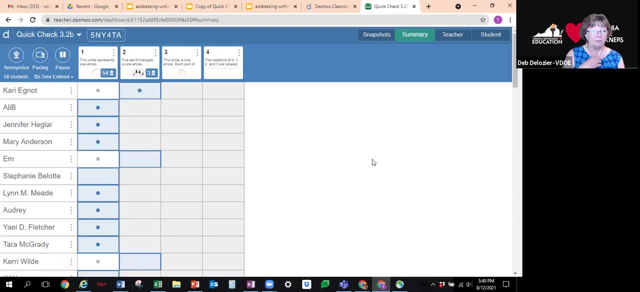 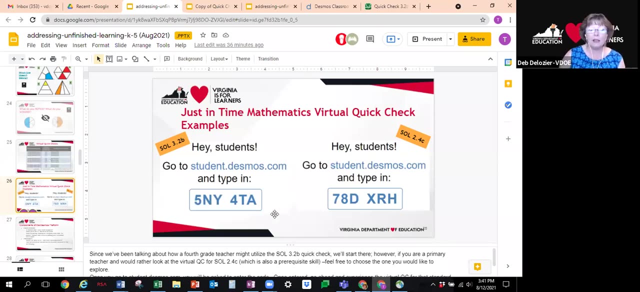 And I'll talk you through some of this in just a moment. Okay, All right, Thank you. I put the code back up on the screen so those who might be struggling could see that. I put the code back up on the screen so those who might be struggling could see that. 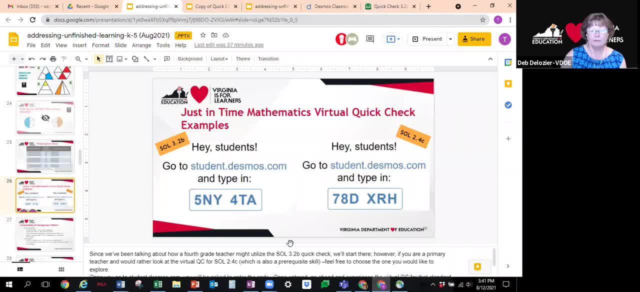 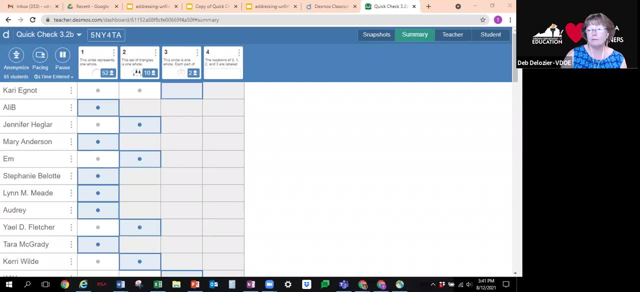 Okay, So again, I'm going to go ahead and type it in, All right. So one of the cool things about using Desmos, even in the elementary school, is that, as the teacher, you can see students as they're working through the activity. 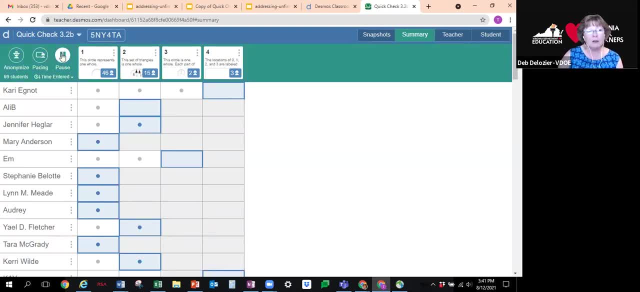 So I'm actually going to press pause And so you might notice now, if you're working in the third grade activity, that I have paused the activity and you can't work just now until I unpause. So I'd like you to kind of go back and look at my screen for just a moment and I'll let 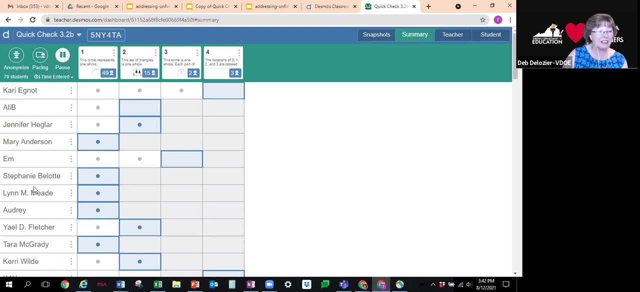 you continue after I talk again and kind of explain some of the pieces here. Okay, so you can see the people, the folks that are in the class. Hi Lynn, Hi Carrie, Hi Jennifer. Good, Great to see you. 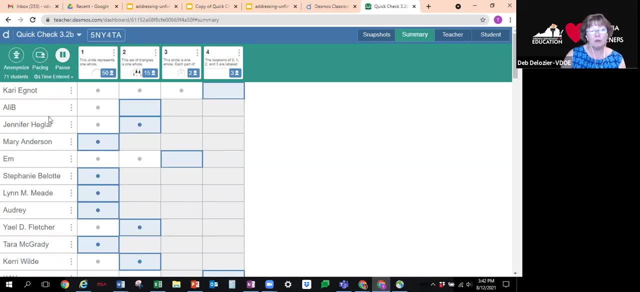 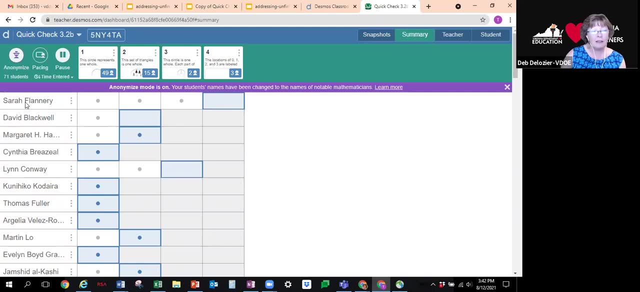 But maybe I, as the classroom teacher, don't want my students to know who is where and what their work looks like, So I can make everyone anonymous by clicking this button here. So now they have these nice cool names and no one really knows who they are, except that 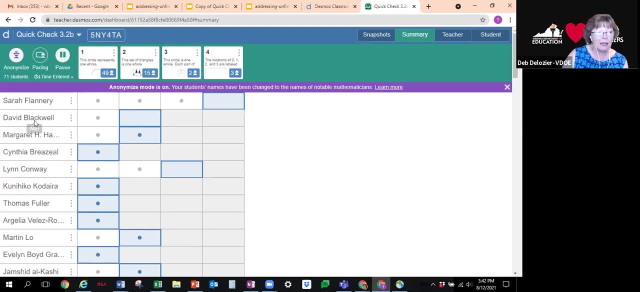 I can go and see. You can see, David Blackwell is really Alebe, Cynthia Rizil, as usual, is actually Mary, But the students don't know. And that is a nice feature. because what if I want to sort of highlight something that? 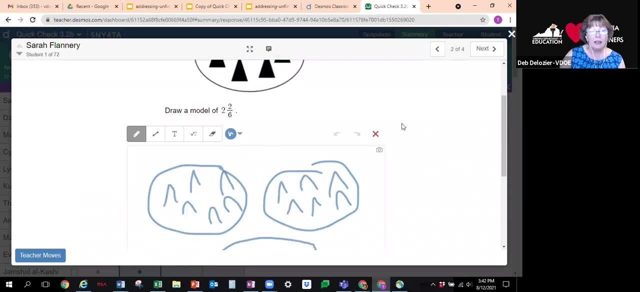 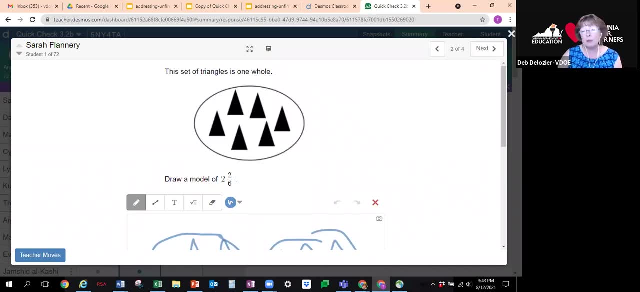 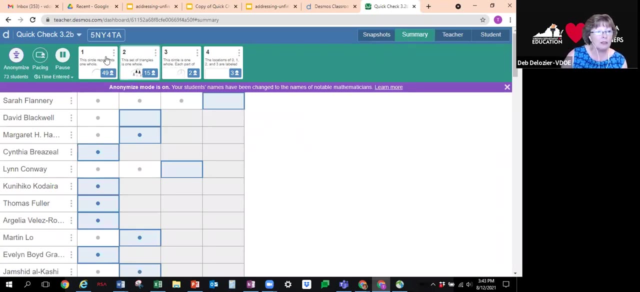 Sarah has done. Okay, I can go and see exactly Sarah's drawings And we can have a discussion as a class, or I can just be using that information because I'm checking for student understanding. I can also go to a particular question. 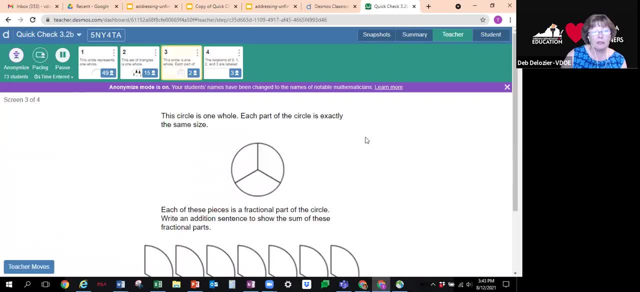 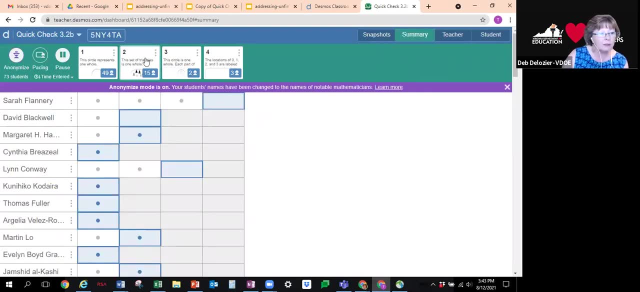 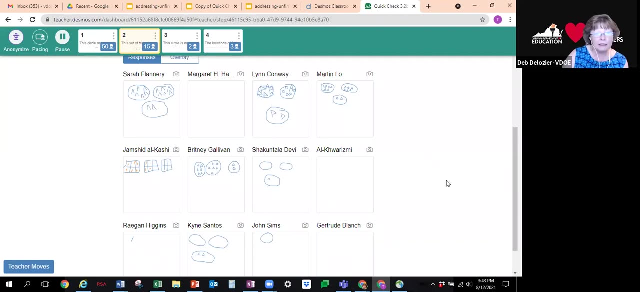 So let me go to this one here, And if I click somebody, no, that's not what I wanted, That's this one, Yeah. So notice, if I scroll down, I can see everybody's drawing And I can see that Margaret hasn't had a chance to start yet. 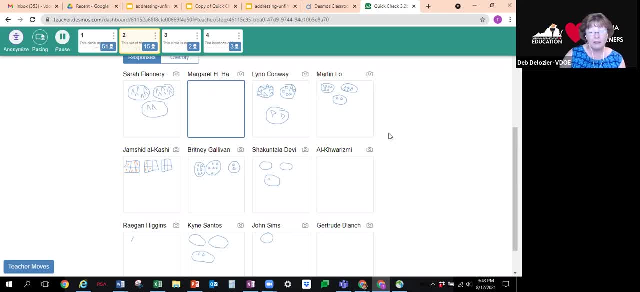 Maybe that's because I paused before she had a chance to do this one. Okay, But I can see all my students' work in a snapshot. You can't do that normally in a classroom, right? Normally you're trying to walk around, you're trying to look at everybody's work. 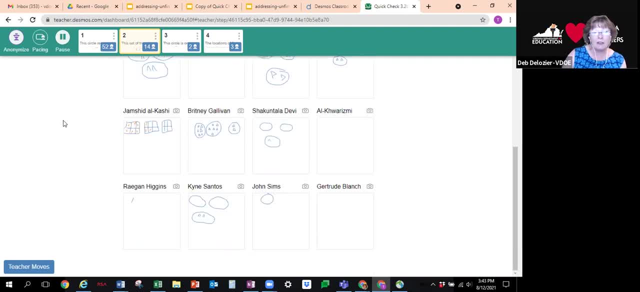 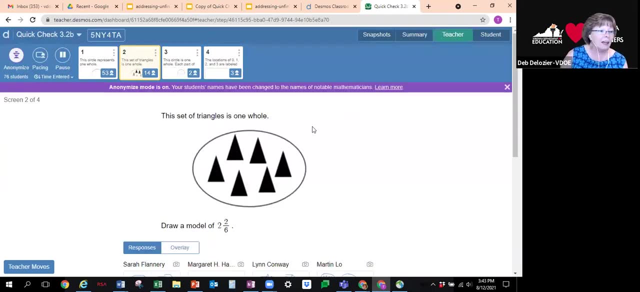 But look how quickly I can see where my students are and how they're doing, So that's kind of a cool thing. So I've unpaused you. If you're wanting to continue, If you're wanting to continue to work, And if I want to look at the activity from the student perspective, I can click just. 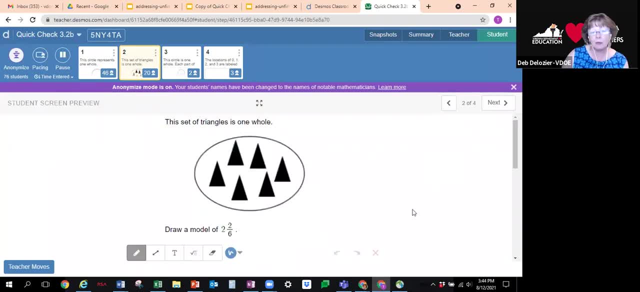 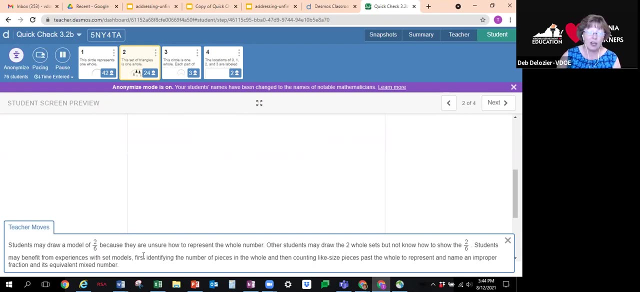 on the student and I can scroll down and see exactly what the students see when they look on the screen. The other cool thing about using Desmos in the virtual QuickCheck versions is that under teacher moves we've added the teacher notes from the actual QuickCheck. 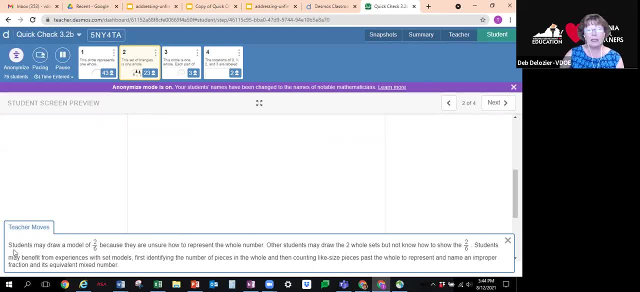 So remember, if you've been utilizing the QuickChecks, that they can take a look at the actual QuickCheck. The teacher notes in the manual will contain common errors and misconceptions And that's where you'll find this information is under the teacher moves. 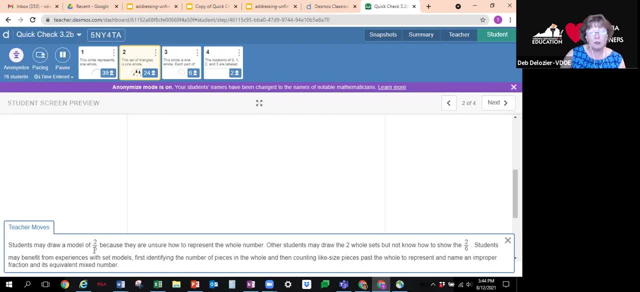 Okay It talks about. students may draw a model of 2-6 because they're unsure how to represent the whole number, or other students may draw the two whole sets but not know how to show the 2-6, right- Different pieces that students might struggle with. 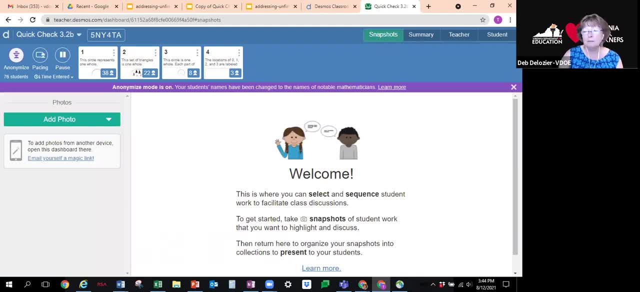 So those are some of the cool features. Kristin, did I miss anything? No, Um, I'm not sure if you mentioned this or not. Did you get? the other neat thing about it is you can, after your class is finished, and say you didn't have a chance to look at how everybody 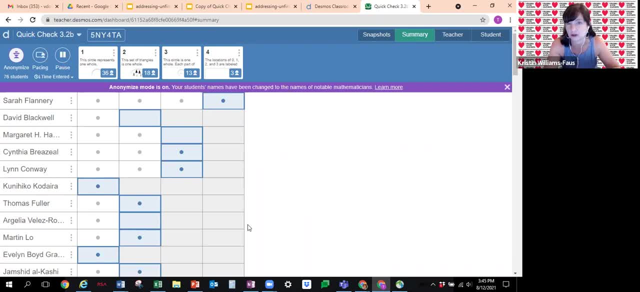 did, or look at their work and so forth. you can go back to the teacher, the teacher dashboard, and it saves all the work, which I think is a really nice benefit as well, especially when you're thinking about your planning for small groups and who needs what in terms of instruction. 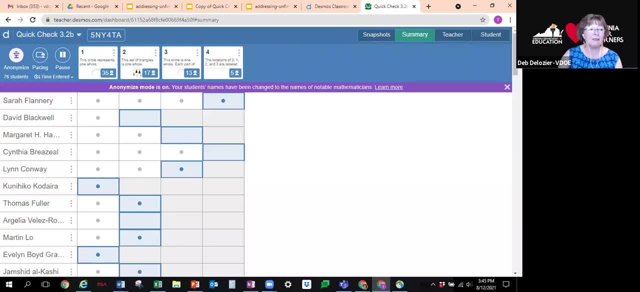 Thank you for bringing it up, because it was interesting, because this morning I went back to look and I said to my from yesterday's session and I said to myself: why were there only 75 people there? And then I remember that I had given two choices, And so 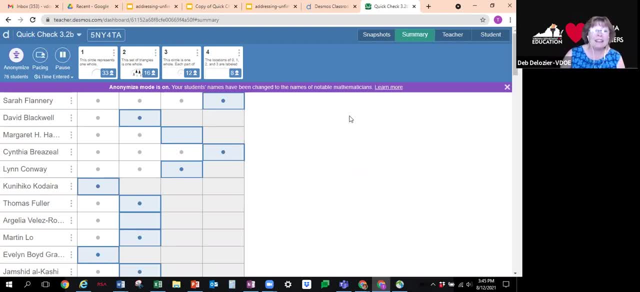 there were 60, some people or so in a second grade version, but I could go back and see the work that everyone had done. So it's really it's really nice, And so you know, sometimes I think as elementary teachers. 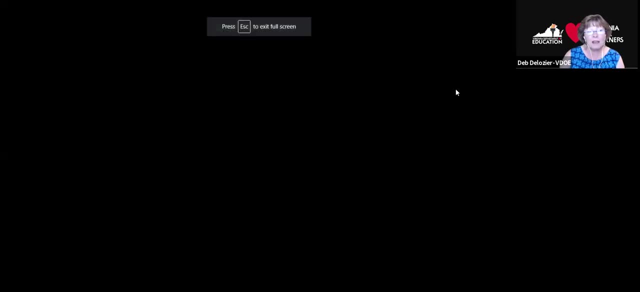 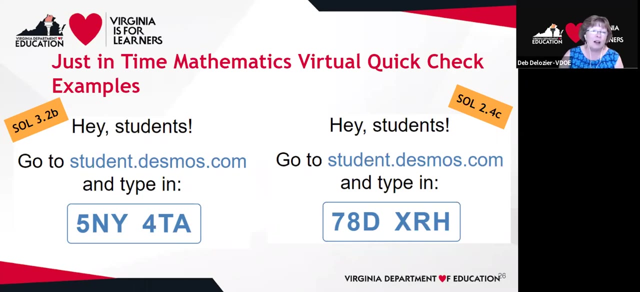 we think that the decimals is just about the calculators, because that's how we initially heard about it, if you recall. But now we recognize that it has so much to offer us instructionally as we work with our students, So we wanted to be sure to kind of give you that. 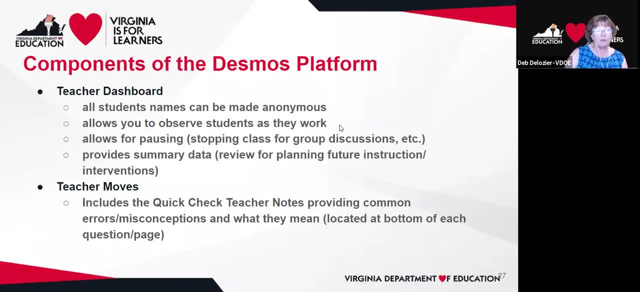 opportunity to explore it if you've not had a chance to explore it before, And on this slide that you're seeing now, it's just really showing you some of those components that we talked about: the making the students anonymous, being able to observe. 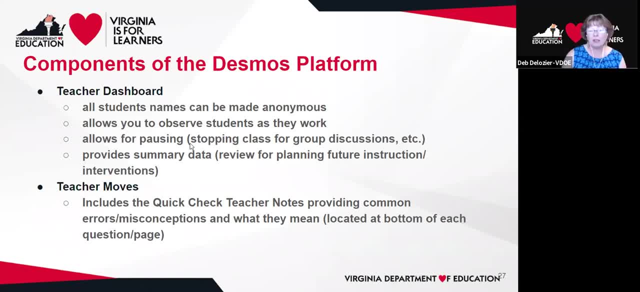 student work. using the pause feature, you might want to pause so you can have a conversation with students before they move on. There's also a way that you can stop. you can say: I want them to do activities one and two, and then I want them to stop until I release the rest. So so those are. 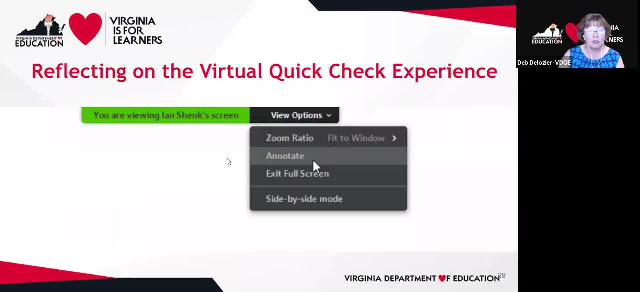 all really nice features and ways that you can utilize that So so I was looking for this slide earlier And I guess we didn't put it in both places, But this is a reminder of how to use the annotate feature, because we're going to ask you to reflect on the virtual quick check experience and 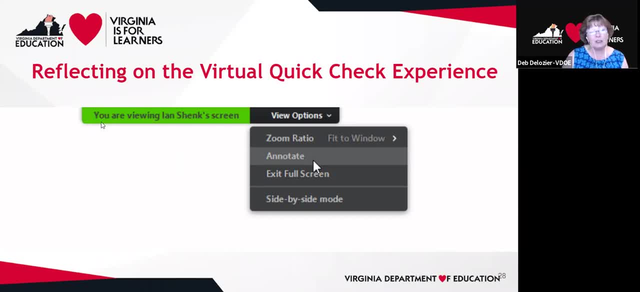 some of your favorite pieces. So remember, at the top of your screen you should be seeing you are viewing Deb Delozier's screen And then, under view options, if you go to annotate, you should be able to go to a stamp And we would like you to select one or two of your favorite aspects or 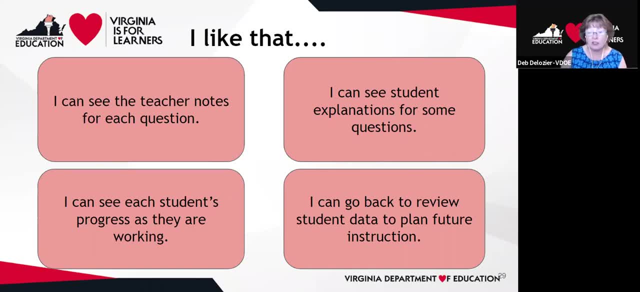 favorite things about Desmos, now that you've actually had a chance to explore it more. And again, if you don't have the annotate feature, please add your ideas or your thoughts in the chat. we'd appreciate that. So Catherine says: I can see other stories that you can use, So I'm going to go ahead and go ahead and 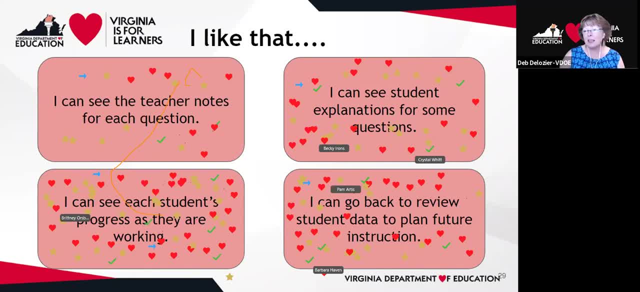 start with the annotate feature And again, if you don't have the annotate feature, please add your ideas or your thoughts in the chat. We'd appreciate that, As you can see each student's progress. that is one of the best things, isn't it, Catherine? to be able to see. 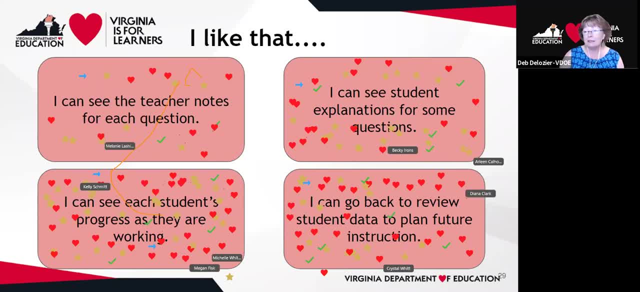 everybody's work so quickly too, And as they're working right, Jamie, that is really nice. You can see if someone gets stuck or appears to be stuck because they're not moving forward, So then you can check in with them And, of course, if you're working, 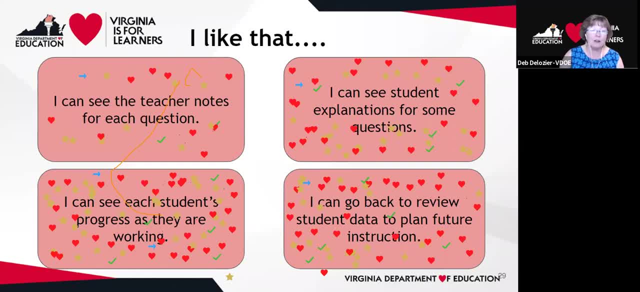 virtually. that's really great to be able to do that, because you don't always have that opportunity. We also have the snapshot tool, which is really cool because you can take pictures of different work And then, as you're doing your class discussions and your discourse, you can select and sequence the work, which is a 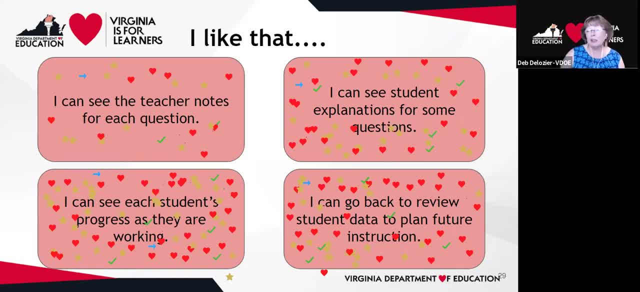 really cool feature, Lynn. I love what you put in the chat. You can easily determine groups of students to meet with based on need. Very important right, And we know that more than ever this year, we're going to have to be really alert to what our kids are understanding every step of. 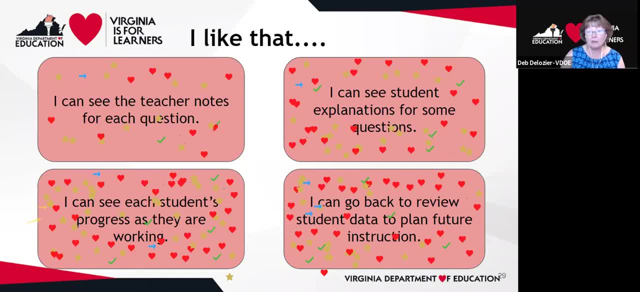 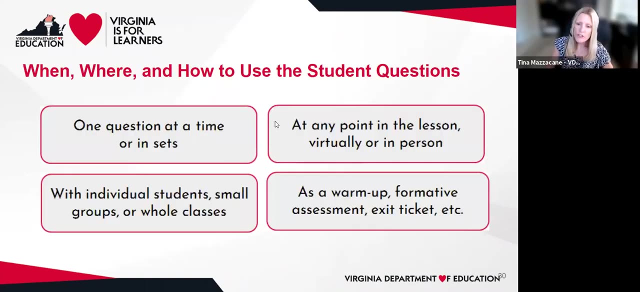 the way, so that we can try to intervene as needed along the way. So great ideas. You guys did a great job with that, So let me clear everything so we can move on to the next piece. Hey, Kristen, I think that you had mentioned too that another teacher could be added to the same activity, So 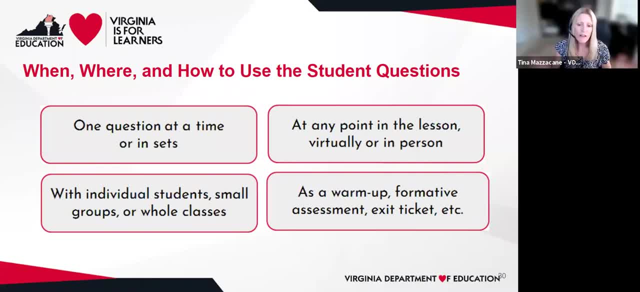 if you were team teaching with another teacher, you could add another teacher to the same activity. They could both look at the results. Is that correct? Yes, you can add. So if you're in a co-teaching situation, you know with a general ed teacher or special ed teacher, both teachers. 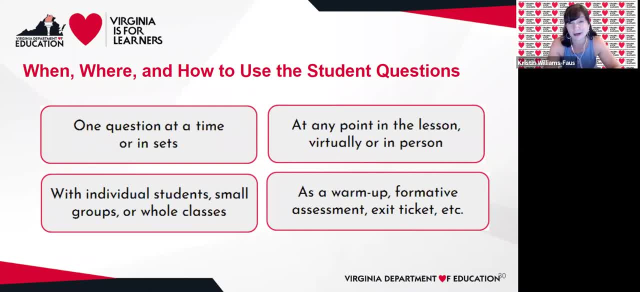 can be on the class, And another great reason to use this is it will help provide information for the special ed teacher in terms of progress monitoring IEP goals when you're forming your small groups, for your different co-teaching models, when you're doing your 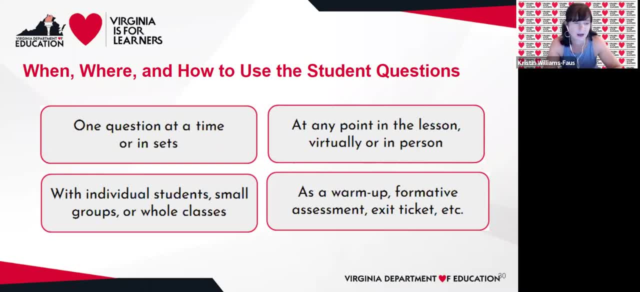 stations, your parallel teaching, your alternative teaching. So yeah, it's an amazing resource that really has a lot of benefits for all of our kids. Thank you for sharing that. That's really important if you're co-teaching- And I had the pleasure of co-teaching with a special ed teacher- 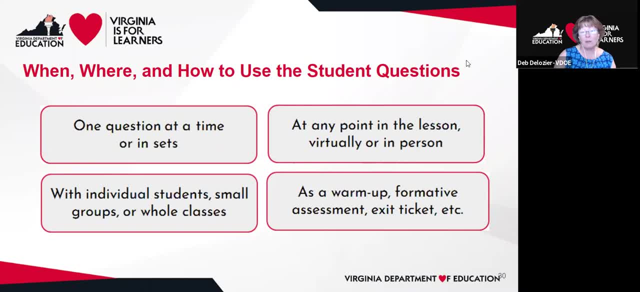 all year long. She came into my room and we co-taught mathematics And it was one of the greatest experiences. So you know we've shared with you the virtual quick checks and you've had to do that, So I'm going to turn it over to you Kristen. 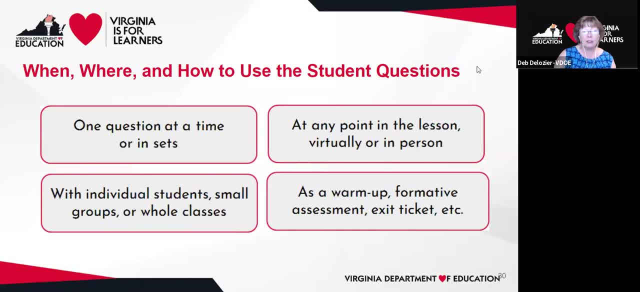 Thank you for having me. I'm going to turn it over to you, Kristen. So we did want to remind you that the quick checks were created to be very flexible. So in thinking about when, where and how you might utilize them, we just want to make sure that everybody is aware. 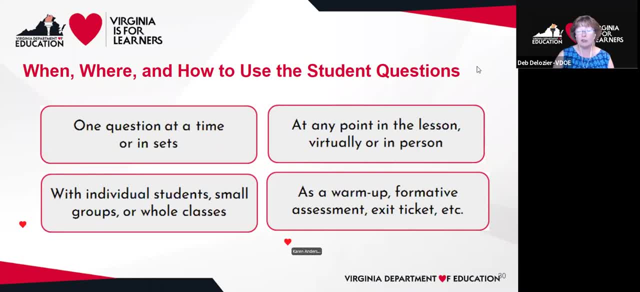 You can take one question at a time from this set. You could use it as a warm-up or an exit ticket so that you could have that information and planning for your lesson the next day, Or you could utilize it at any point in the lesson, either virtually or in person. 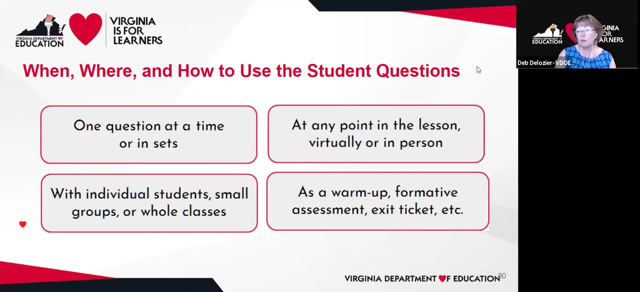 You can utilize them with individual students or small groups or your entire class. We just did an entire quick check with the whole class, So I kind of modeled that, but you don't always have to do it that way, right, And, as I mentioned, you could use it as a warm-up and 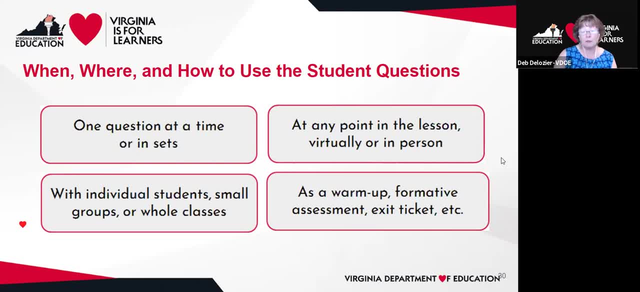 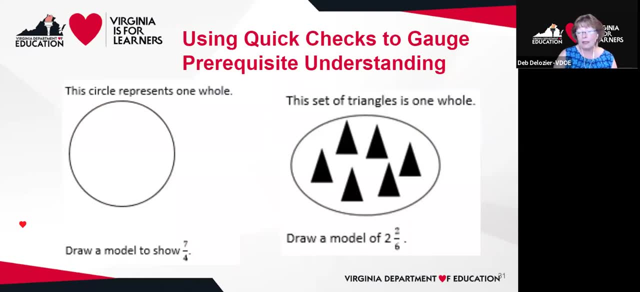 certainly formative assessment is going to be extremely useful to you as you move forward, helping students In terms of thinking about additional ways. an example that would be a teacher utilizing the quick check or questions to connect prior knowledge with current grade level. grade four content could be at the beginning, So she might use one of these questions. 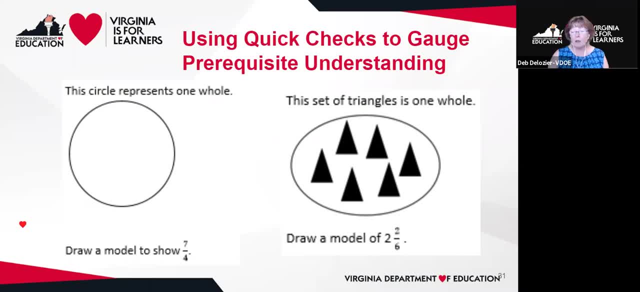 to kind of see where everybody is in their understanding. I used whiteboards a lot in my classroom and perhaps you do, or you use something very similar. You know students had their own whiteboard so they were able to represent this individually and show it to me. because you don't always have to do it. You can use it as a warm-up, but you don't always have to do it individually and show it to me, because you don't always have to do it. You can use it as a warm-up. 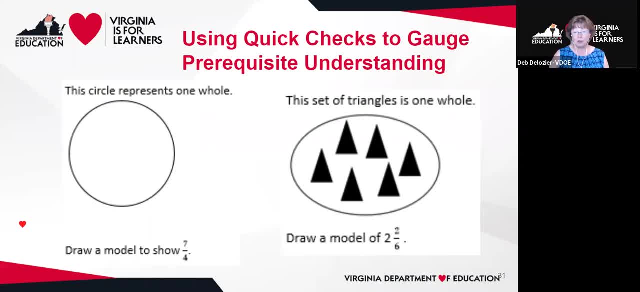 but you don't always have to do it. You can use it as a warm-up, but you don't always have one-to-one computers where students could do the virtual version. So we just wanted to be sure that you're thinking about all the ways that you might be able to utilize these moving forward, One of the things we want to make. 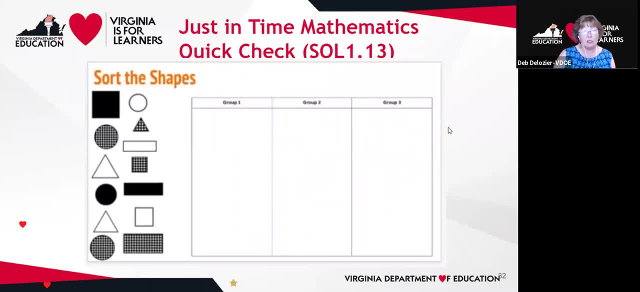 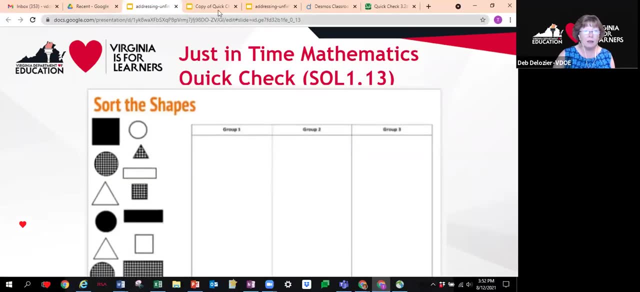 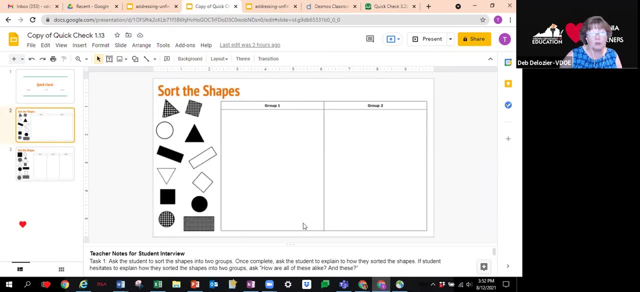 sure that you know, for our early grade teachers in particular, is that most if not all whoops, most if not all of the kindergarten and first grade quick checks are in Google Slides, And so I just changed to the Google Slide for SOL 113.. Okay, so this is a first grade quick check, virtual quick. 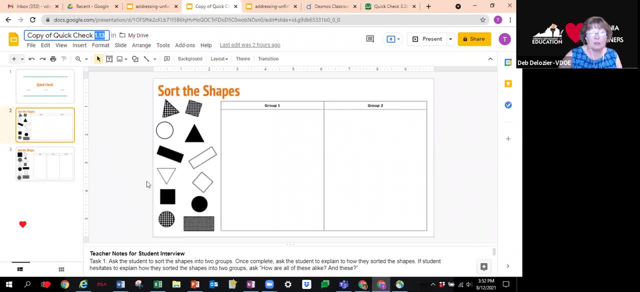 check, And here I can have my students sort. this is the sorting by attributes standard, And so students can manipulate the shapes and do sorting however they decide what the criteria is going to be right. So I think you all figured out what my criteria is, But another student who has the same slide. 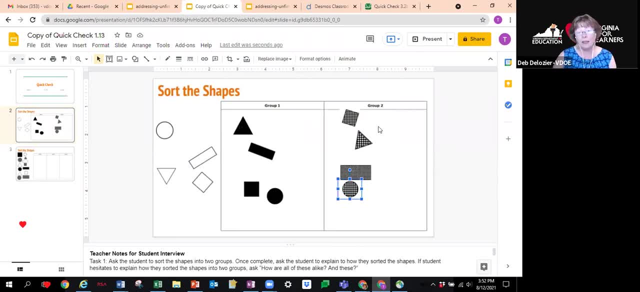 could be sorting by triangle someone, or straight edges, right No sides, So my circles would be on the one group, So there are lots of ways that they might be sorting. The interesting thing, or nice benefit rather, is that the teacher notes are included in the 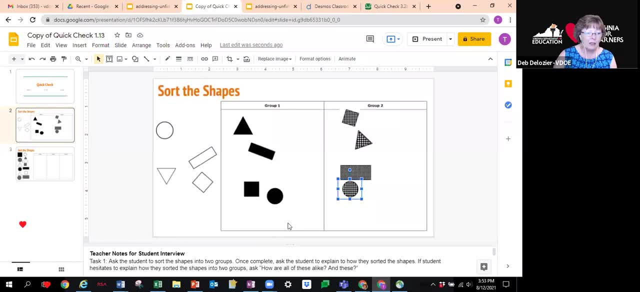 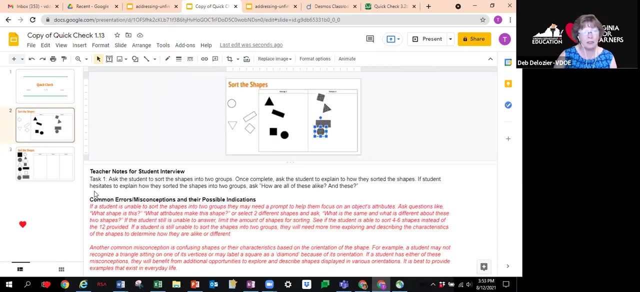 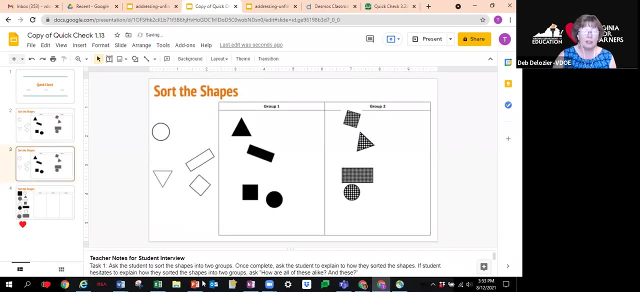 presentation notes section. So they're all right here for the teacher to look at, And if you've ever used Google Slides, you know it's extremely easy to duplicate the slide, So I can do that over and over again When you click on the standard in that spreadsheet that I shared earlier. 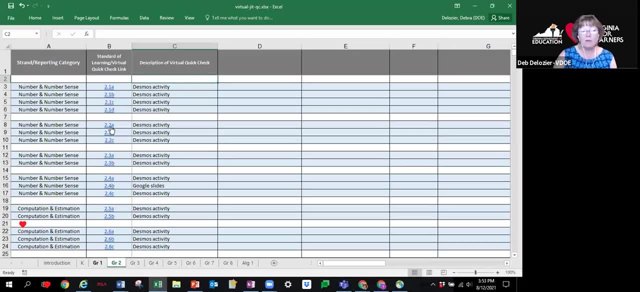 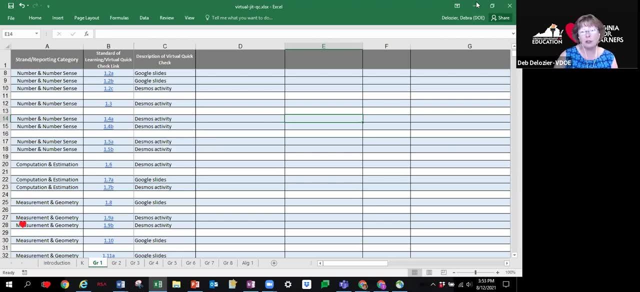 when you click on the standard, if I'm in first grade, it's going to force you to make a copy. It automatically will come up make a copy and you just click that. it makes a copy in your slide. It's going to make a copy in your Google folder, So I just wanted to share that feature with you. 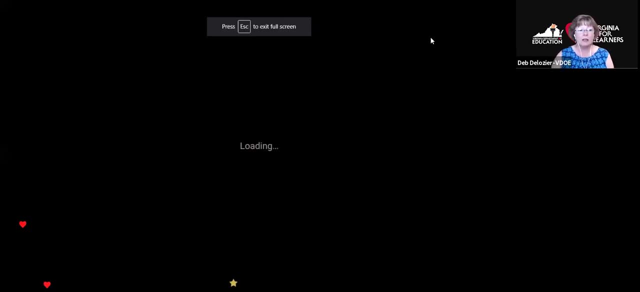 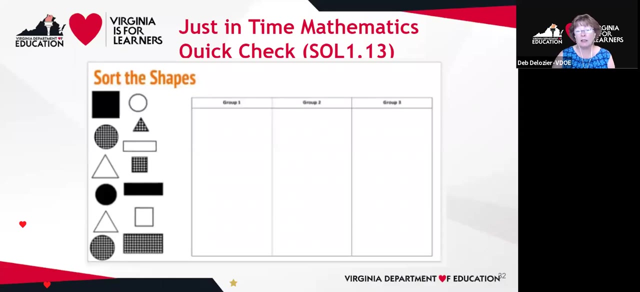 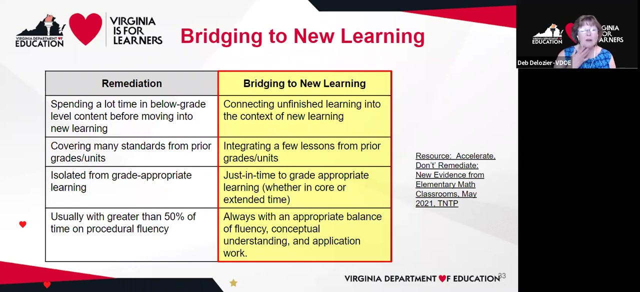 because many of the kindergarten and first grade quick checks were developed in Google versus Desmos. But there are some, and especially starting at second grade on up, most of the quick checks you'll find in Desmos. But we're going to talk a little bit more about some of the primary. 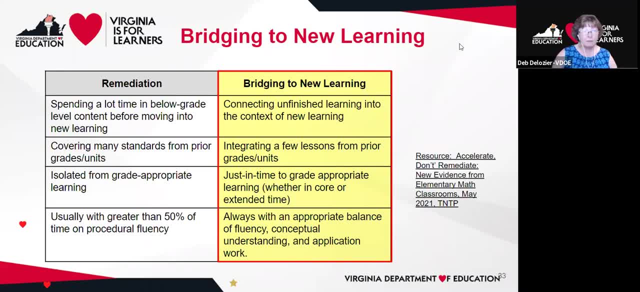 activities that you'll also find in Desmos moving forward, All right. So getting back to this idea of bridging to new learning, We know that this year is going to have its challenges, but we also know that the research is clear. It's clear that creating a bridge between 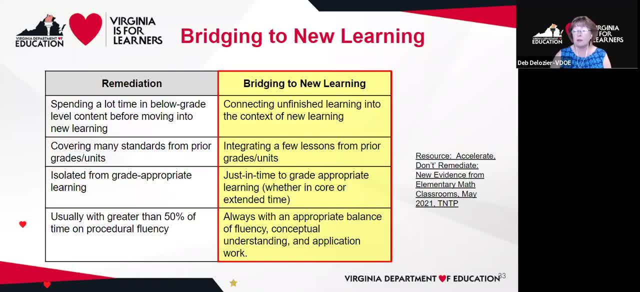 prior concepts and the new concepts at the current grade level are going to be key. So, for instance, we keep talking about this fourth grade teacher. The fourth grade teacher, for example, is going to need to start with fourth grade content. You're not going to have time to go back and redo all a. 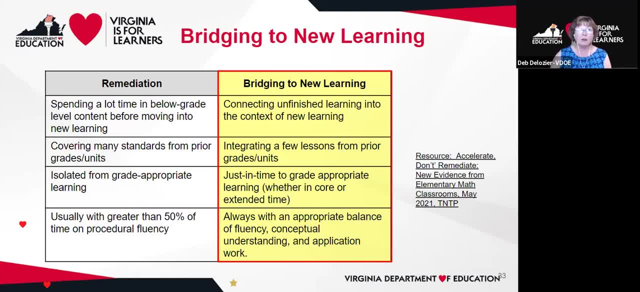 third grade. that you've done, So you're going to have to start with the fourth grade. content You think might be lacking or that kids might not have had sufficient time to learn right? So you're going to. the research is telling us we must start with the current grade level content. 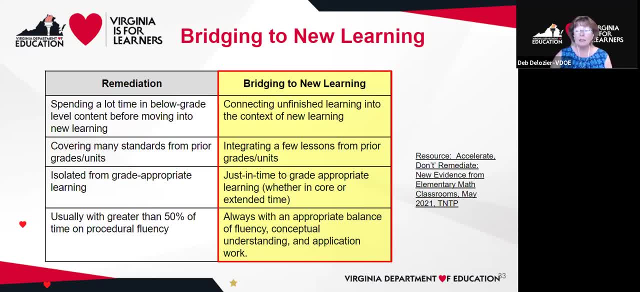 but then we have to strategically build in key third grade concepts when students might need them. Hence that just-in-time idea in order for them to master grade level work. The just-in-time teaching ensures that students spend more time on their grade level work. 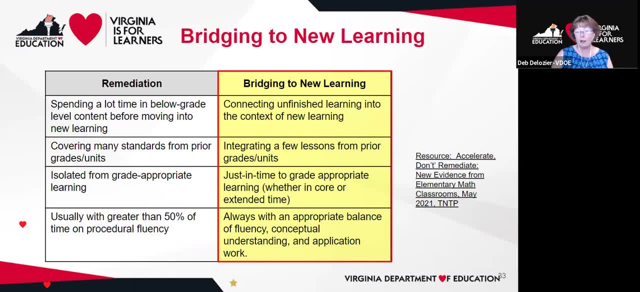 And key, of course, is ultimately to get to grade level if they're not already there. The TNTP report that we mentioned is linked here on the screen And, as we mentioned earlier, you'll get a copy of this presentation, But it mentions and provide and not mentions. 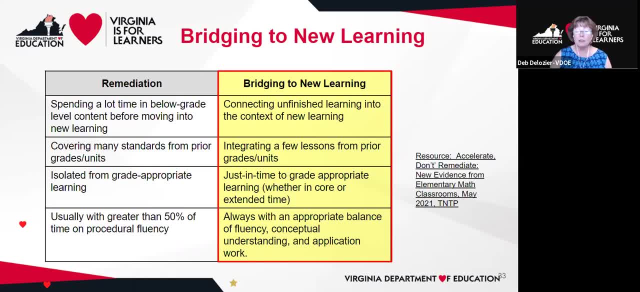 rather, it provides strong evidence that learning acceleration, not the traditional approach to remediation, should be the foundation of school systems plans in helping kids. So I think that's one of the key points And I think that's really important to have a look at as well. 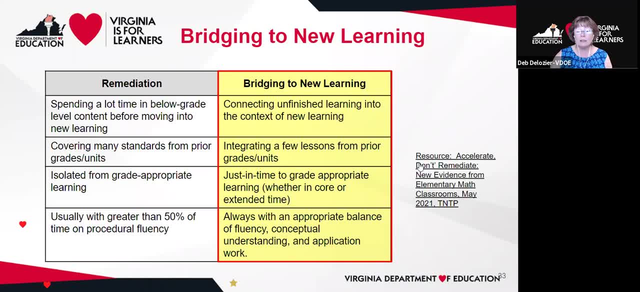 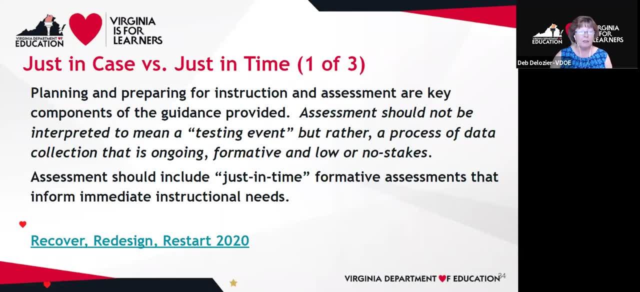 And this is where we kind of have to clarify the difference between the concept of just-in-time and the concept of just-in-time, And I think part of that is you can also see that when we talk about this fact that we need to have classes that are held in a specific time frame, 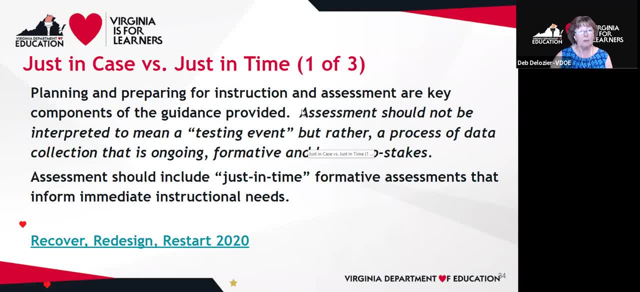 where you have classes that are elegant currently and we want to have a time frame that's in a specific time frame. So see that this in-time version of the four grade system, this method that we're using, is going to be that type of course that we're talking about. 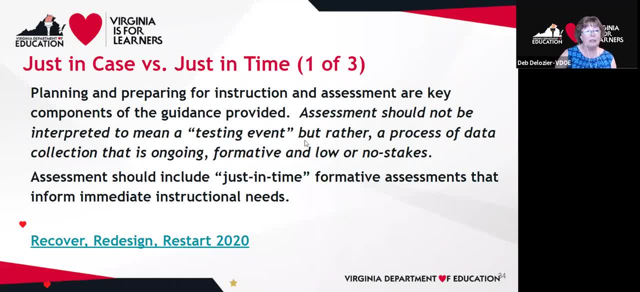 and it's going to be a whole different type of course, right? So it's really going to be a whole different forty-five-year process. So these are the ways to how assessment should not be interpreted to mean a testing event, but rather a process of data. 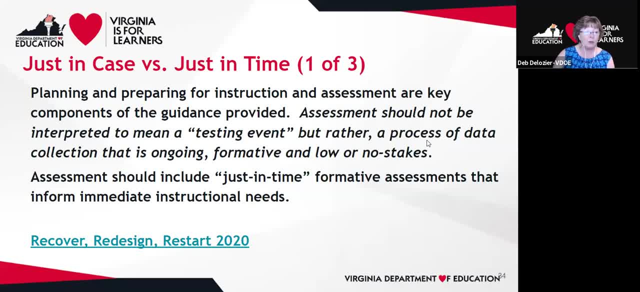 collection that's ongoing, formative and has low or no stake. That's what the just-in-time quick checks were created for: to allow you to formatively assess payments to plans. So let's give an example, or show you an example, of this idea of just-in-case versus just-in-time. 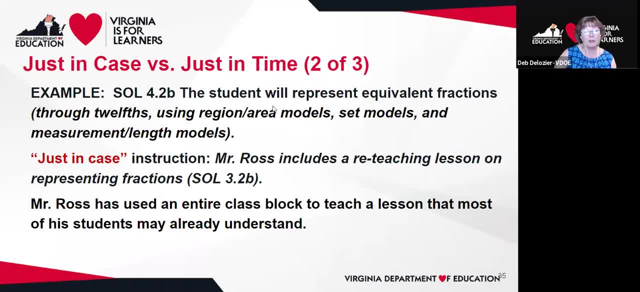 So remember we started out our session today talking about this standard. 4.2b Students will represent equivalent fractions. Of course, you know the limiter is right here. So an example of just-in-case instruction would be Mr Ross. He includes a reteaching lesson on representing. 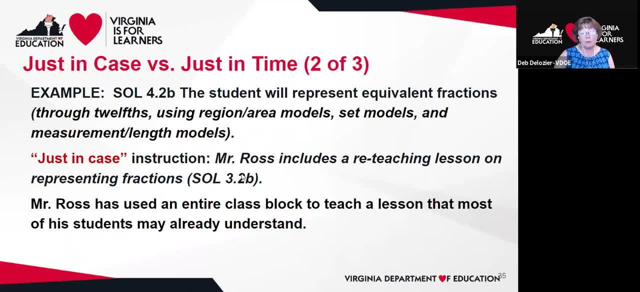 fractions representing fractions with models and symbols as part of 3.2b. He uses up an entire class block time to teach a lesson that most individuals don't know how to do. He uses up an entire class block time to teach a lesson that most 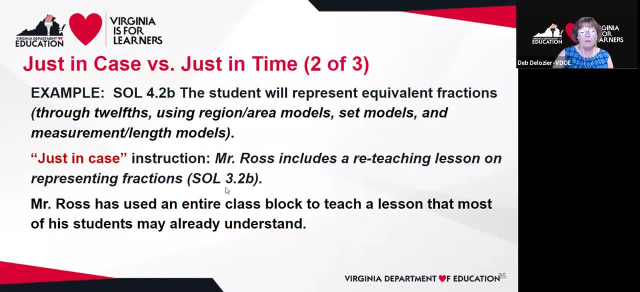 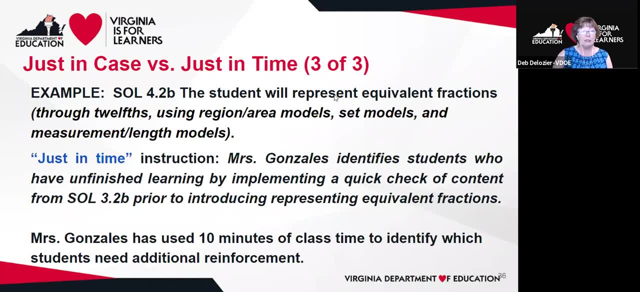 individuals don't know how to do. He uses up an entire class block time to teach a lesson that most of his students may already understand. Where we have Mrs Ross, she's getting ready to teach the same standard, representing equivalent fractions 4.2b. Instead, she identifies the students who 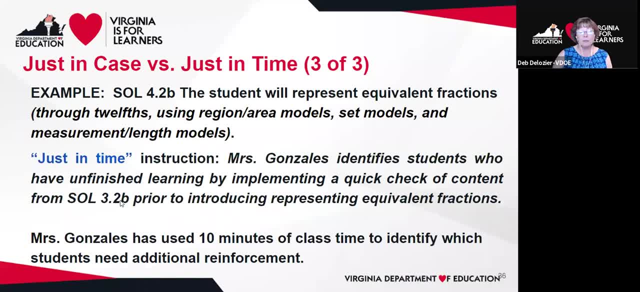 haven't finished learning. by implementing a quick check of content from 3.2b- maybe the one we just looked at right prior to introducing representing equivalent fractions. She wanted to know what understanding her students have of representing fractions. She wanted to know what understanding. 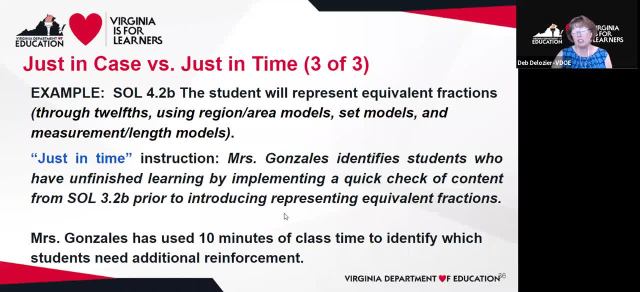 her students have of representing equivalent fractions. She wanted to know what she can use after she's done learning free action before she goes into talking about equivalencies, But she was able to. she's done learning free action before she goes into talking about equivalencies, But she was able to. 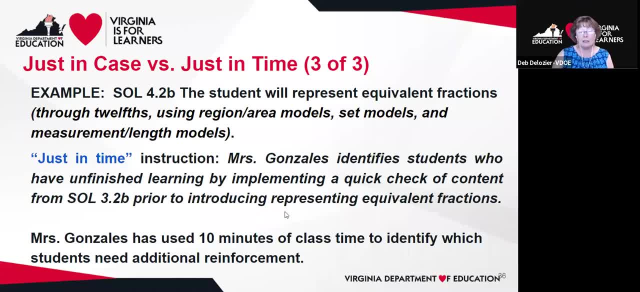 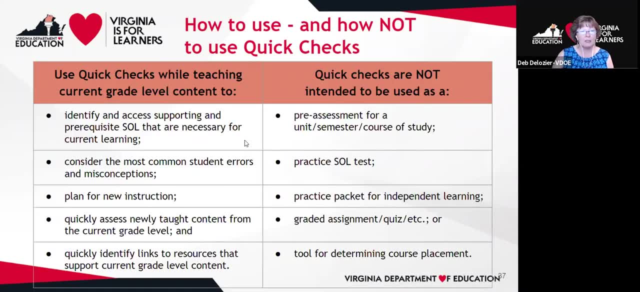 use up just 10 minutes of her class. She may have even utilized the routine that we tried earlier: use up just 10 minutes of her class. She may have even utilized the routine that we tried earlier. So we knew that the quick checks will be helpful to us in identifying and supporting prerequisite. 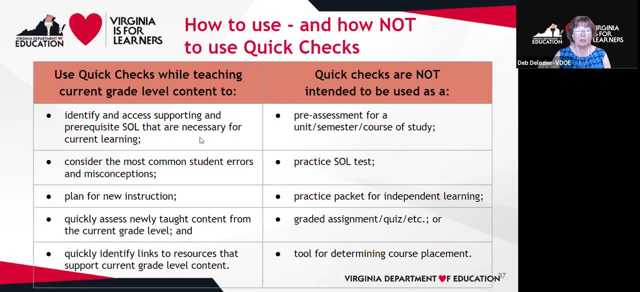 learning um. that really pinpoints what students are currently learning in class. We also know that helpful in helping us to consider those most common student errors and misconceptions. They'll help us plan for instruction and they quickly assess newly taught content. So I could use them. 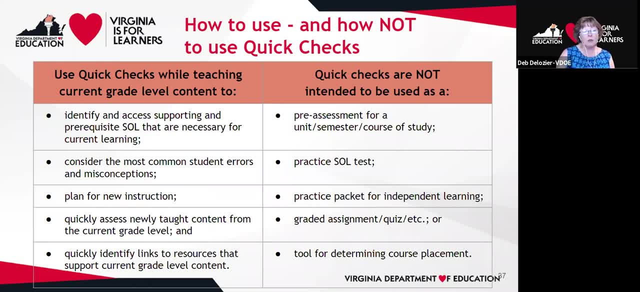 to see where students are in the current grade level content. They also quickly help us to identify links to the resources that support that current grade level. So we'll show you that in just a moment, in case you've not seen those resources. But they really were not intended. 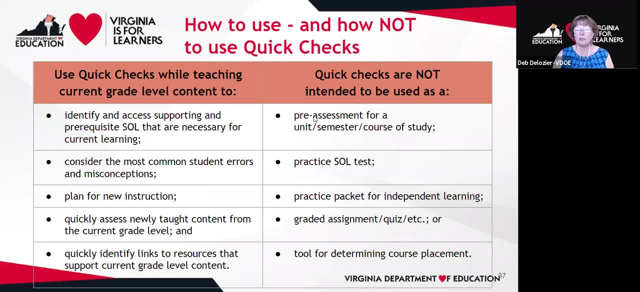 to be used as a pre-assessment for a unit semester course. So I wouldn't pull all the fraction quick checks together and give that to my students as a pre-assessment before I teach my fraction unit. right, And they're not really meant to be practice SOL test items. They aren't. 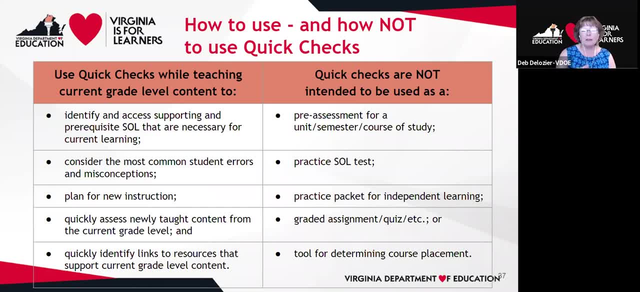 even written that way in many cases. They were meant to be formalized. They weren't meant to be formative assessments, So they weren't really meant as a practice test. They're not really meant to be put together, all these questions, for independent learning or to be graded. We really 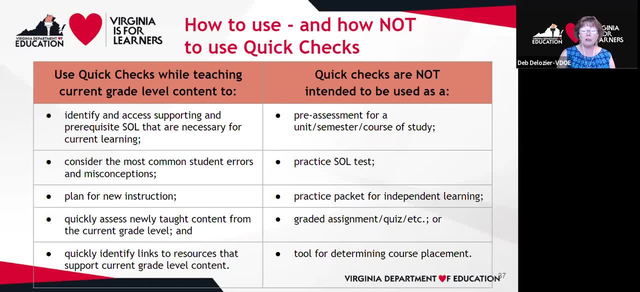 think that the best way to utilize these is for you to utilize them and understanding where students' understanding is. What strengths do they have? Where do they still need to grow? And then they definitely were not meant as a tool for determining course placement, So I wouldn't. 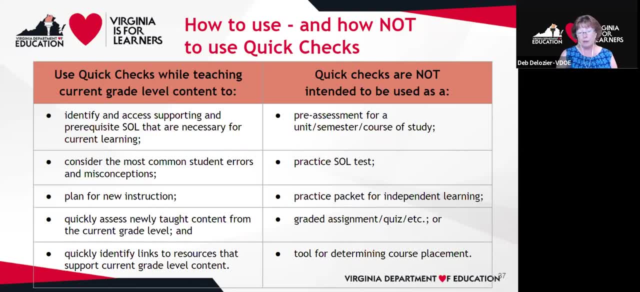 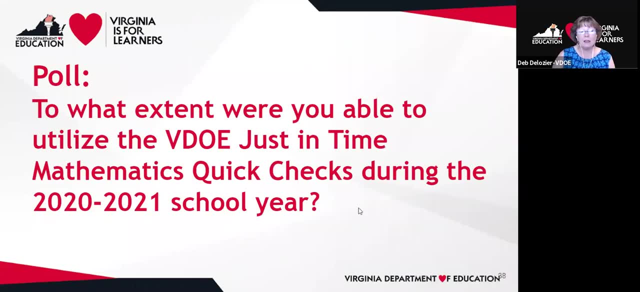 use the fifth grade, So we wanted to remind you of the great uses, And now we want to take a moment to give a poll and ask you to what extent were you able to utilize the quick checks during this last school year, And so you're going to have the opportunity to pick several answers, And I believe you're. 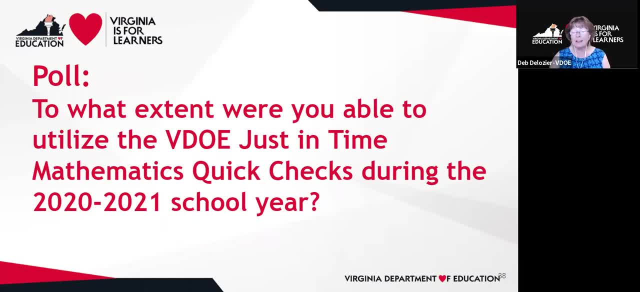 seeing the poll. Is that right, Kristen? Yeah, Okay, Everybody started, So you're seeing it. Yes, So click all. Thank you, Click all that apply. So you've used it perhaps as a pre-assessment to assess prerequisite skills. Maybe you've used it as a formative assessment to assess current grade. 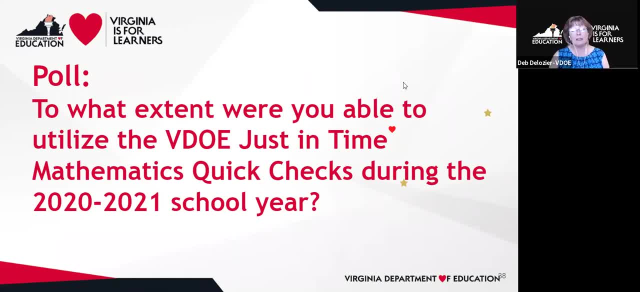 level skills, Or you've used it during planning for instruction, Or perhaps you're new to quick checks or you just haven't had a chance to use them yet. That's okay too, If you let us know that. it will help us to know where to go as we move forward and how to best meet your needs in. 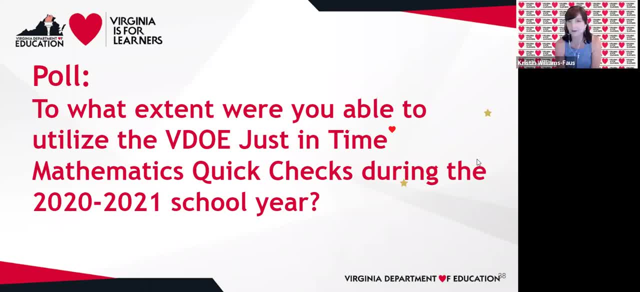 the rest of the session. We have about 60% participation so far, So we'll give it another few seconds. Thank you, Kristen. Getting close, sir, We still have about 75%. Yeah, Okay, We still have about 30 or 40 people who have not yet had a chance to answer. 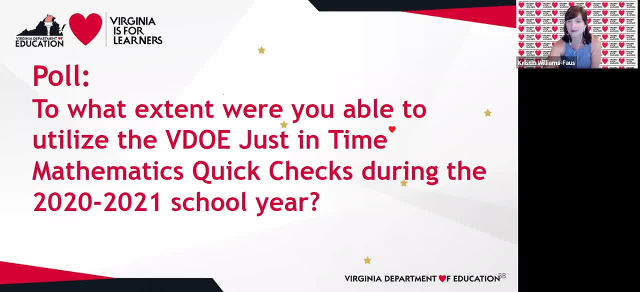 Okay, I think we're in pretty good shape, All right, So we'll go ahead and stop there. All right. So it looks like 35% of you have used it as a pre-assessment to assess prerequisite skills. 47% have used it as a formative assessment to assess current skills used during planning for. 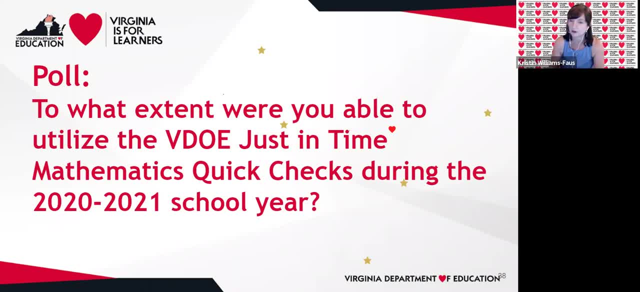 instruction. And then, I'm sorry, 42% have used during planning for instruction and about 32% of you have have not had a chance to use this resource yet, And some of those might be some of our administrators who are on the webinar today as well. 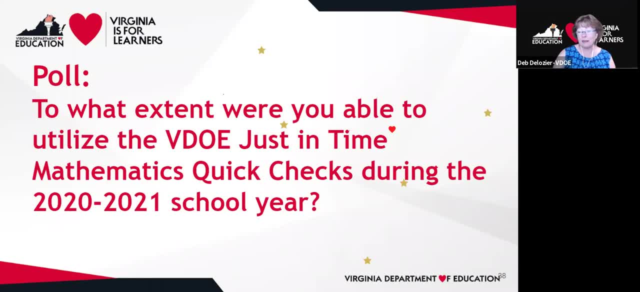 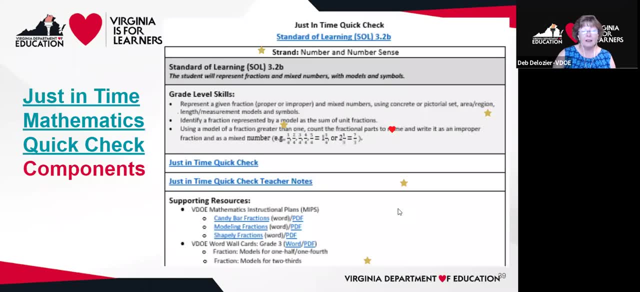 But it does help us to know, just like a pre-assessment you might give in your own classrooms. All right, So we want to take an opportunity to just look at a quick check And I think, Kristin, are you going to put that one in the link in the chat box. Excuse me, 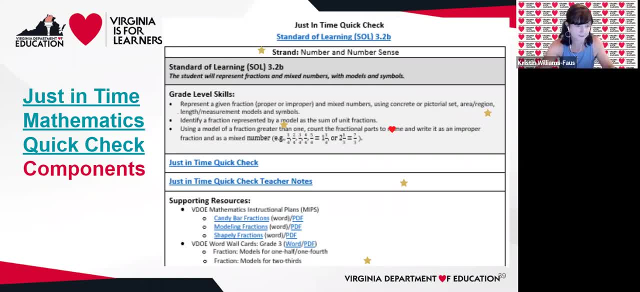 Yes, Sorry, I need a drink of water. I'm going to put a link in the chat for this particular quick check, which is the one we've been talking about: 3.2b, Thank you. So I am going to get out for just a moment. 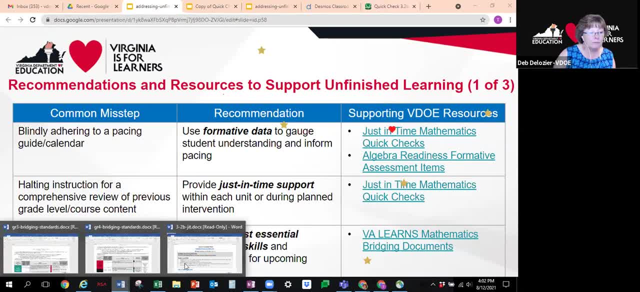 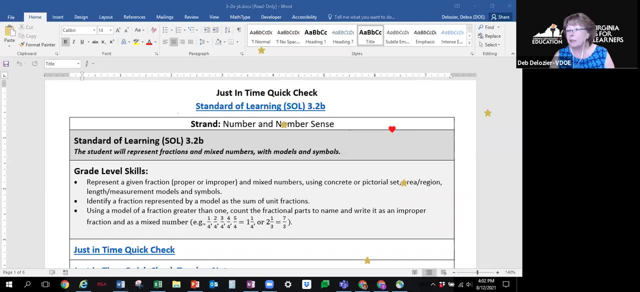 And pull that up on my screen, And you likely will have pulled it up on your screen as well. Although you don't have to, you could follow along with me if you would like. So just a quick refresher for those who may be newer to using the Quick Checks. 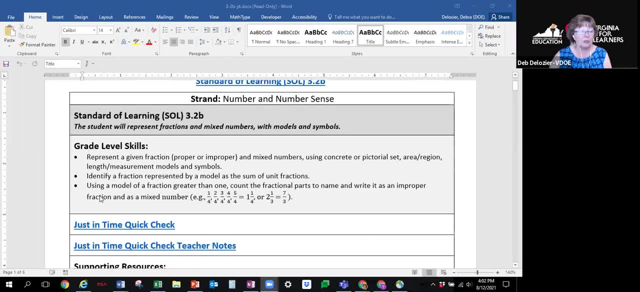 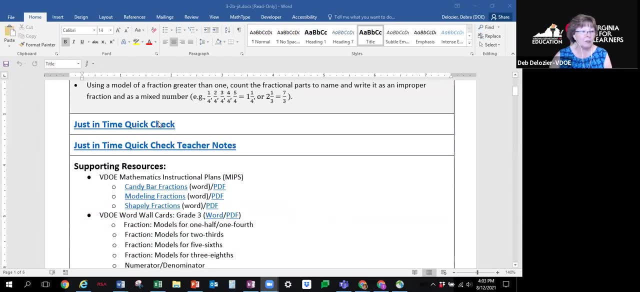 I wanted to just share about the components. Of course, you see, under grade level skills you notice that there's a little bit of a difference between the components. Those are the EKS bullets And if I click on the Quick Check tab it takes me directly to the questions. 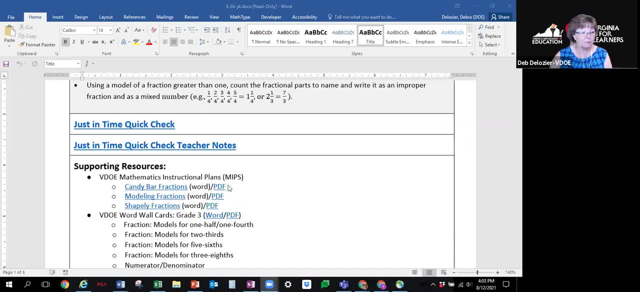 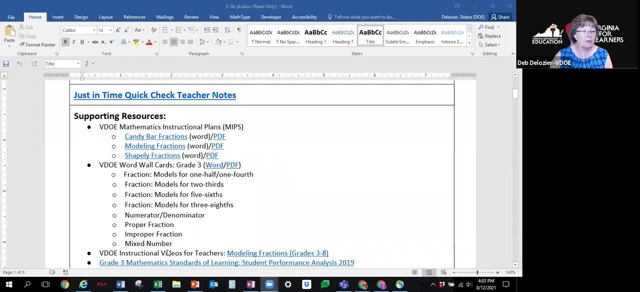 If I click on the teacher notes tab it takes me directly to teacher notes. But the nice thing about page one of the Quick Checks is that you see the supporting resources. So the teachers who helped us to develop these really looked at the mathematics instructional plans and identified which ones correlated most closely with this standard. 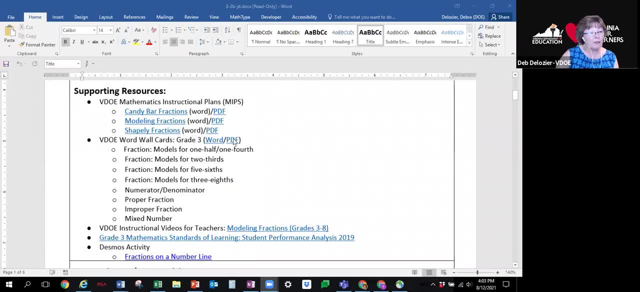 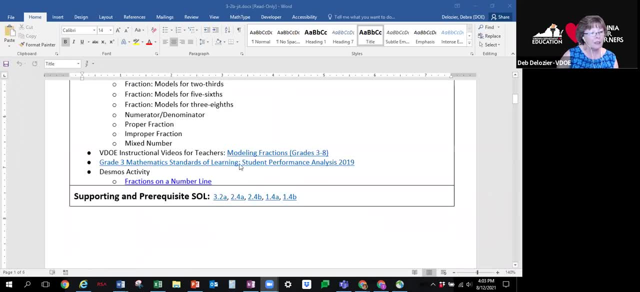 And they also looked at the word wall cards And they provided the links here for you, but they also put the cards that they felt applied most directly to this particular content. If there were instructional videos, those were included along with the links. In addition, if there were student performance analysis PowerPoints still available, then they put those links. 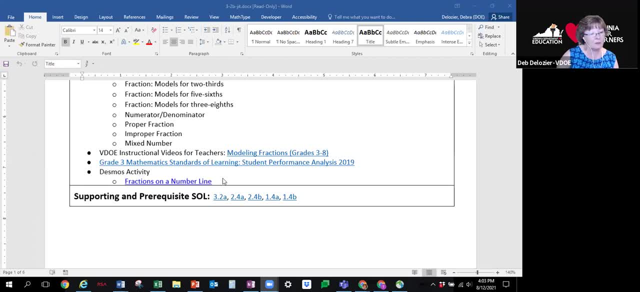 And, as you'll notice, here they put any Desmos activities that were on our Desmos Activity log, which we're going to share with you in just a moment. there And, last but not least, at the bottom of the page, it always gives you the supporting and prerequisite standards. 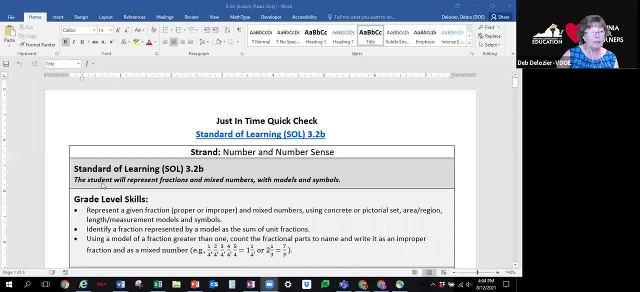 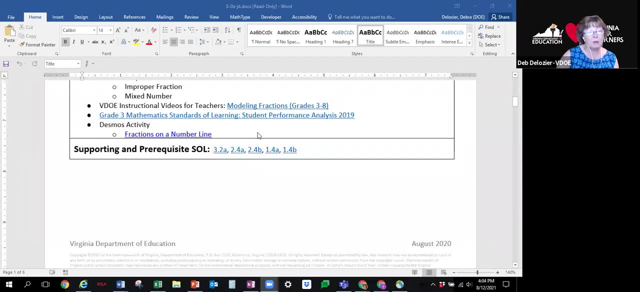 So remember this is standard 3.2 B, that is representing fractions and mixed numbers with models and symbols. So at the bottom these are the supporting standards And you'll notice that they go all the way back to first grade. So if I have some students that I might want to go back even further than the third grade. 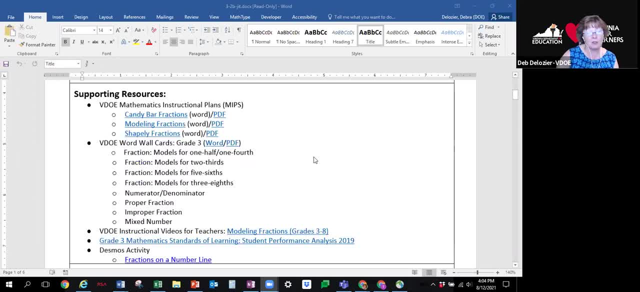 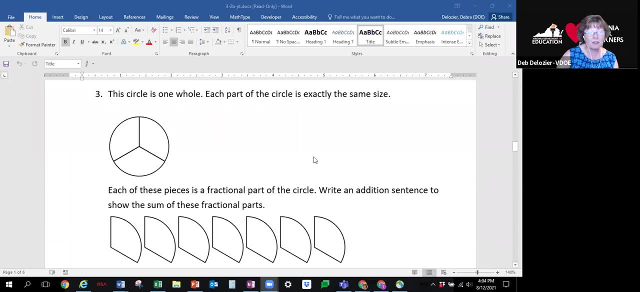 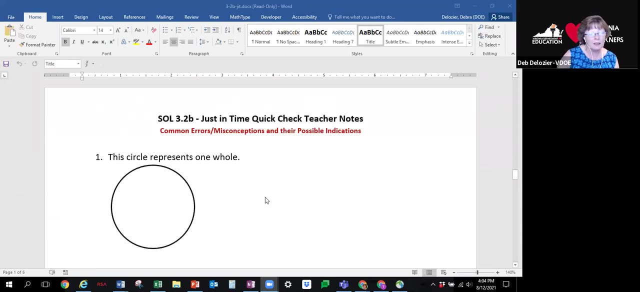 standard. I can utilize those as well, But then as I scroll on, you see the questions that we shared earlier and that you solved using the virtual quick check. So this is the print version And we'll put that link for all of the quick checks in the chat box as well. 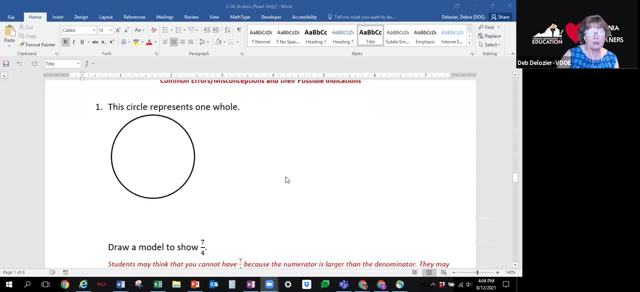 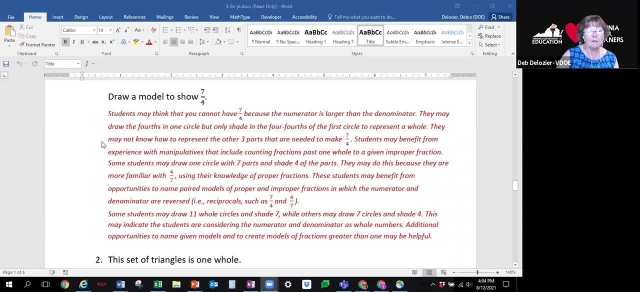 But then the next section provides the teacher notes. So one of the things that the teachers who helped develop these did was to identify first What were those common misconceptions that students make around representing fractions. And then they created the question and they provided those misconceptions here for you. 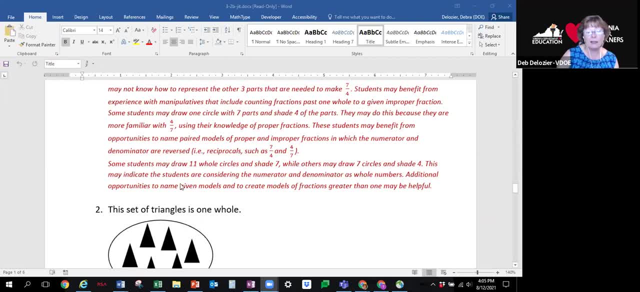 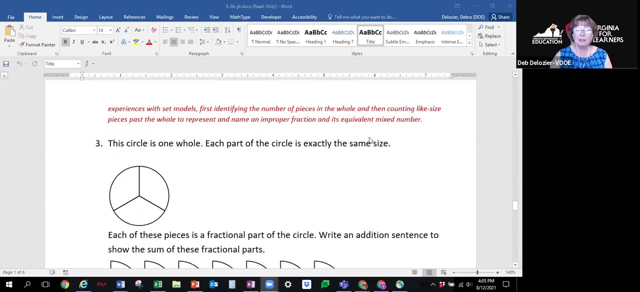 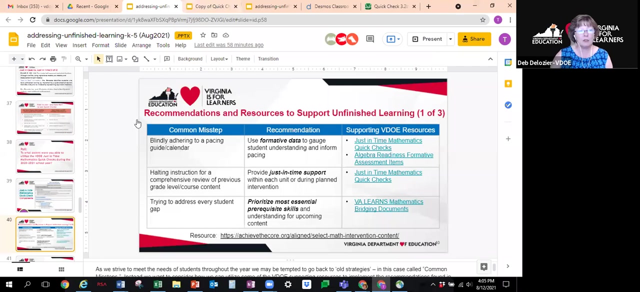 And they tried to give you examples of how you might help students. So here, and a suggestion is that additional opportunities to name given models and to create models of fractions greater than one may be helpful. So they are really great resources. They're really great resources in planning instruction and also in providing formative information on your students' current understanding. 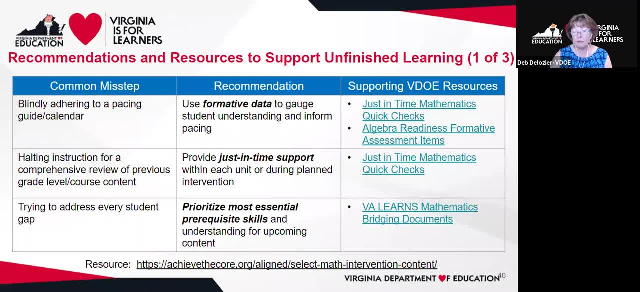 All right, I have a frog in my throat for some reason. All right, So bringing this section to a little bit of closure As we strive to meet the needs of students this year, which we know it's going to be a challenging year. 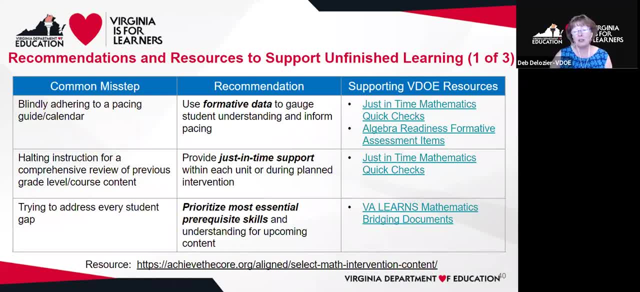 we have great educators in the state of Virginia. You all are going to do phenomenal work And our students are so eager to get back to school to see their friends, to see their teachers. But sometimes, when we're thinking about how are we going to fill what sometimes appears to be gaps in student learning- remember, these aren't gaps. 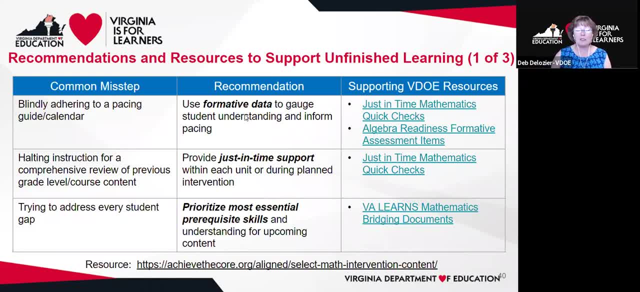 It's just where our students are Like at any other time when we start a new year, we're always thinking about: I wonder what my students know about this. I wonder what my students know about this. I want my students to know about that. 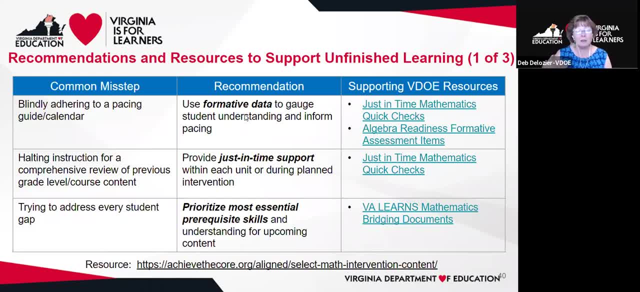 And sometimes we make what this resource Achieve. the Core calls common missteps. So sometimes we blindly adhere to a pacing guide or to a calendar, But the recommendation is really to use formative data to gauge student understanding so that it can inform our pacing right. 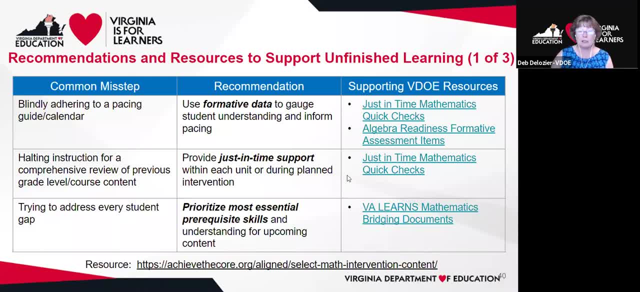 And then in the chart that we're going to be showing you on the next couple of pages, what we tried to do was take those missteps recommendations and provide you with links to any DOE resources that we feel would benefit in that area or that would go along with that particular recommendation. 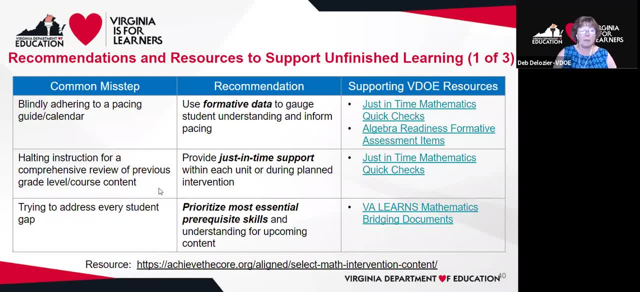 So another misstep that we often make is we stop instruction, Like we see a problem and we stop instruction and we do a comprehensive review of third grade. So I'm a fourth grade teacher and I see that students are struggling in fraction. I'm going to stop everything. 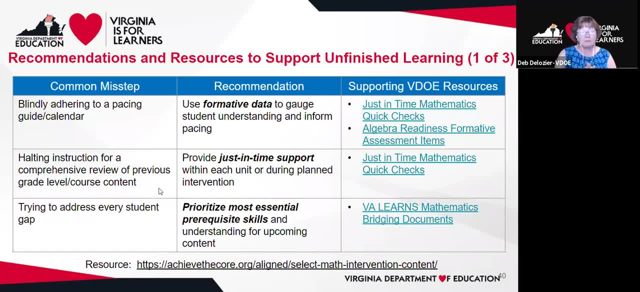 I'm going to go back and teach the third grade standards. Well, that's not. That's not the best thing to do. We really have to think about how can we provide that just-in-time support with each unit or during that planned intervention time. 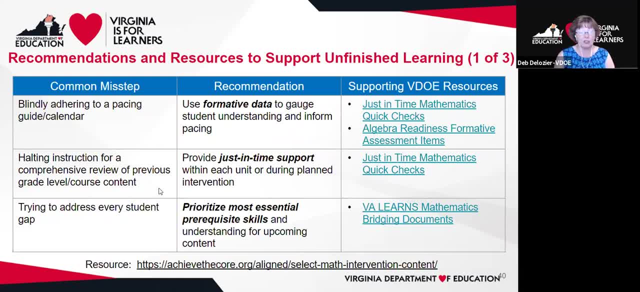 And something that will help you with that is those just-in-time quick checks And trying to address every student gap. there's just not going to be time to do that, But we can prioritize those most essential prerequisite skills and understanding. that's going to help with the upcoming content. 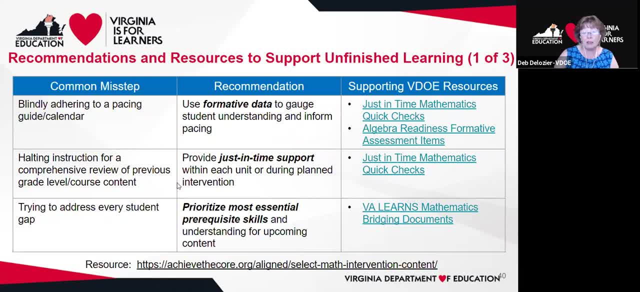 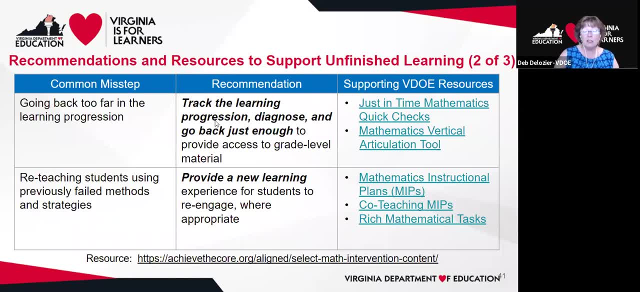 And so some of the resources found in the Virginia Learns math bridging documents will help you with that In terms of thinking about trying not to go back too far in the learning progression. you want to track that progression right Diagnose and find out where kids are exactly so that you can meet them right where they are. 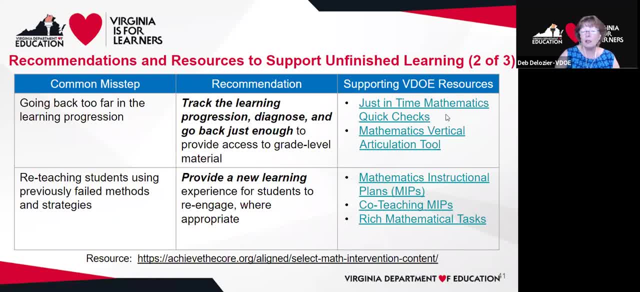 And some of the resources that help. there are going to be the quick checks, but also the MVAT tool. The MVAT tool will show you the progression from kindergarten all the way to Algebra 2.. So that will be a helpful tool as well. 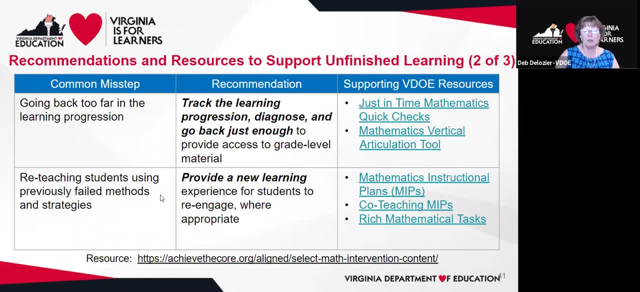 One of the things that we often do is we reteach students using those same strategies that weren't successful before. So we need to think about how do we provide a new experience, How do we engage kids in a different way that's still appropriate and still connected with the content. 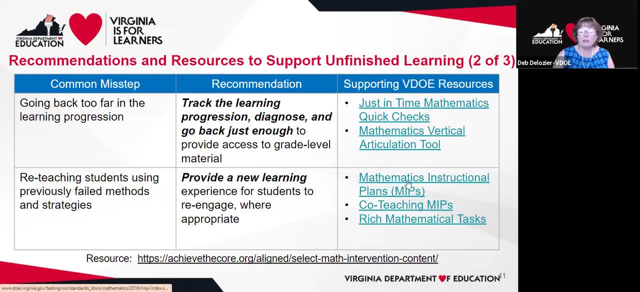 So here you can see, we've put a link to the instructional plans, the mathematics instructional plans, as well as the co-teaching math instructional plans and the rich mathematical task, And we hope you will join us. We'll be able to utilize those as you move forward this school year. 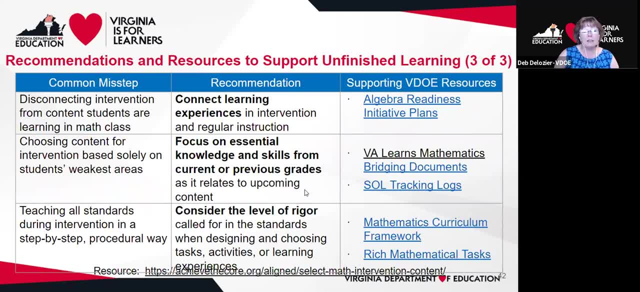 The next thing really to think about is not that we often make the problem. that we often do is disconnect an intervention from what's happening in class. So if kids are working on something different in their intervention than what is being focused on in class, that's not the best way to go about it. 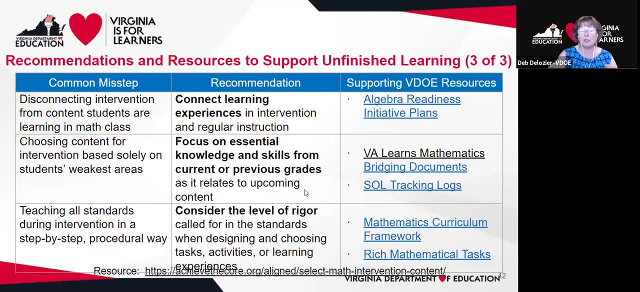 We really want to connect those learning experiences to the intervention so they complement one another right, And so the algebra readiness, The algebra readiness initiative plans, can assist with that. Those plans, however, are more grade 4 and up, but they can help you with that, as well as the other resources that we've been sharing today. 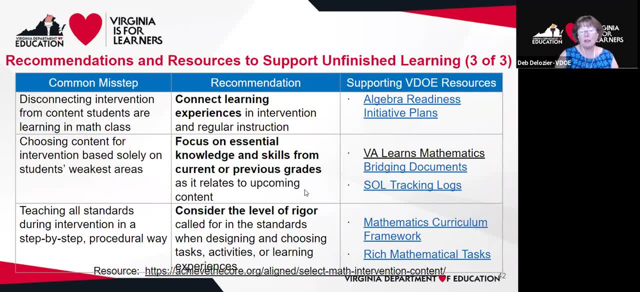 But being sure that we focus on essential knowledge and skills from the current or previous grades as it relates to the upcoming content, rather than just choosing content based on students' weaknesses but really thinking about how those students' weaknesses connect with the essential skills and knowledge that they need for the upcoming unit or for what we're working on right now. 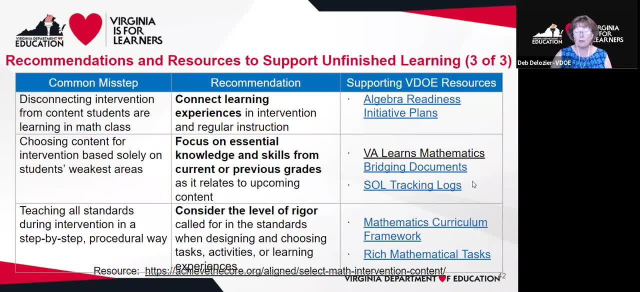 And so the tracking logs will help. if the prior grade level has shared those with you, That can be very helpful in your planning if you know that students didn't have enough exposure or the previous grade teacher didn't feel the students were as successful as they could have been in certain areas. 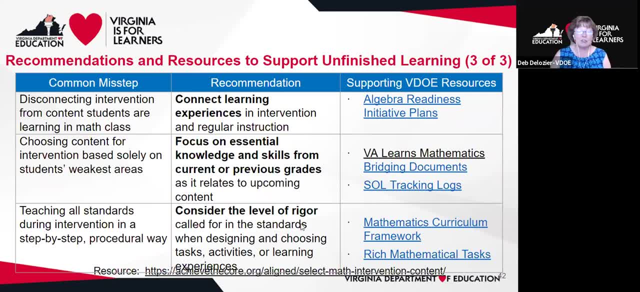 So tracking logs or something similar that provides you some of that information will be helpful. Thank you. The last misstep on the chart here is teaching all the standards during intervention in a step-by-step, very procedural way. We have to keep in mind the level of rigor of the standards right when we're designing the activities and tasks that we're providing to students. 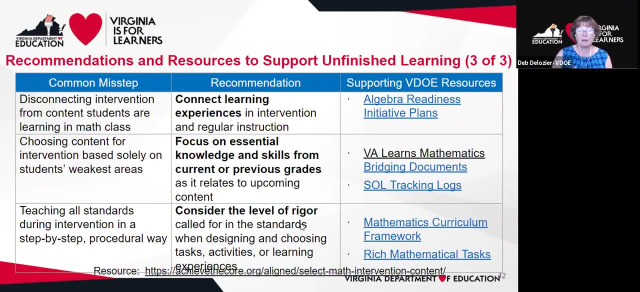 So we want to make sure that they align versus providing step-by-step strategies and not meeting the level of rigor. So you'll definitely want to refer to the frameworks as well as utilizing rich math tasks moving forward. So hopefully some of those strategies will work or some of the resources will be helpful to you. 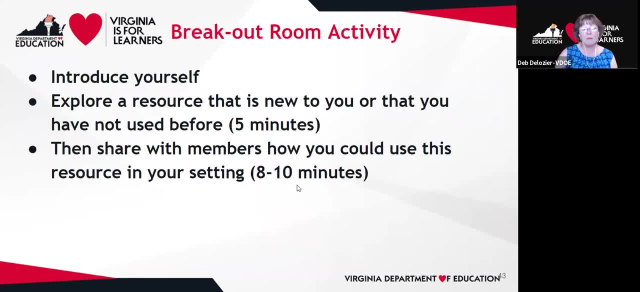 So we wanted to spend a few minutes doing sort of two things. I've kind of modified this a little bit. We're going to do a breakout room activity and we want you- Kristen's- going to put in the chat the link to the PowerPoint. 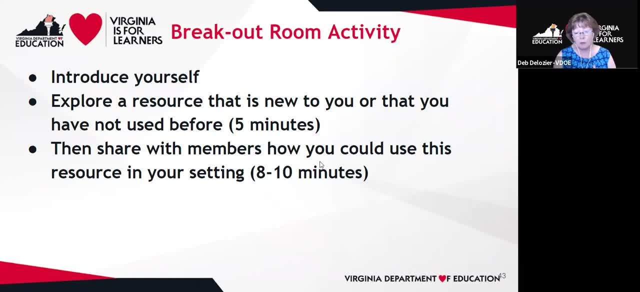 So we want you to go to slides like 40,, 41, and 42.. That's the PowerPoint. Okay, That's where the slides. I just went through And look at some of those resources. Choose a resource that's either new to you or you haven't had a chance to explore. 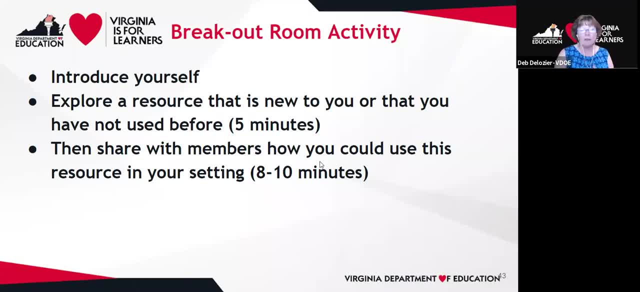 Maybe you knew about it, but you haven't had a chance to check it out. So we'd like you to choose one of those resources When you get into breakout rooms. you're going to introduce yourself, You're going to explore the resource. 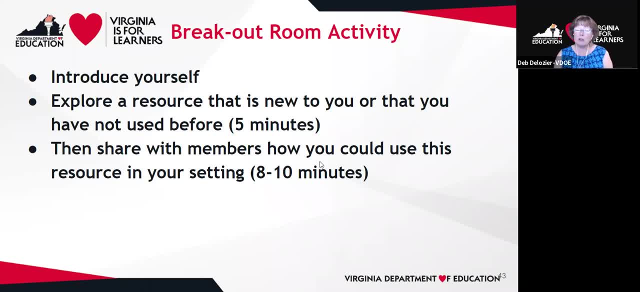 And then you're going to share with members how you think you might be able to utilize that in your setting. But also, when I said I'm going to modify it, I'm still keeping in mind Sharon early in the session, Who talked about how to help teachers. 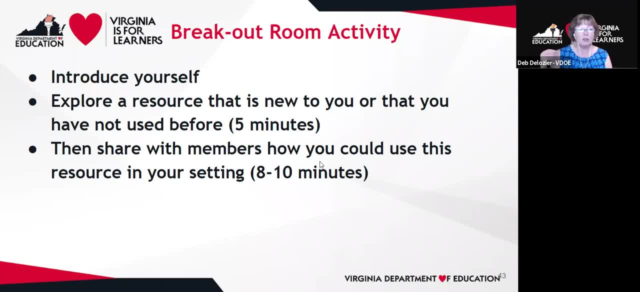 She's supporting teachers, So how might she help teachers utilize some of these materials in meeting the needs of students in the coming year? So, Kristen, are we about ready? You're on mute So we're not hearing you right now, Sorry. 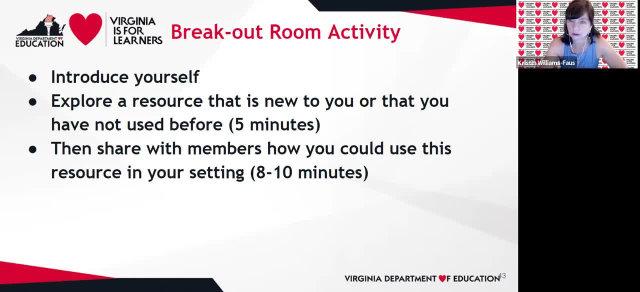 Kristen's going to open up our breakout. Yeah, I'm thinking we're going to do 40.. 40 rooms: Yeah, So it'll be about four participants per room, All right? All right, Here we go. Perfect, We'll bring you back in about 10 or 15 minutes. 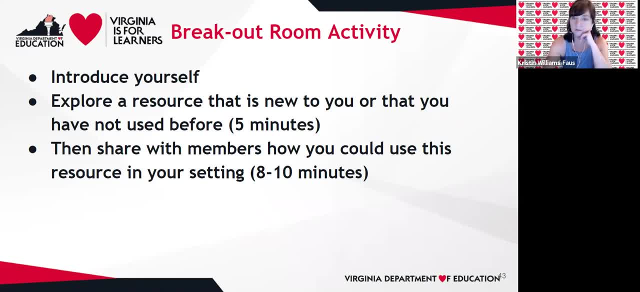 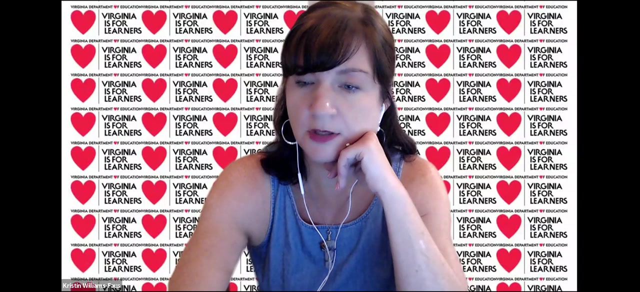 We'll check out how you're doing, But you should be getting an invite And if you would join the breakout room that we're sending to you. If you're still in the main room and you're having any trouble getting to your room, let us know and we can try to help. 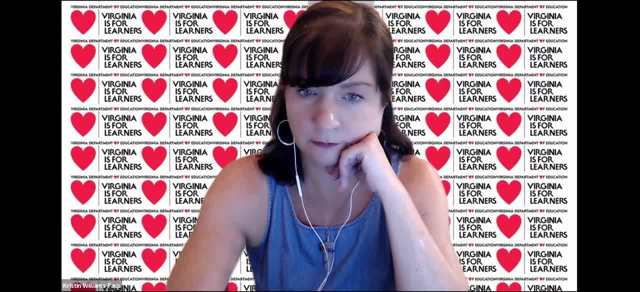 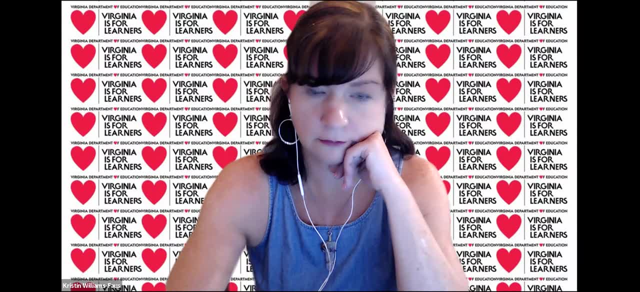 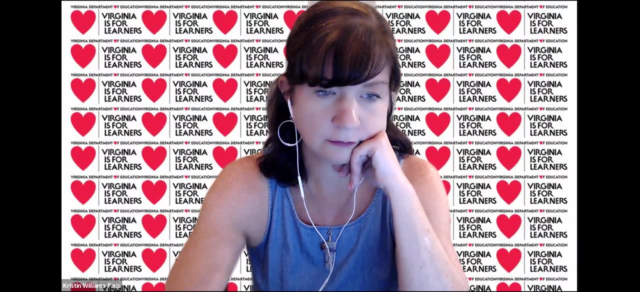 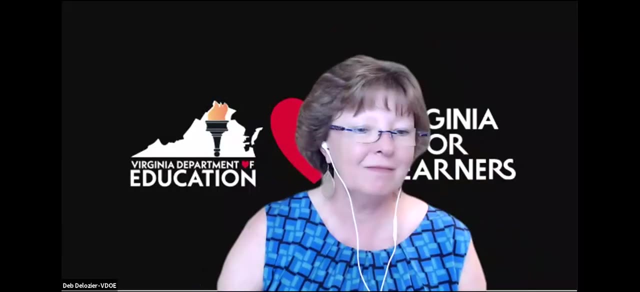 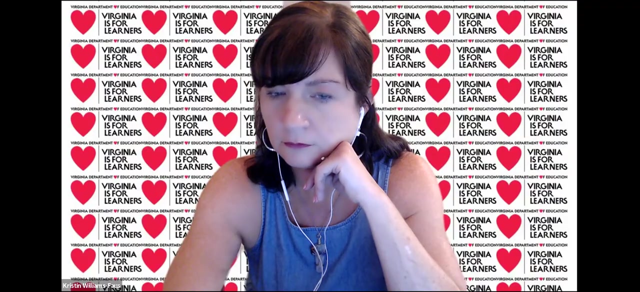 All right, All right, All right. Okay, Sharon or Betty, can we help you at all? Did you find your rooms? They may have stepped away. Mm-hmm, I think I've been talking too much because my throat is dry. 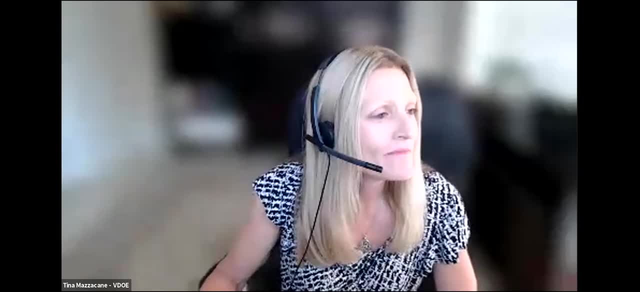 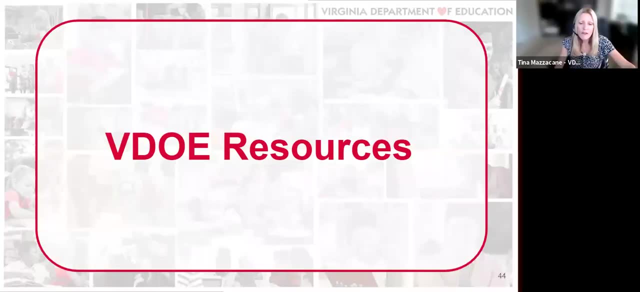 take us to the last stretch. all right, everybody. well, we hope that you enjoyed having a little bit of time to network with some of your colleagues. um, it's always nice to be able to talk to someone outside your school division. sometimes it's on the whole other side of the state, which is really- it's really great, um, so 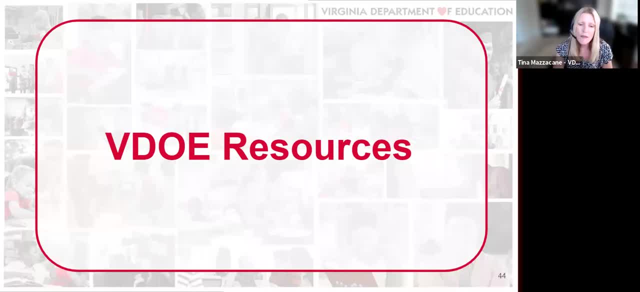 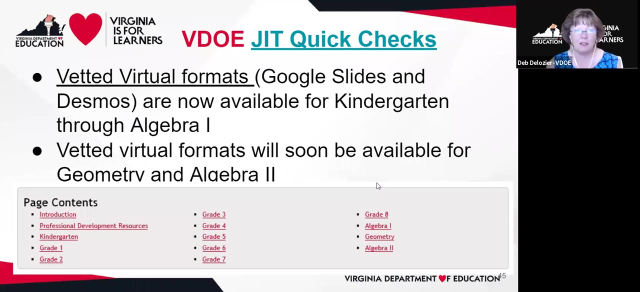 we wanted to just share some additional resources that you may um or may not be familiar with. so on the next slide we have some information about a resource that can you click to the next slide. deb, sorry, i was in the chat, you're fine. so not only do we have the just-in-time quick. 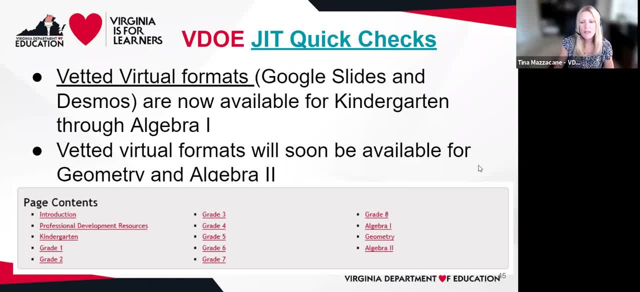 checks, as we mentioned, that are available on our web website in word and pdf format, but we also have the virtual format, some that we kind of previewed for you today. those are available in an excel spreadsheet and currently they're available for kindergarten through algebra one, and so you can. 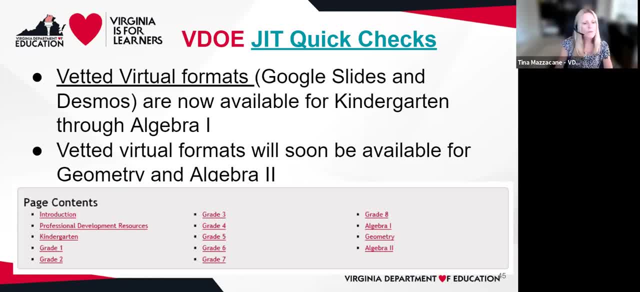 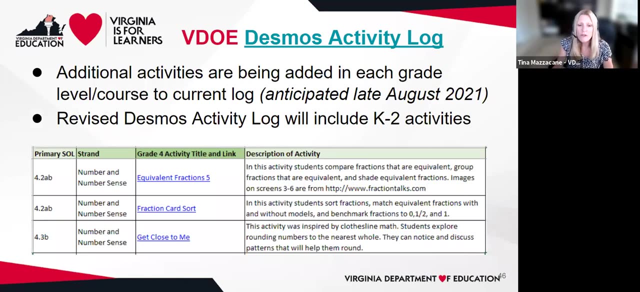 take a look at those and kind of see what what might help you in your instruction as you plan for the upcoming school year. and on the next slide it looks like we've got information about our desmos activity log and this is also an excel spreadsheet with with several links that are organized by grade level. 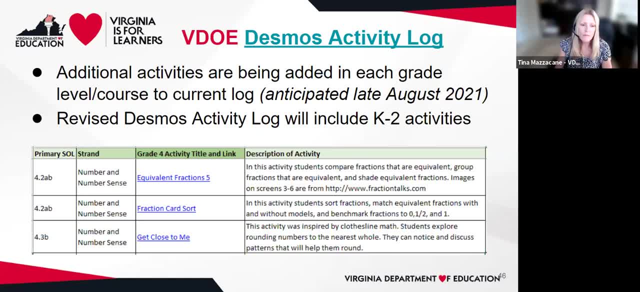 and they are activities that align to the standards of learning that are available in desmos. so these are in addition to the virtual quick checks. these are actual activities that you can use with your students. we did have a committee that worked and revised this log, so we'll be posting that later. 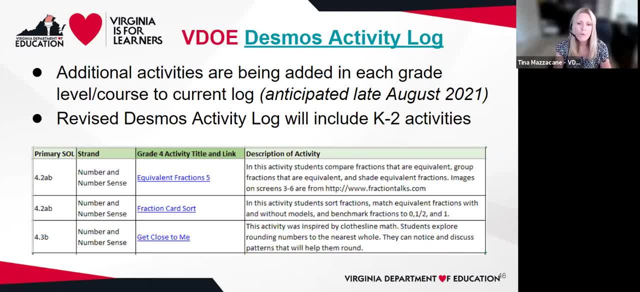 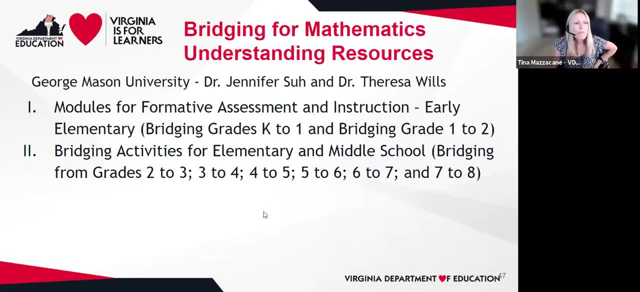 this month, after we've been able to vet all of those links to make sure that they're working appropriately, so you'll have an updated version of that. we also wanted to mention that we've been working since this past spring with george mason university, with two of the professors there, and we're very excited about the work that they're doing and 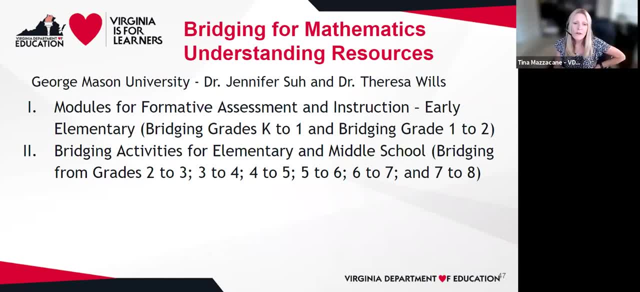 creating bridging activities. they're working in grades k all the way up through eighth grade, looking at how we can bridge from one grade level to the next and creating modules that include different resources and things that might help you in in planning your activities and your instruction to help bridge from that one grade level to the next. so on the next slide, it shows: 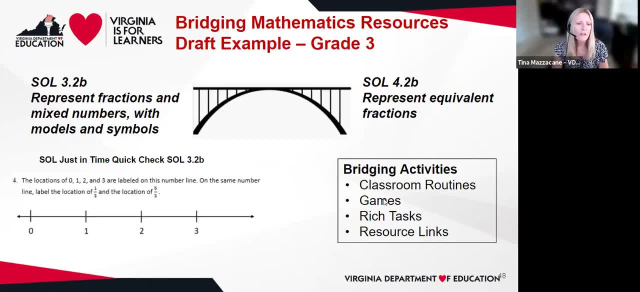 a little bit of information about what a bridging activity might look like. so they typically include a just-in-time quick check that you can click on and use with your students. and then, for example, this one is is again that example we've been using from third grade into fourth grade about 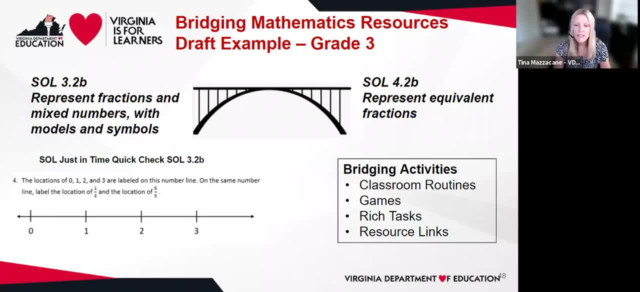 equivalent fractions. it might include some classroom routines or games, or a link to a rich task, or even some other resource links that might help you in planning instructions. so again, another bank of resources that might be helpful to you. we are going to be previewing this particular. 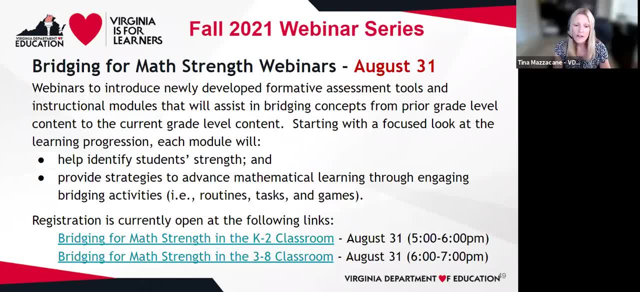 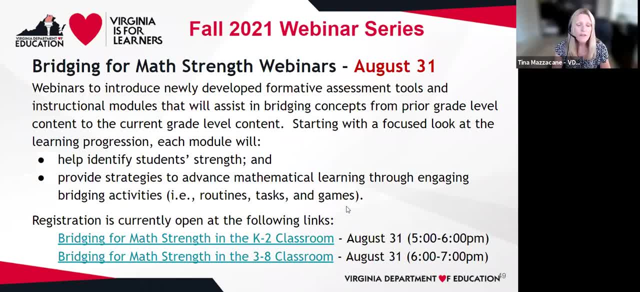 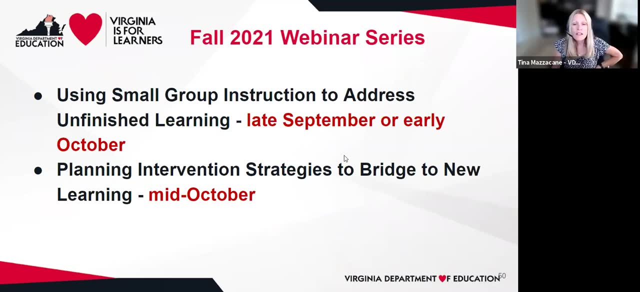 webinars that will be happening later on this month And those resources will be rolled out at that time so you can kind of look and see how they work and what's available. We also mentioned at the beginning of the session that this is a first in a series of webinars that 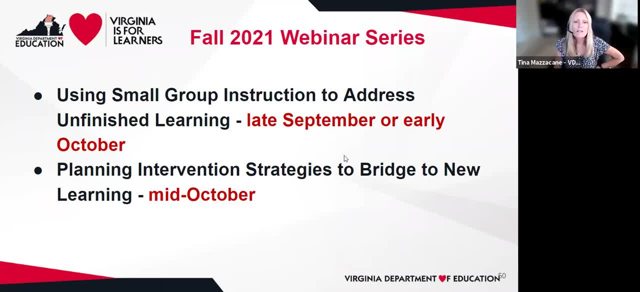 the Virginia Department of Education is offering. So late September or early October we'll be looking at using small group instruction to address unfinished learning and then in mid-October we plan on looking at planning intervention strategies to bridge to new learning. So be on the lookout for registration links for those particular opportunities. 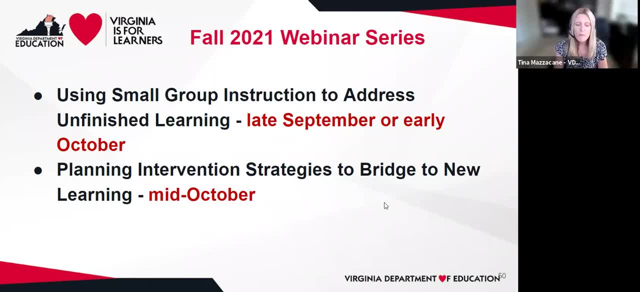 Oftentimes we put those on our TeacherDirect website and those are also emails that go out every Wednesday. If you haven't registered for TeacherDirect, you can go to the BDOE website and there is a link for you to go there. 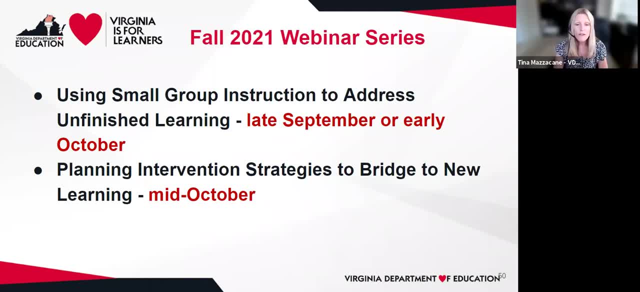 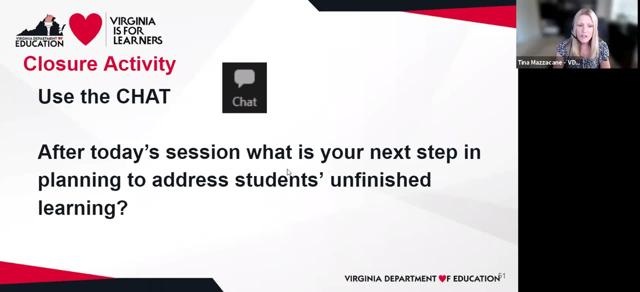 to put in your email and they'll send you an email every Wednesday about different offerings, not only in mathematics but other disciplines and information. So as we close up today we've talked a lot about addressing unfinished learning, So just kind of want to get your closing thoughts about what might be your next step in planning, or maybe. 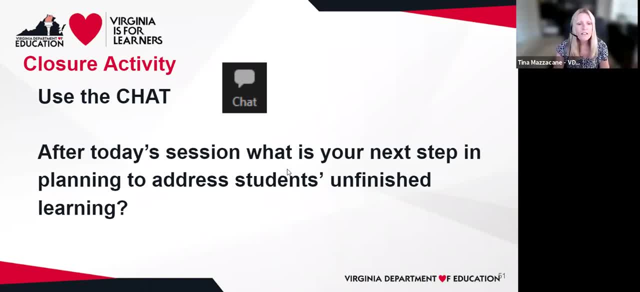 some ideas that you got from today's session to help you in planning for that unfinished learning. We can also certainly stay on afterwards to answer any questions that you may have, So feel free to hang around and open up your mic. We're happy to answer questions. We're very pleased that. 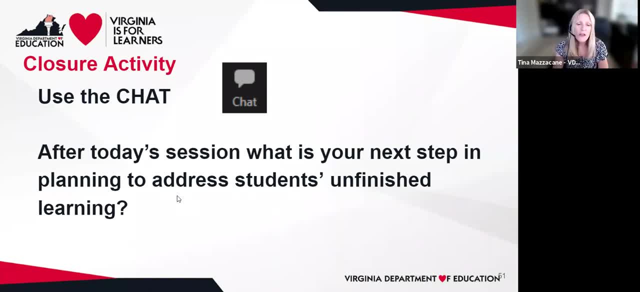 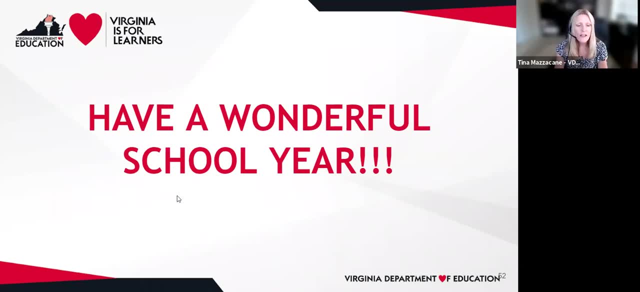 you're able to join us this afternoon for this session. We wish you the best of luck as you open school- if you haven't already- and have a wonderful school year. So please feel free to stay on and ask questions, or you can put your questions in the chat, along with your ideas about.